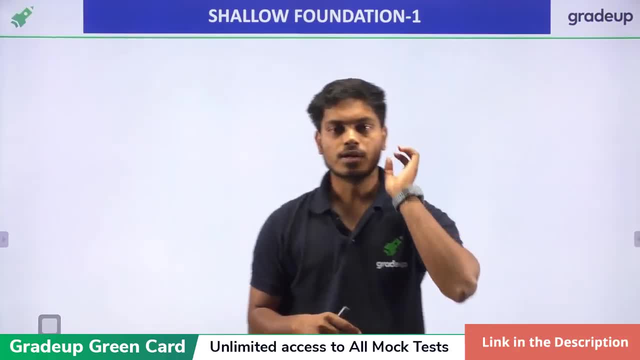 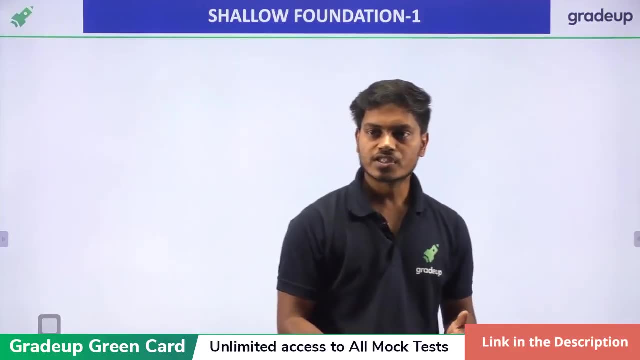 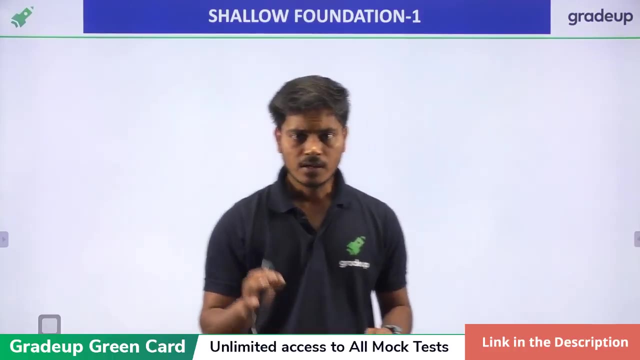 possible so that you people have time to revise them. and as soon as this subject will completed will be completed, we are going to have a doubt session. in the doubt session, we'll solve some questions also and we'll take the doubts here and itself. okay, then, and there, no, nothing will left. 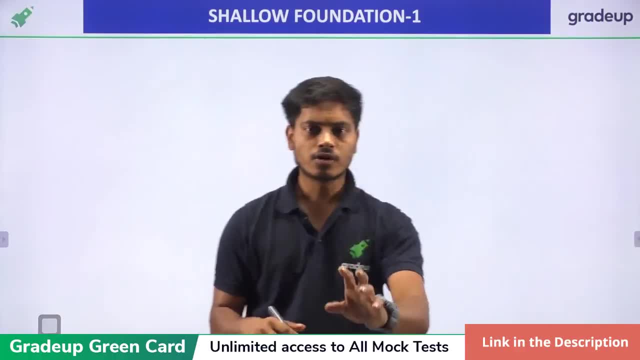 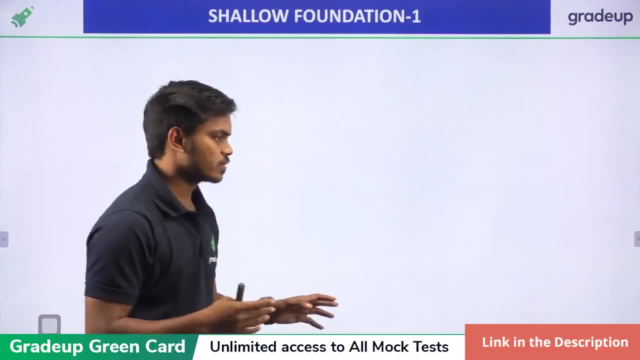 for like further time. we'll just you. you have any doubt? you ask me, i'll answer you. okay, you won't take any doubt along with you in that session. so that's the reason why i'm not taking more number of questions and i'm focusing on the theory only right now. okay, that, but also i try to give you. 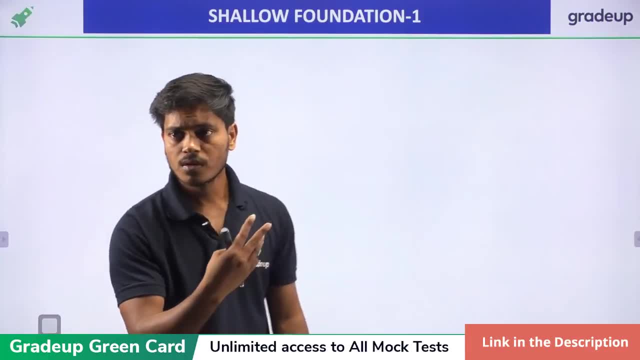 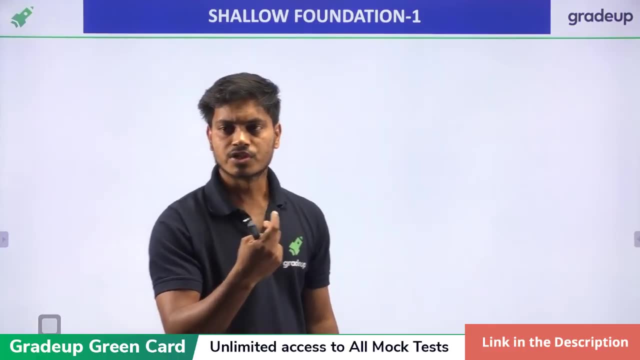 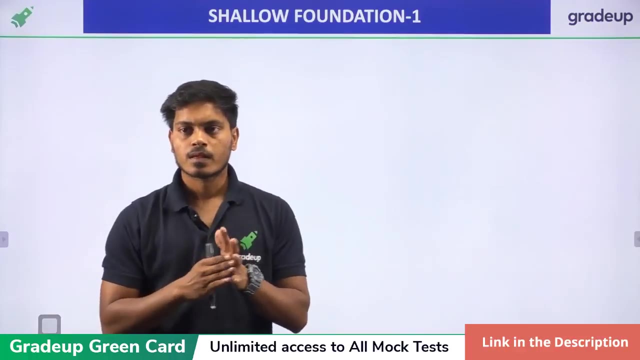 some questions like tomorrow. we have solved three questions. i am third year student. please tell me, uh, the subjects, tell me some tips, sir, i'll explain in irrigation, okay. okay, uh, preparation thing. suresh, uh, you are in 30 here. all right, I have something for you. just please let me know in the end of 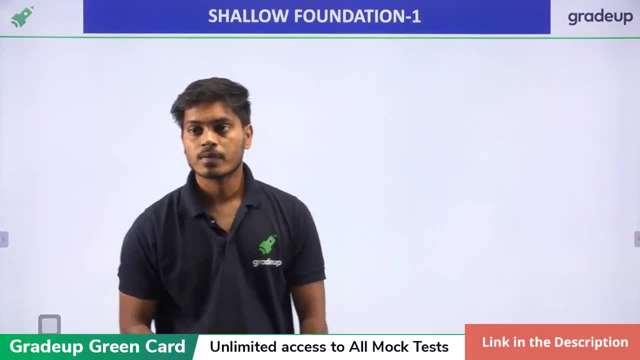 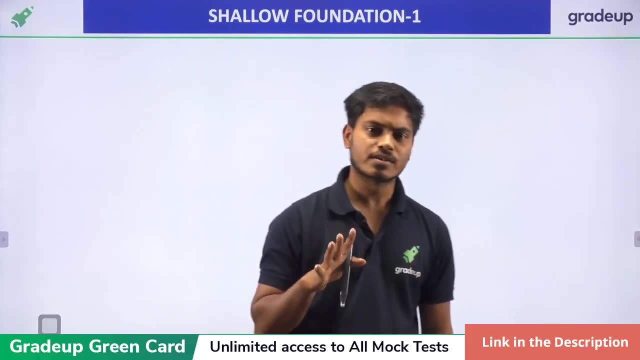 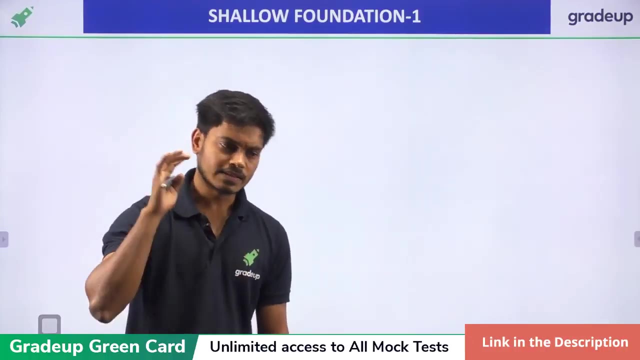 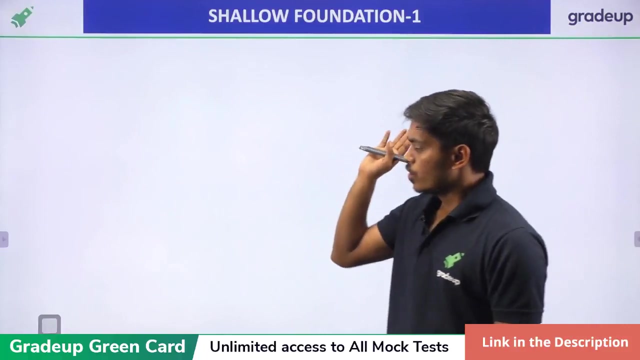 the session. we are going to have a good discussion. okay, so, as informatics, is the concepts enough for? okay, this- this question is from so much, so many students that is this enough for the gate? see, the whole concept behind these class is it is a quick revision classes. okay, it is a quick revision classes, so. 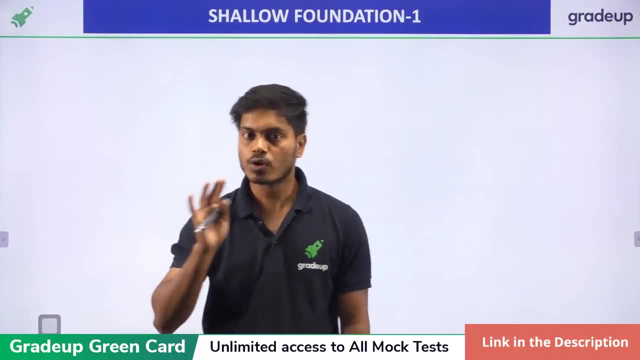 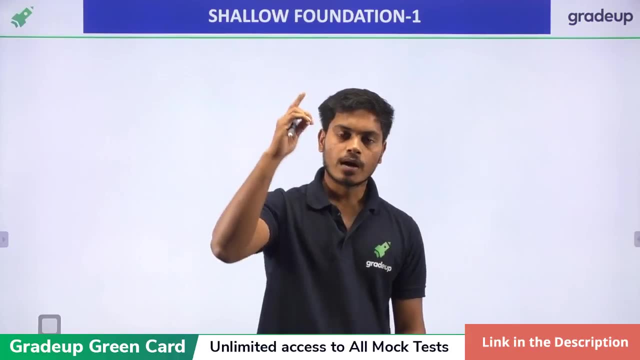 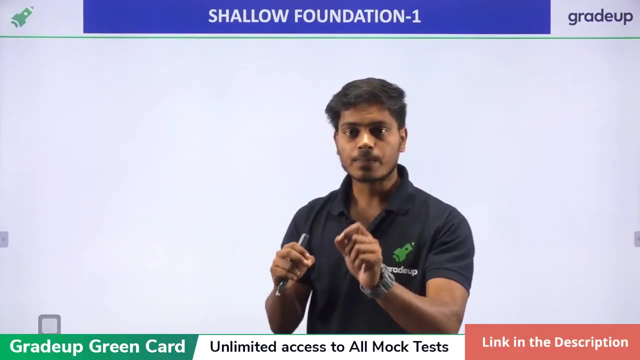 you have to study the subject thoroughly by yourself, at least once or twice, according to the potential you have. okay, at least once and once or twice, and solve each one, each- and I'm just see, I'm emphasizing the word each- each previous year question. then only you will get to know what is the pattern or what is the. 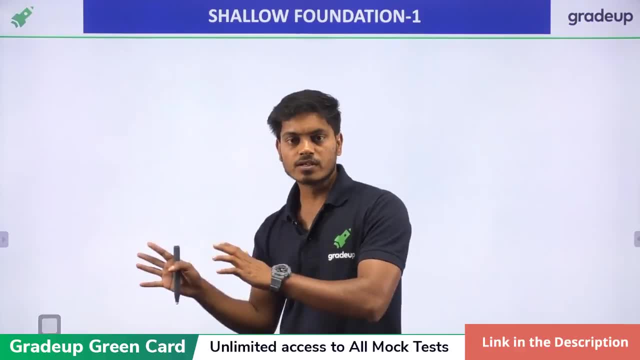 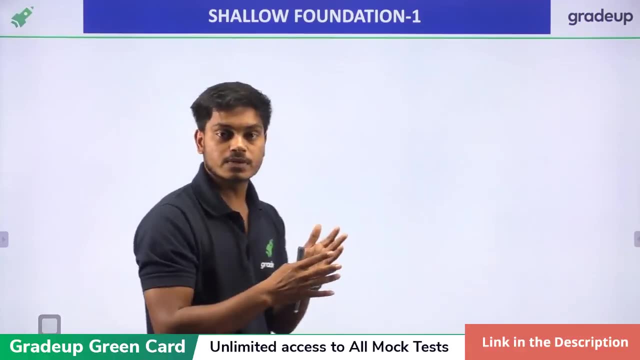 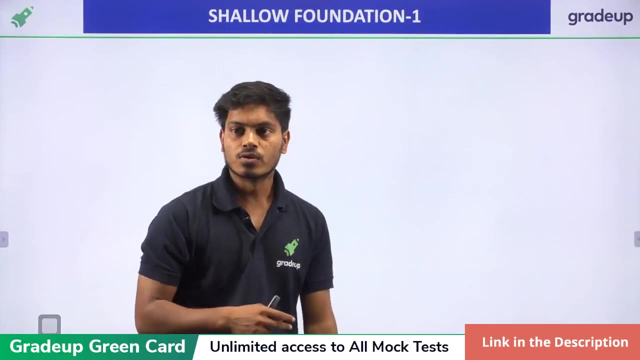 important things that are going to be there in your examination. okay, so that's the thing here. all right, we are focusing here on the major concepts. okay, whichever are there, so these are the things that we are discussing here. yes, actually I know, Kumar, like this is the time when we have your, like you have your semester. 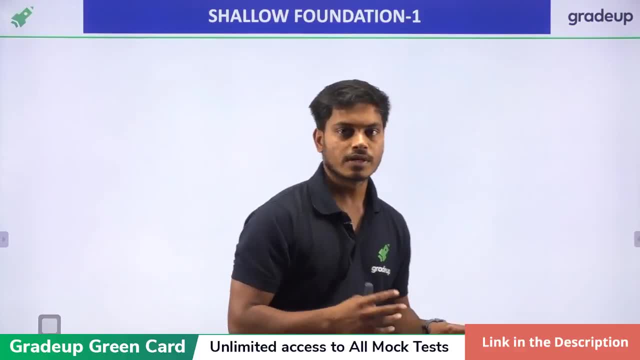 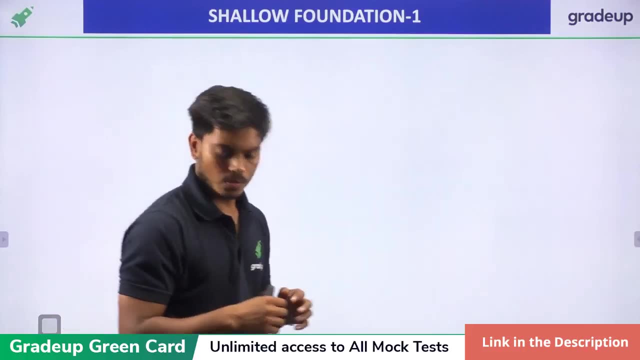 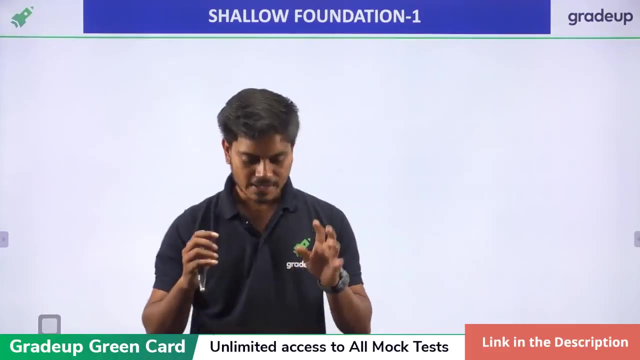 examinations okay, but it is like the best time when you can have a quick revision. hi Neha Abhi, hello. okay, so we were discussing about when to use which one, which type of foundation. so when the structural load is less and the type of soil is medium to dense, in that condition you have to use shallow. 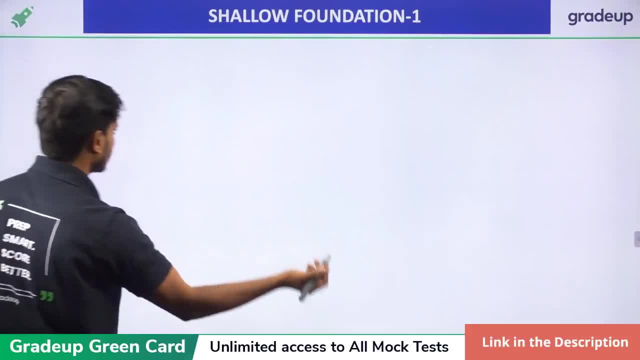 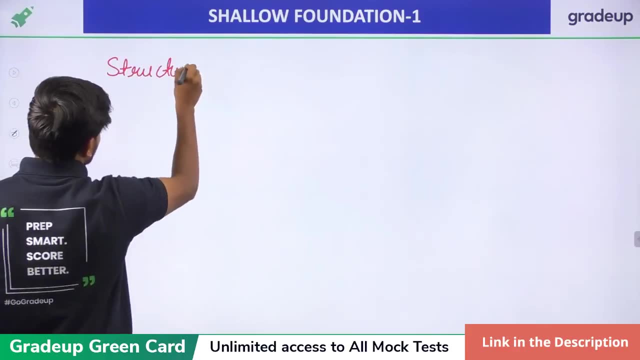 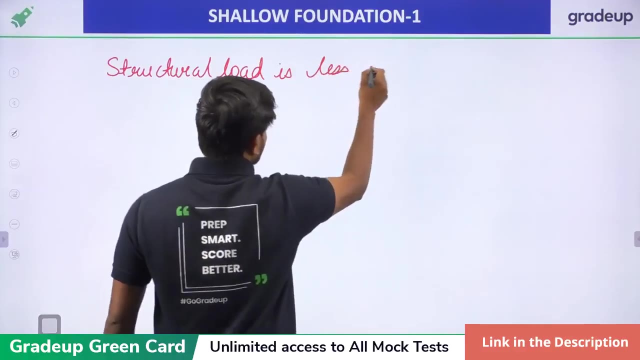 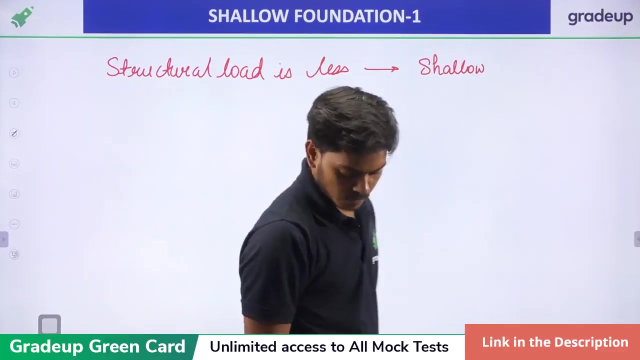 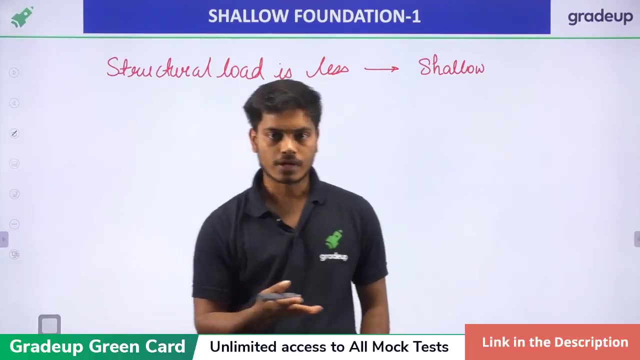 foundation. so I'll just write it here, if you want. you can note this, note this down also. so structural load is less, structural load is less, okay, soil is medium to dense, then you have to use shallow foundation, all right. and if there is a chance of differential settlement, okay, differential settlement. 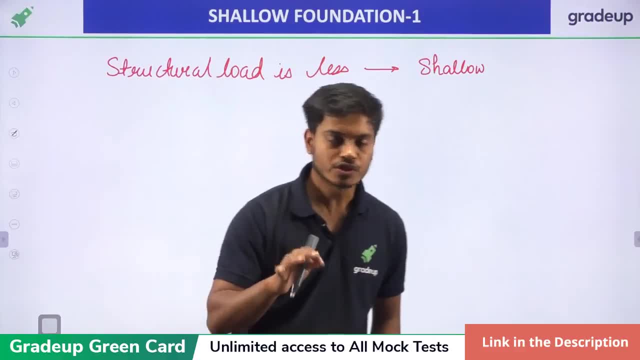 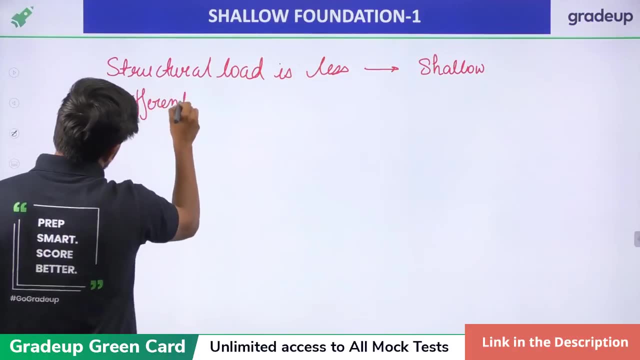 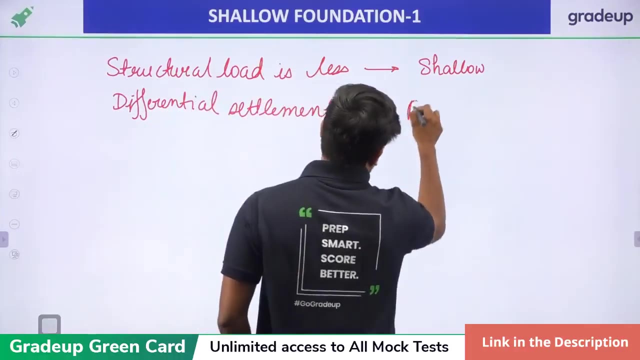 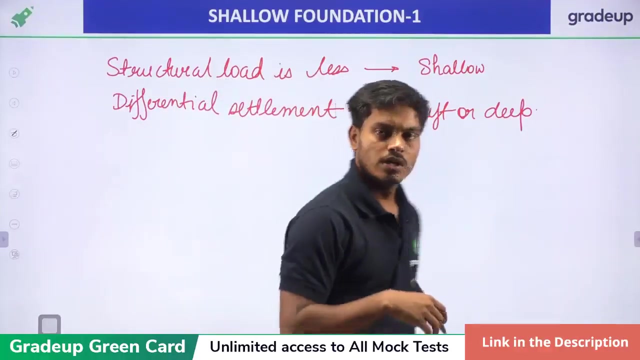 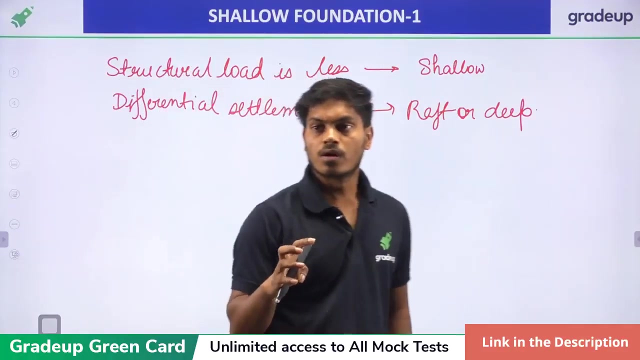 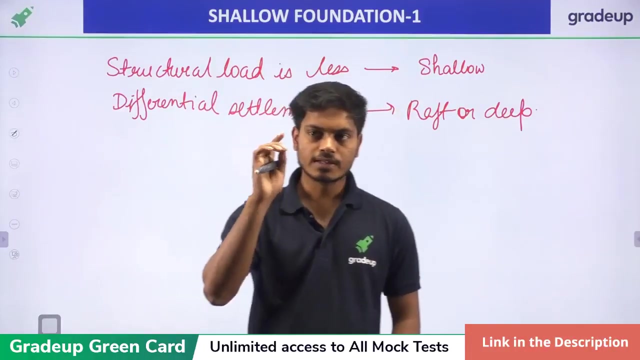 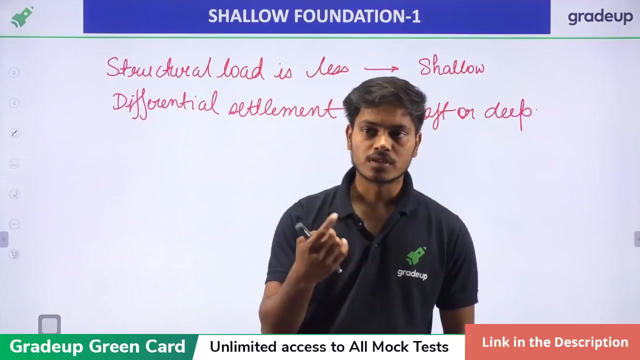 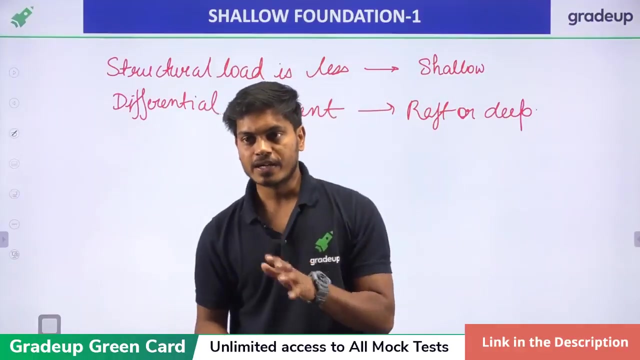 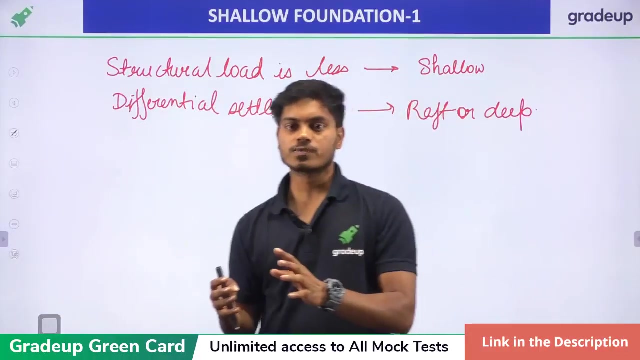 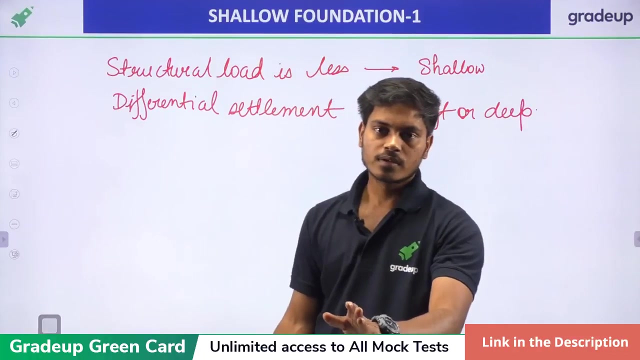 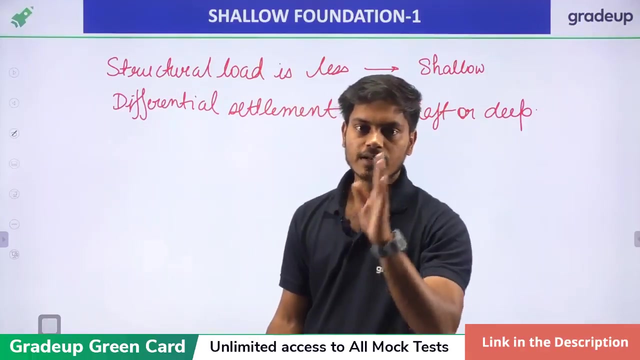 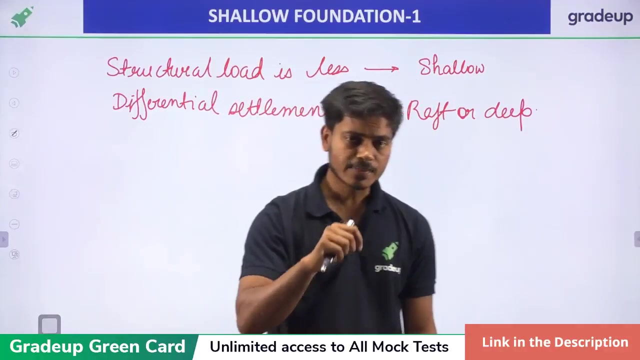 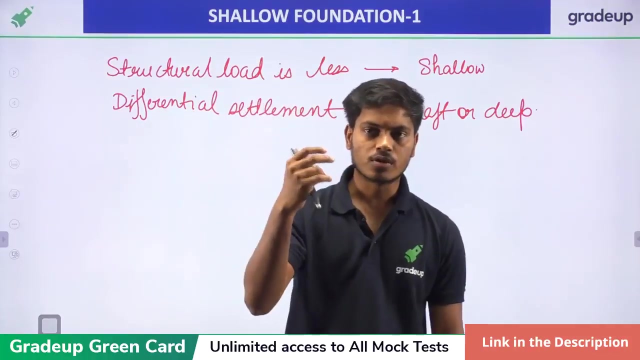 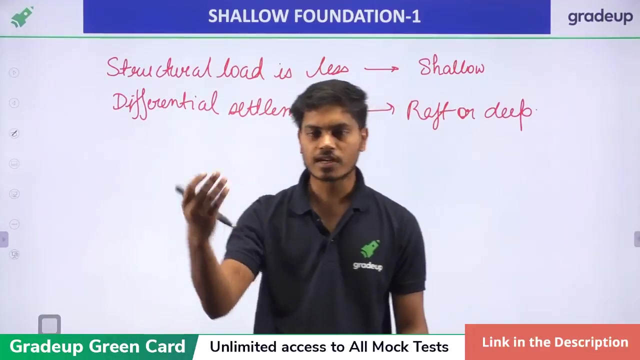 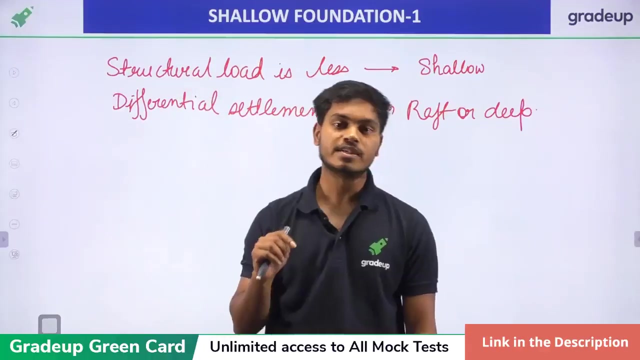 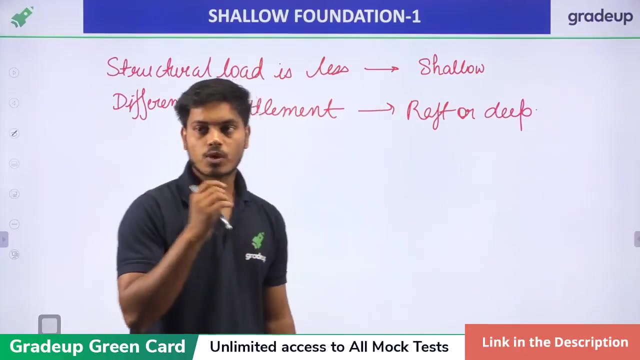 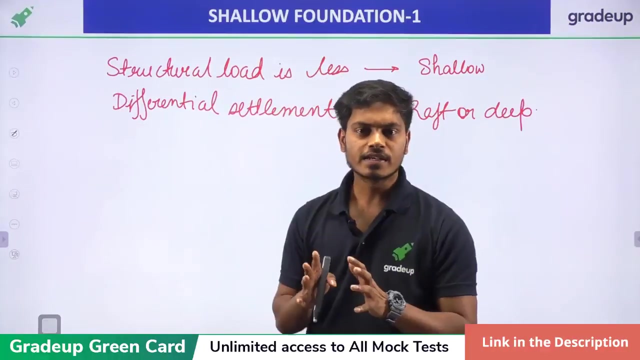 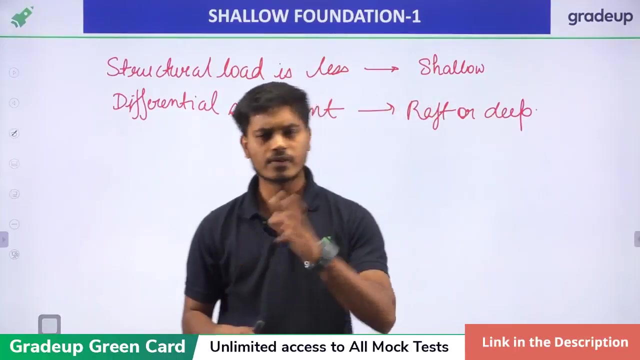 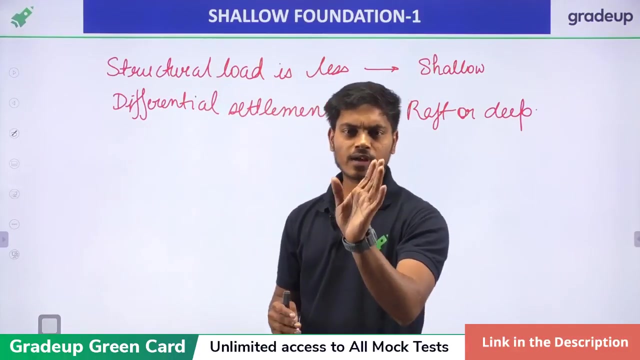 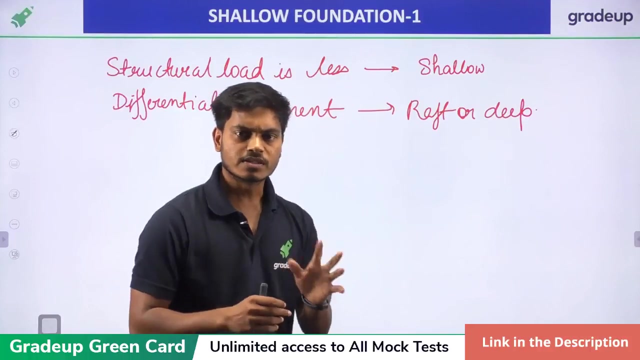 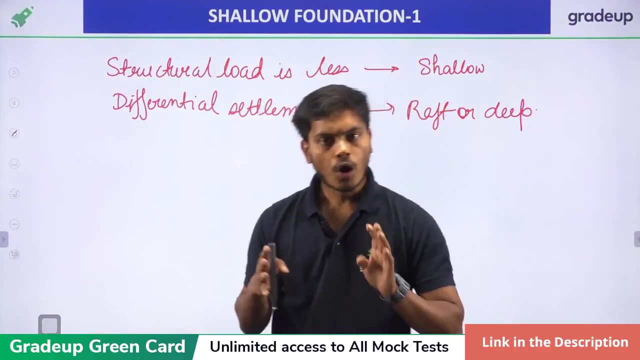 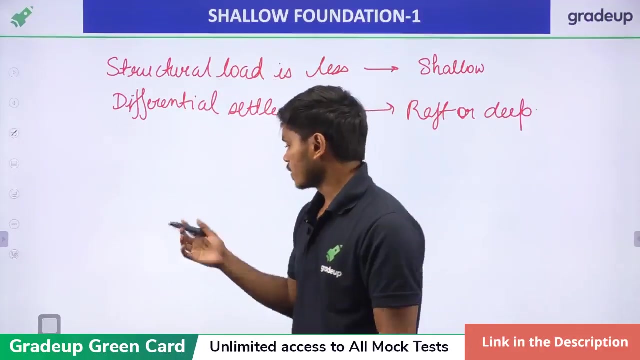 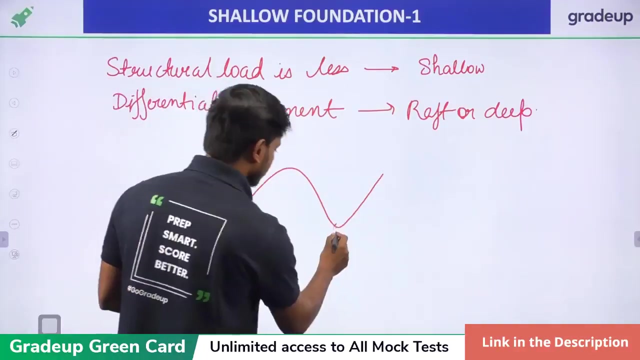 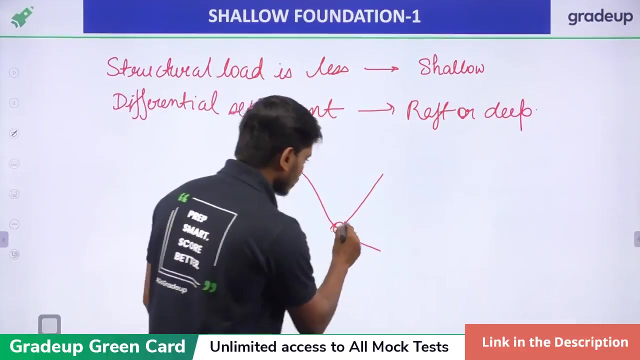 in that case you have to use the rough foundation or the deep foundation, so differential settlement you can. you notice that there is no such thing existed. you are going to go upside only so. you just have to focus and you don't have to take care, you don't. 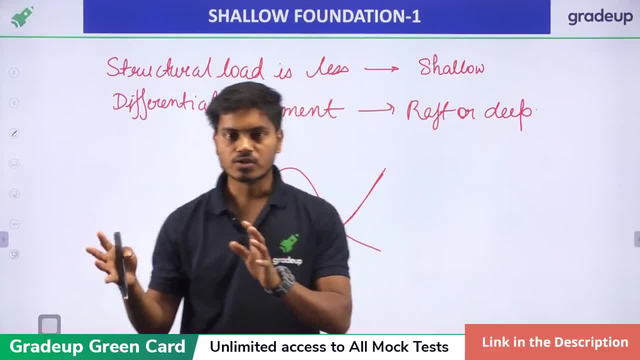 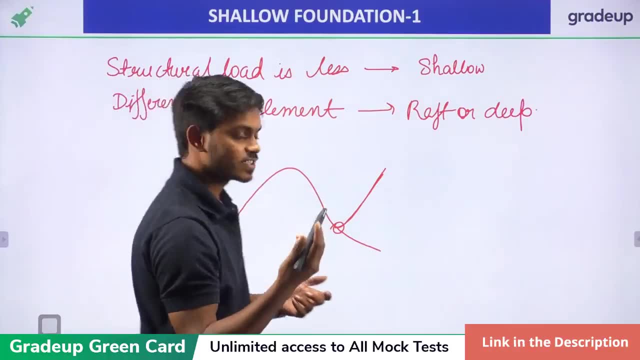 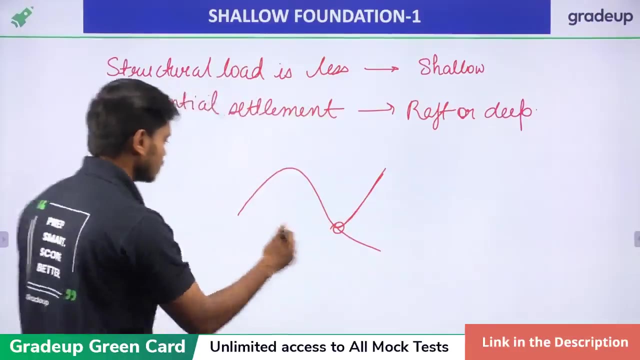 have to worry about this thing, that you are thinking in mind, that you are getting demoralized or anything else. you don't have anything to lose. you are going to gain only. so just concentrate, just focus on the gate. only this is the time and just learn new things, okay. 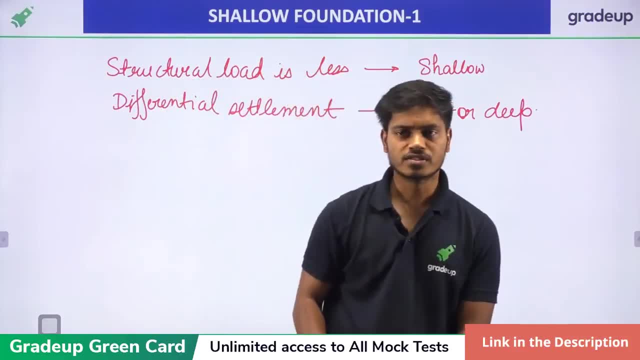 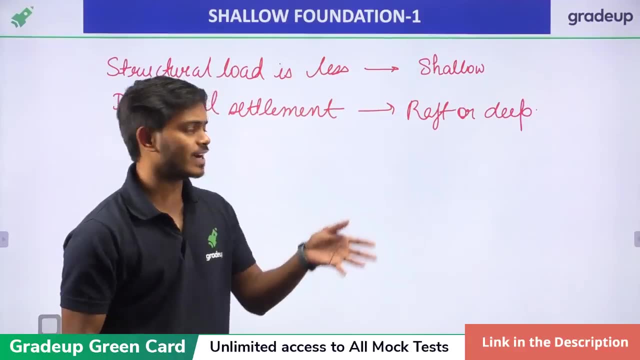 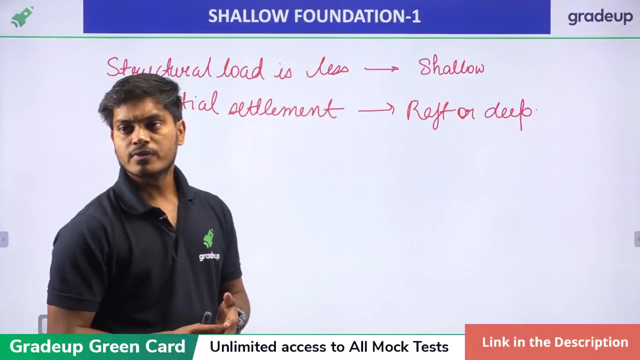 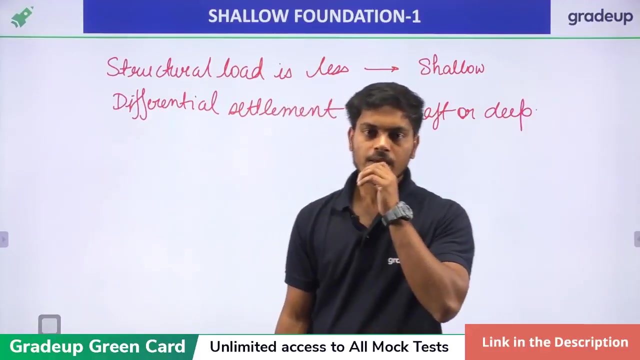 this is not the end. all right, this is not the end. please, you are not late, Harshit. okay, we just introduced that. shallow foundation is there and deep foundation is there. okay, concept karne ke baad bhi question nahi ban paata. okay, this is the only. this is the. this possibility only occurs if you have. 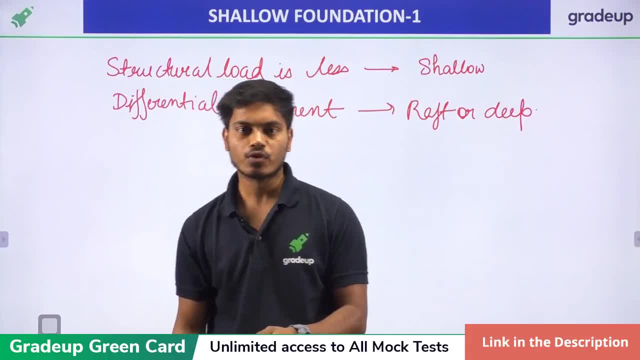 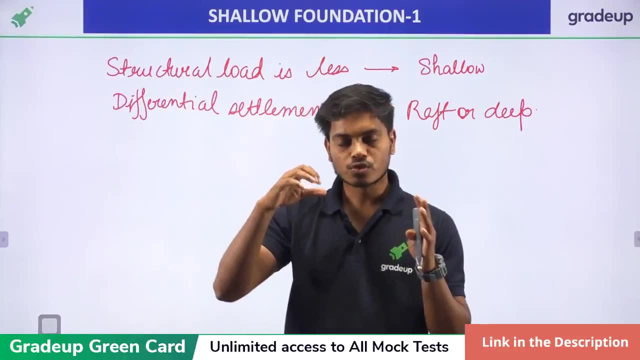 solved a less number of questions. okay, this is not important. that if you have studied the concept, you are going to be able to solve a less number of questions. okay, this is not important that if you have studied the concept, you are going to solve the question because one concept, okay, there are. there are so many. 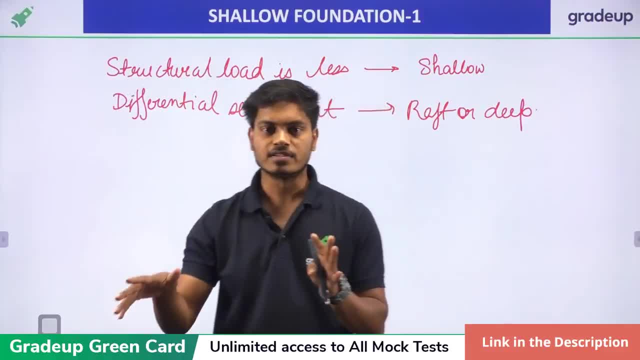 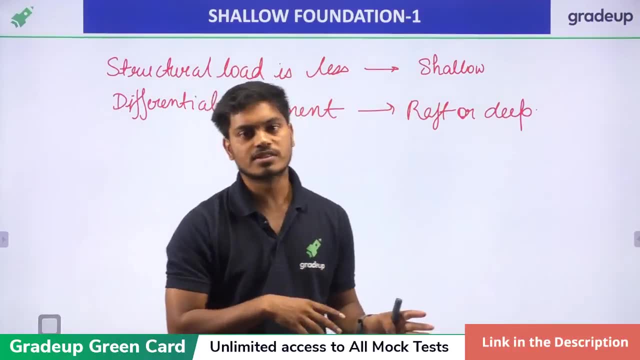 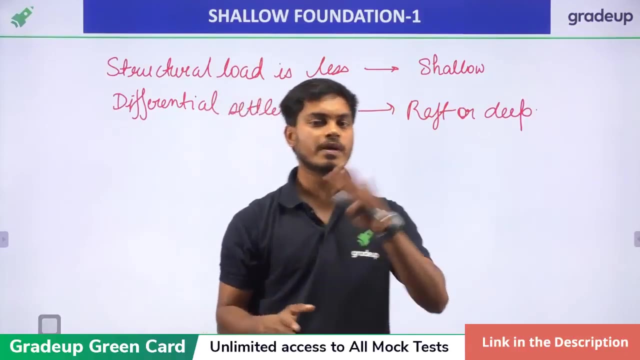 questions can be made on one concept with different, different styles. so it Doesn't matter that you will get that question if you know the concept, but how you can get that concept by solving the total number of type of questions that could be made on that concept. okay, and this: 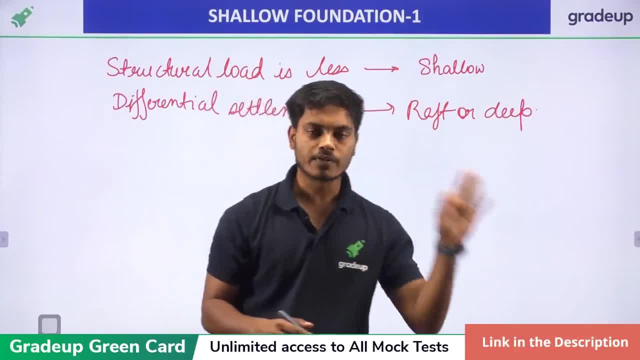 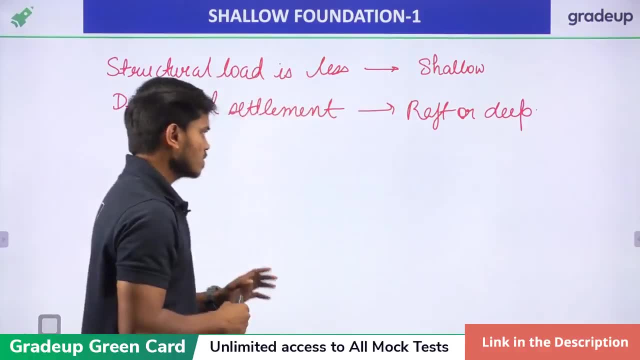 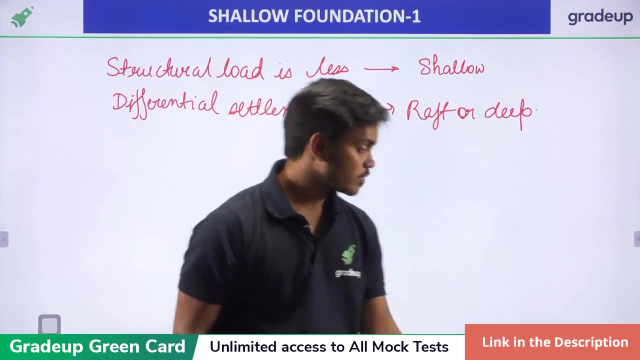 will be only happening if you will solve more questions from more questions previous year and also if you will attempt more number of test series. all right up that, okay. so, uh, we have reviewer. okay, swelling pressure: differential structural load is heavy. then you have to use pile foundation or deep foundation. it is done if there is a 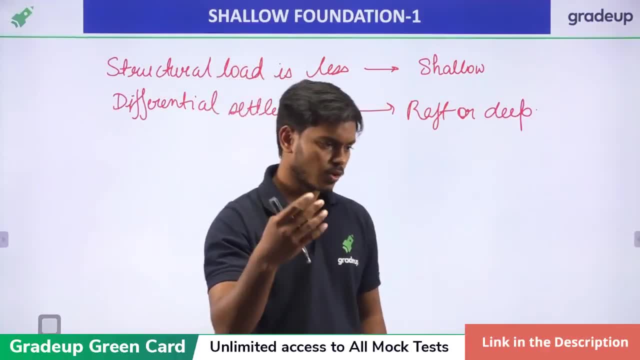 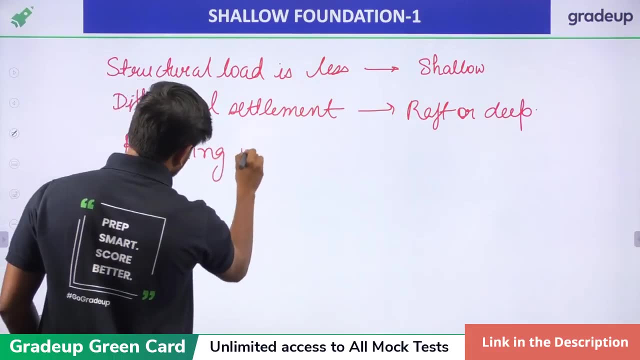 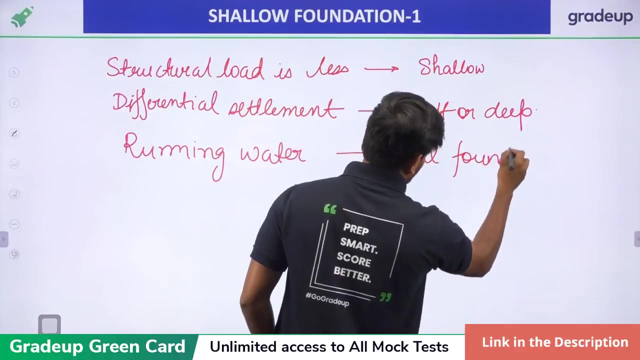 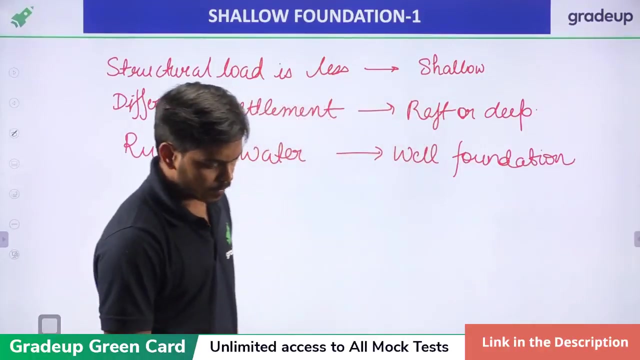 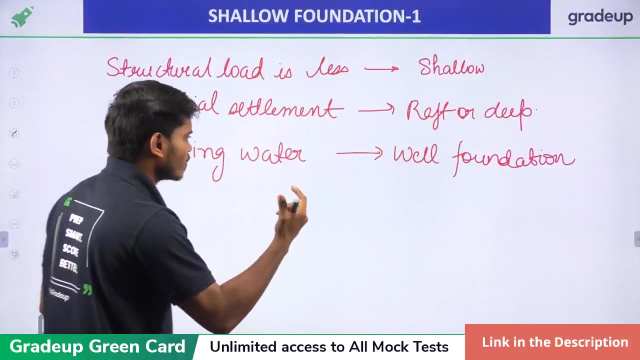 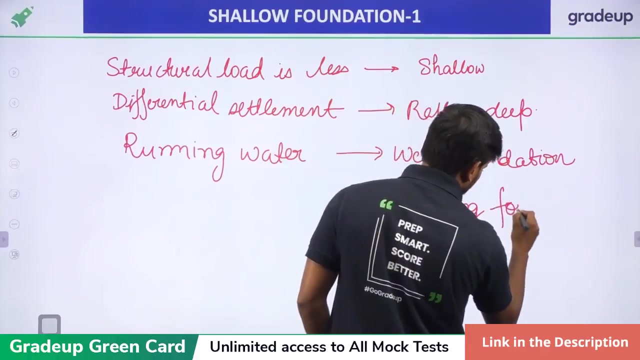 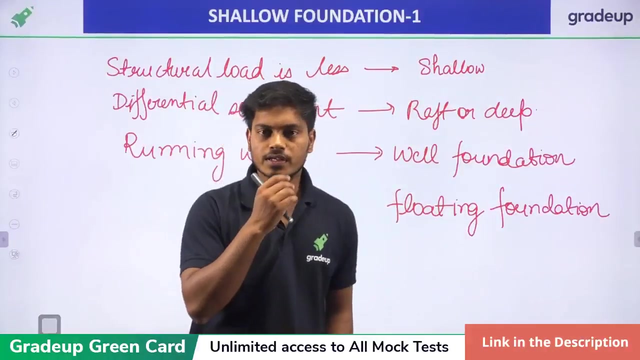 foundation which you have to made in what you can say running water, running water. then you have to use well foundation, well foundation, okay, and there is this very interesting: there is very uh interesting, uh foundation there available which is floating foot foundation. so in this kind of foundation, what we do is we excavate the soil. okay, we excavate the soil. 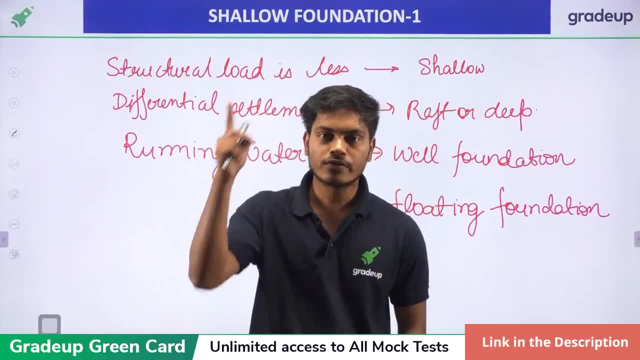 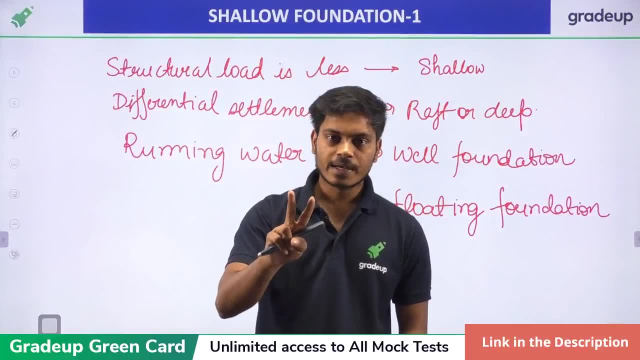 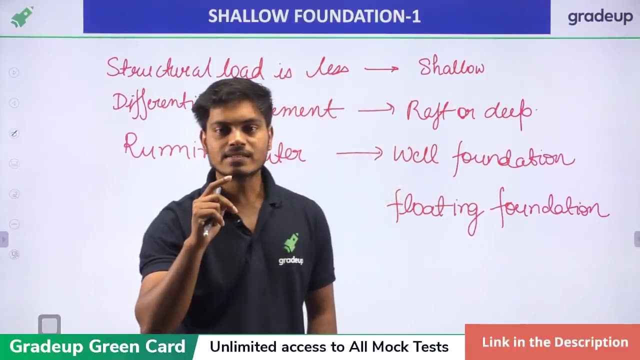 whose weight? whose weight will be equal to the weight of the building plus weight of the foundation. okay, two benefits will be there, like one: you don't have to like make this uh, pile foundation or anything. second is you are getting a parking space, or you can say: 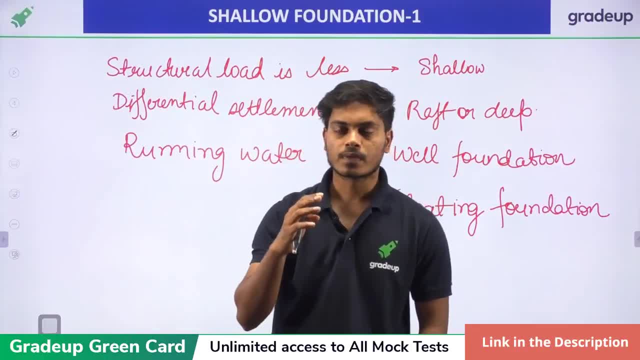 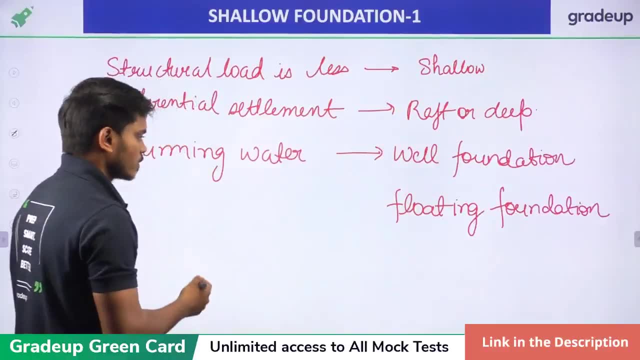 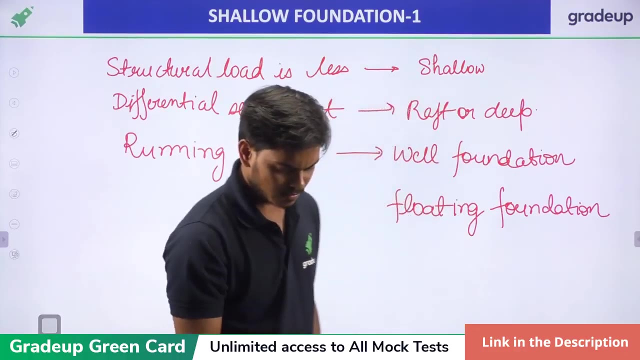 underground area you will get, so you can use uh accordingly. you can use it for parking or anything else, whatever is the purpose. okay, so floating foundation is there and so this is it. like nothing much is there. this is like a general stuff. okay, this could be uh asked in. 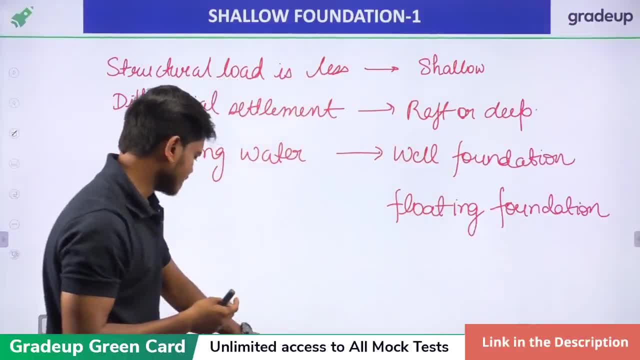 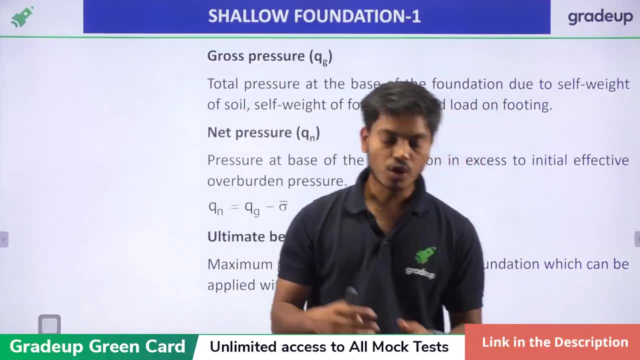 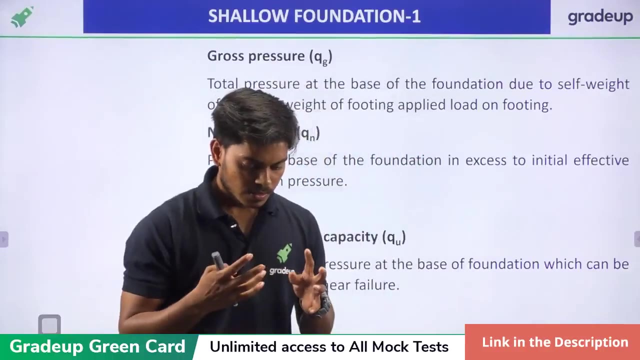 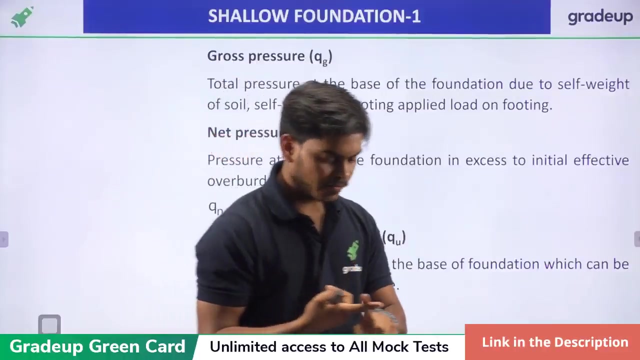 one one marks question only. okay, so these were the types of foundation. you can say: see, uh, there are types of pressure that your foundation is going to experience. okay, the thing is, the safe load is actually based on two criterias. first is safe load based on shear failure and safe load based on 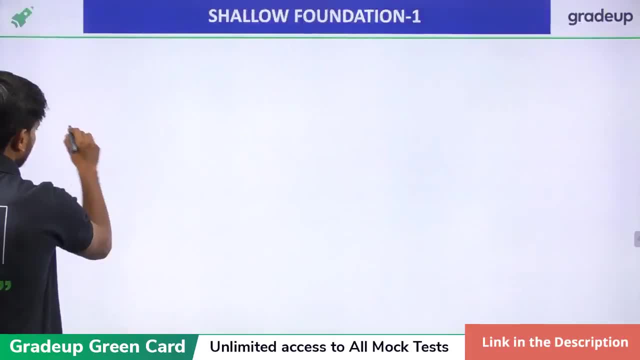 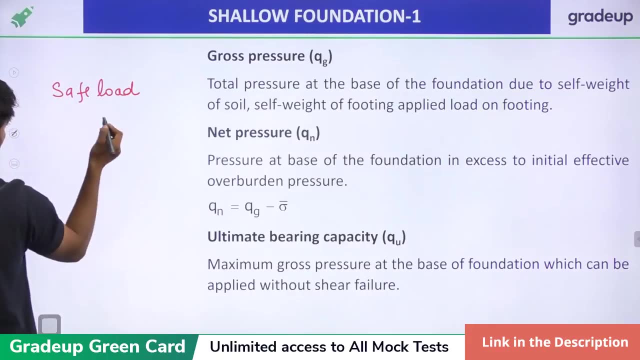 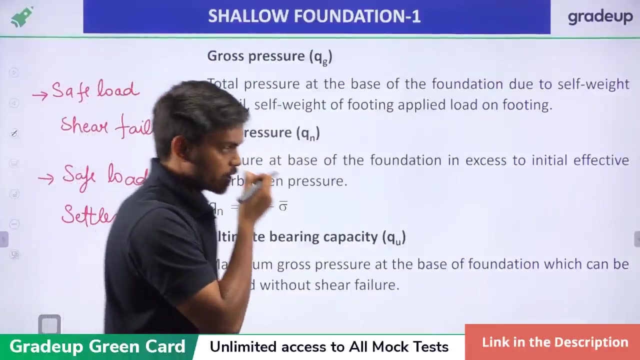 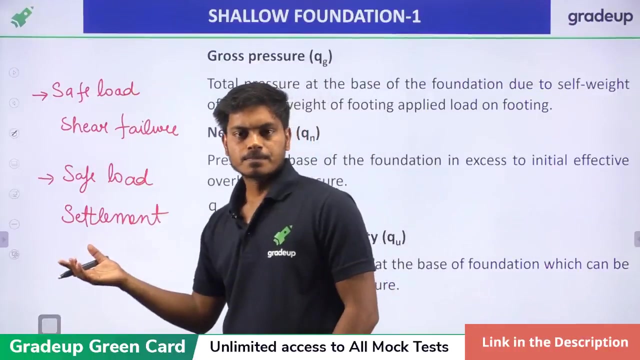 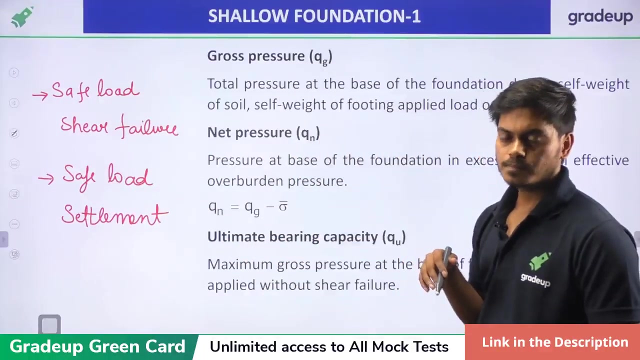 settlement: safe load based on shear failure. another one is safe load based on settlement. okay, so can you please tell me, if i want to design the foundation or the footing, what should i take? minimum of both of them or maximum of both of them? minimum or maximum? which value i have to take? 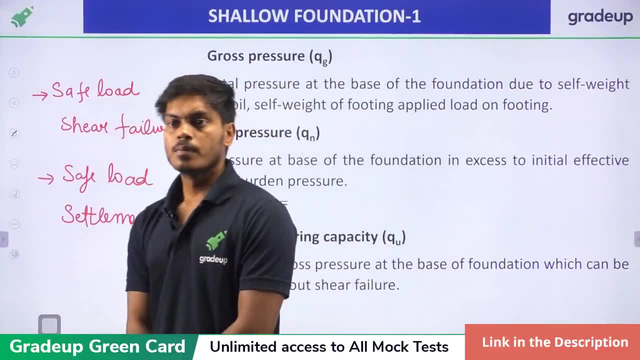 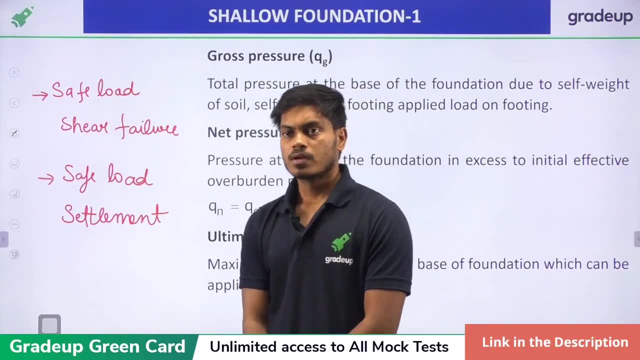 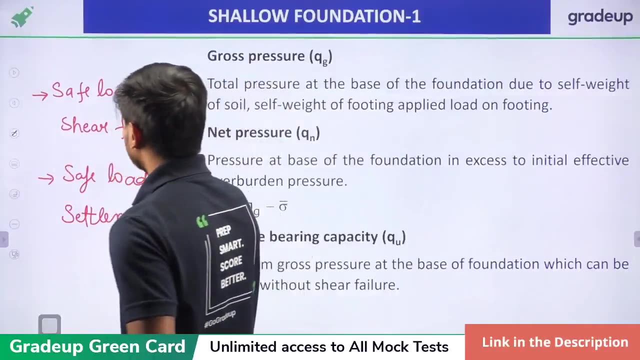 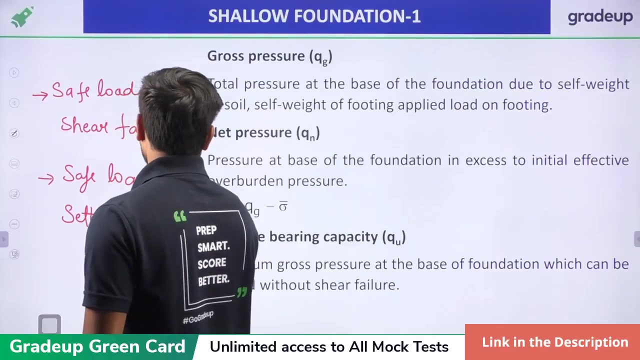 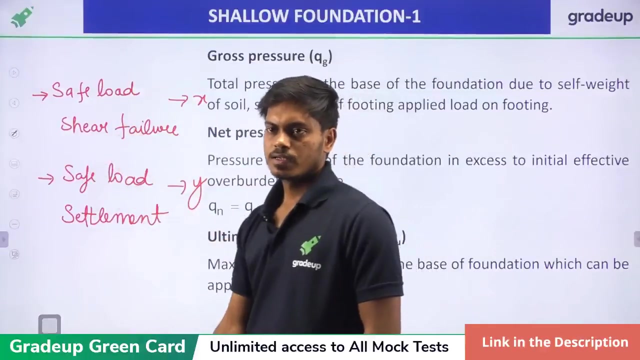 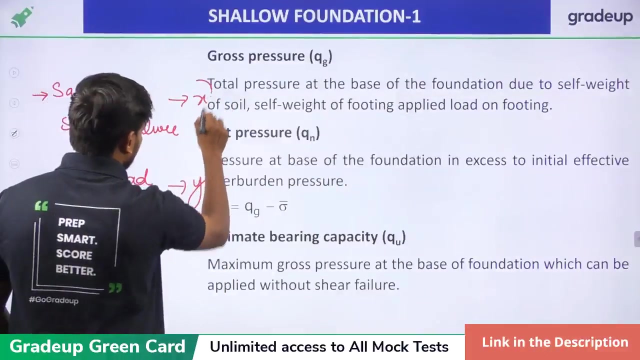 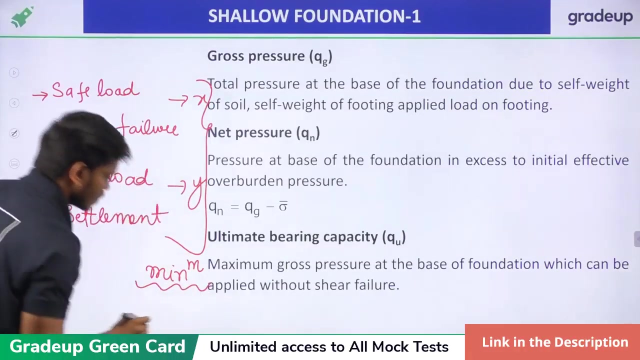 maximum. okay, minimum minimum minimum. province is maximum. just, uh think, practically i have two criterias. okay, one: we have safe load for shear failure. all right, suppose the value is x, one is y. okay, so this is the Poliera. we actually choose safe load as a minimum minimum low or minimum low. 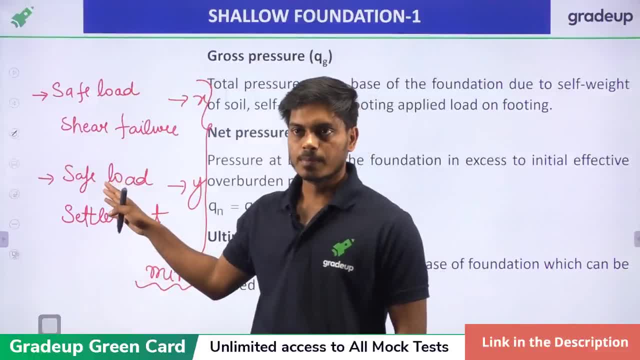 in fact, the mean angle is nothing but the minimum mean angle, a high or minimum minimum, minimum, minimum, default minimum, minimum minimum, no by that, which state yes when it consider, marginalize both the minimum values. trust me in the data field, safe load, encourage us to use the safe load. so in this case, we have to adopt the minimum, we have to adopt the minimum, the minimum value among both of them. so most of us have been corrected and most of you are correct. okay, most of you are correct and the answer is only minimum. right, pois, I did. 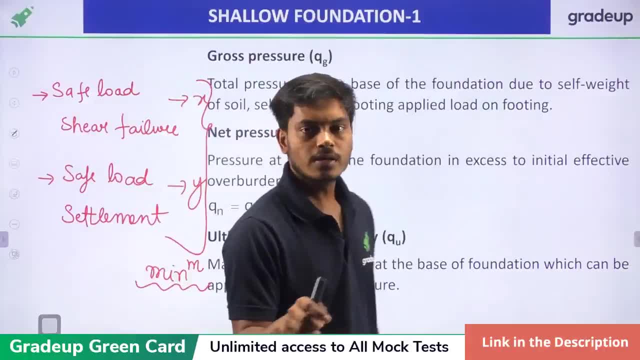 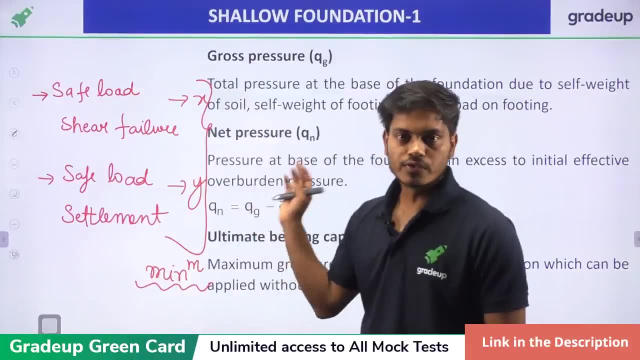 NT NO, ADOPT THE MINIMUM VALUE OF THE BOTH OF THEM. SO MOST OF YOU ARE CORRECT AND THE ANSWER IS ONLY MINIMALY, AND THE ANSWER IS ONLY that you have to consider settlement only. you have to check for both. so whatever will be there, you have to take the minimum value for that, okay. so if 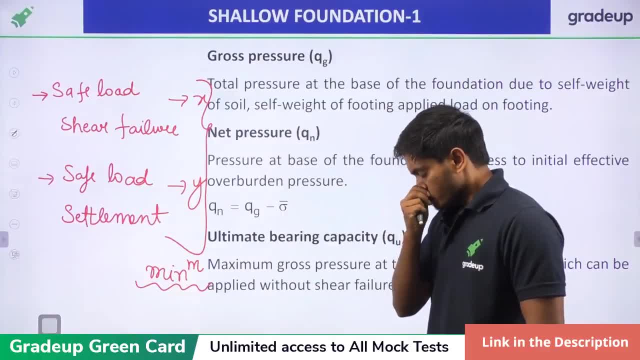 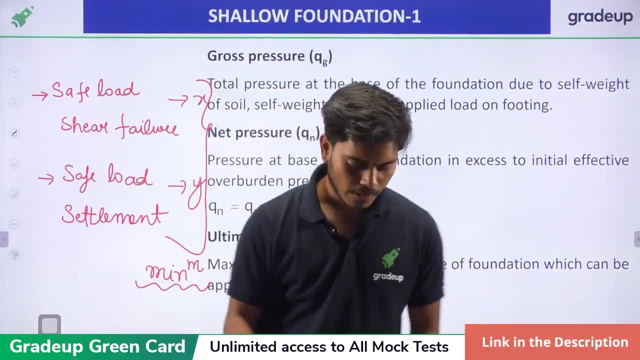 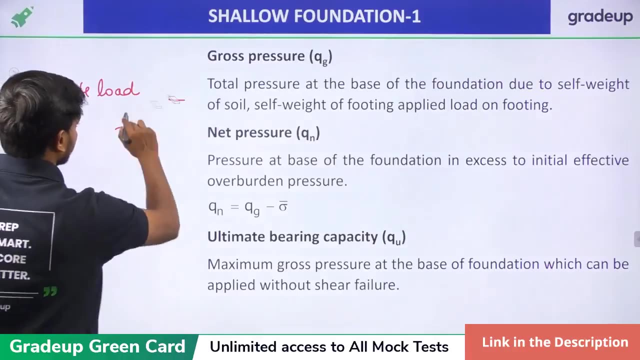 you will design for minimum. there will be sorry. there will be a safe load that you will get will take care of both of them. so you don't have to be specific about that. you have to take settlement, he settlement or shear. so, one by one, we are going to talk about it. shear failure: what is shear failure? type of shear. 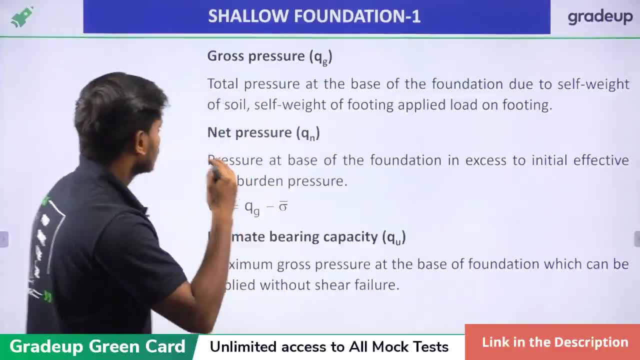 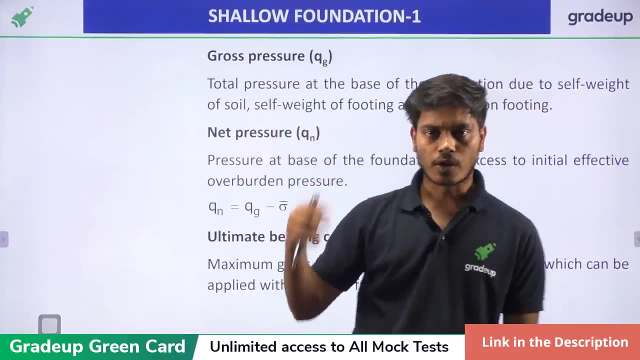 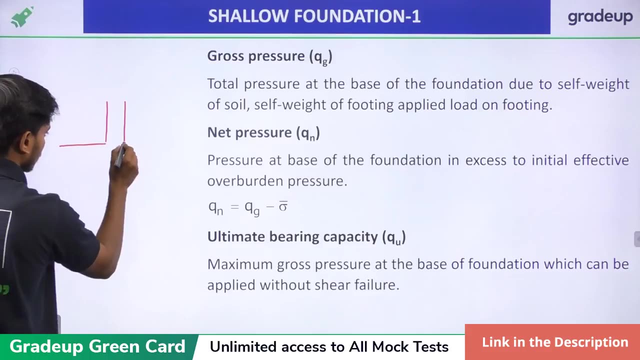 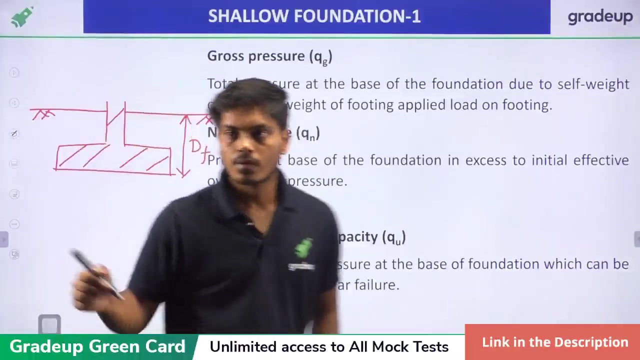 failure, we'll see. all right. so first we have to see what type of pressures are there which is applied on your foundation. suppose you have a foundation here. I'm just drawing a rough diagram. okay, suppose this is your foundation here. this is your ground level. okay, this is the depth of foundation. all right, and 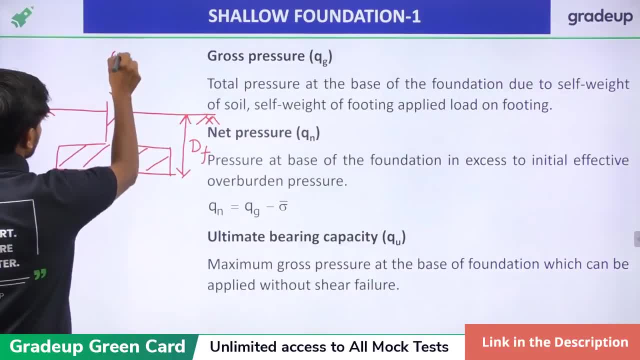 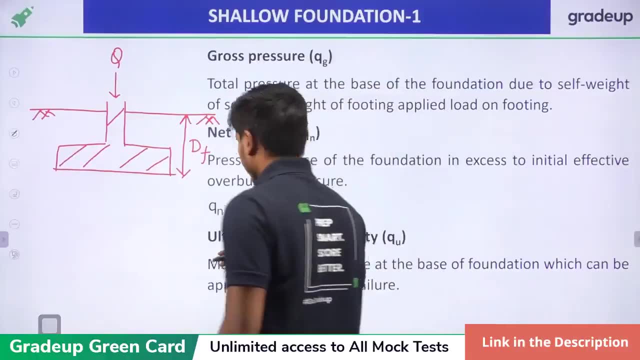 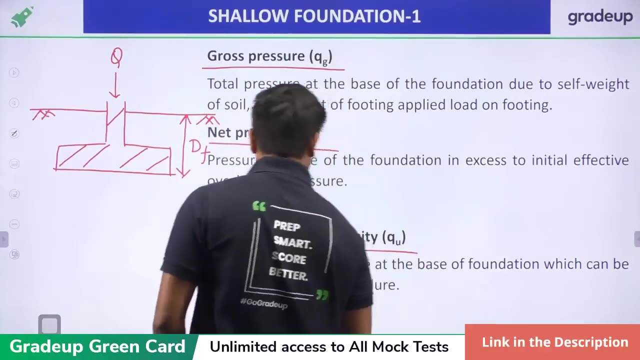 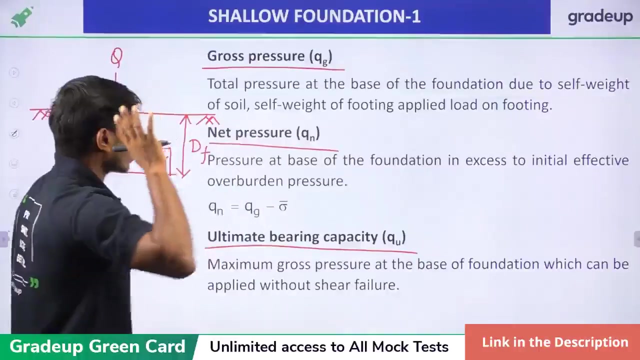 suppose the load here is Q, all right, so one by one we'll see all type of pressures. one is gross pressure, net of pressure, then ultimate bearing capacity is different thing we'll see one by one. so gross pressure here is the total pressure at the base of the. 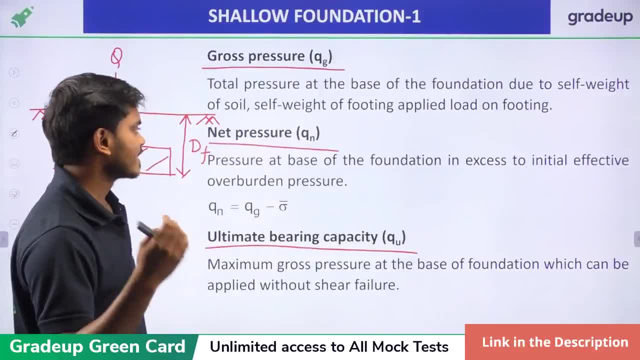 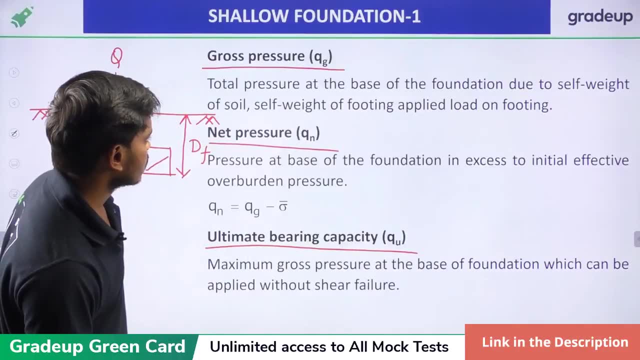 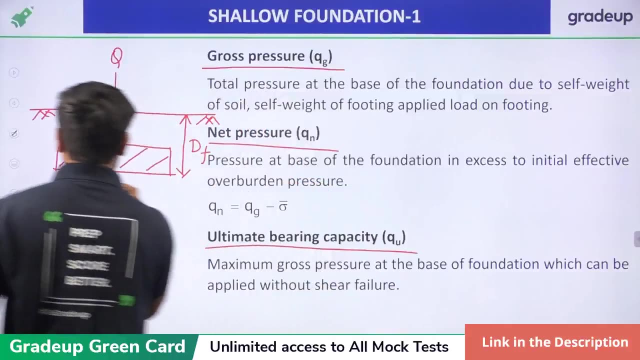 foundation due to self weight of soil, self weight of footing applied load on footing. cell weight of footing applied load on footing. the thing is, only thing, is that you have to consider we are talking about at the base of foundation. I'll use different color at the base of. 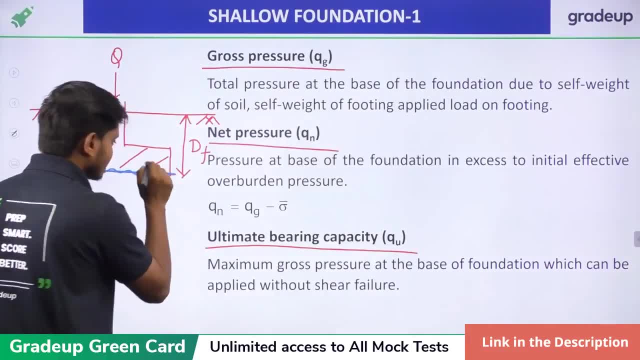 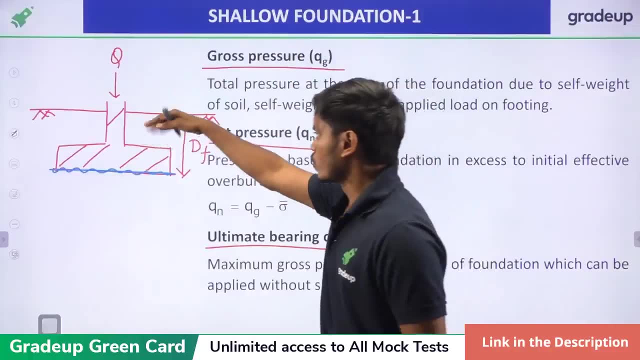 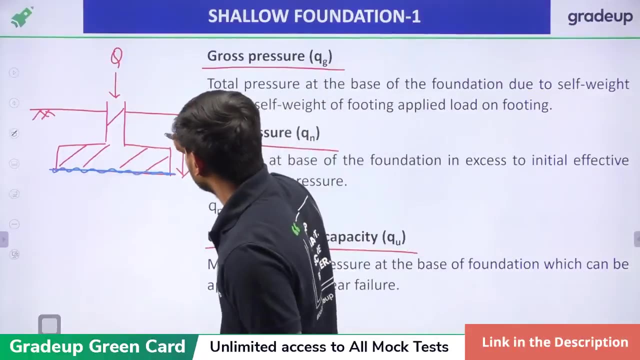 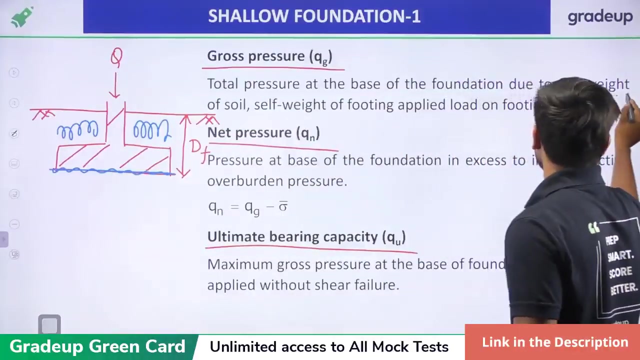 foundation. all right, so at this particular position, whole pressure, which means the applied load. okay, so, because of this, first, the self weight of this particular foundation. one second, this self weight of this soil as well, which is there. so you can say that, due to self weight of soil and self weight of, 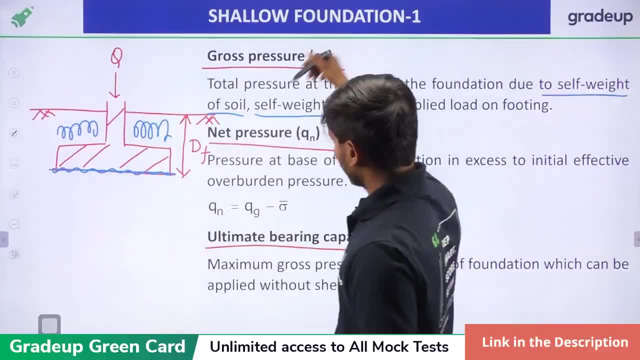 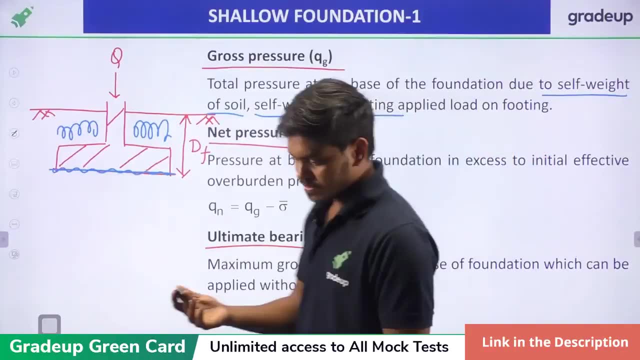 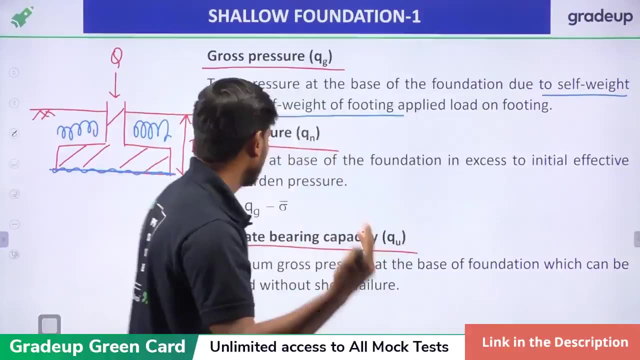 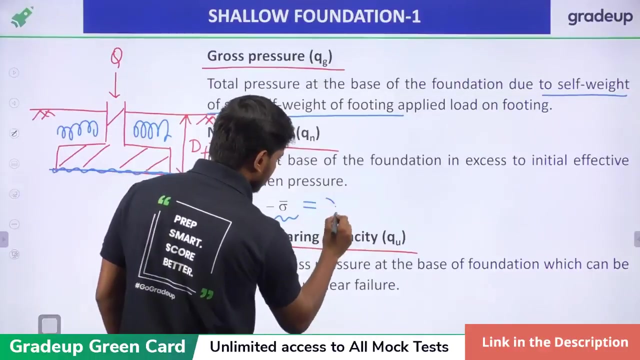 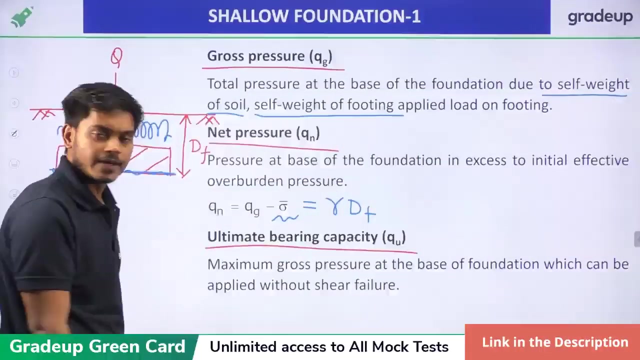 footing. all right, so this is your gross pressure. next is net pressure. see, net pressure is what? net pressure is? nothing but the gross pressure minus the gross pressure, minus effective overburden pressure. overburden pressure, which is represented by this Sigma, dash is nothing. but this is Gamma, CF, gamma, DF, gamma is bulk here. all right, so you just have you. 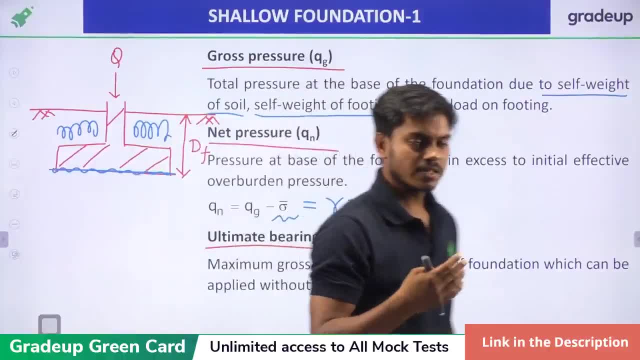 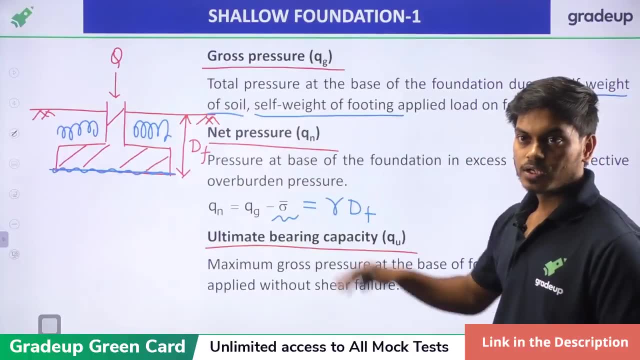 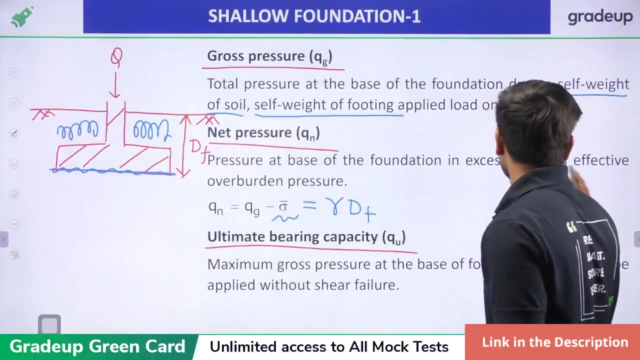 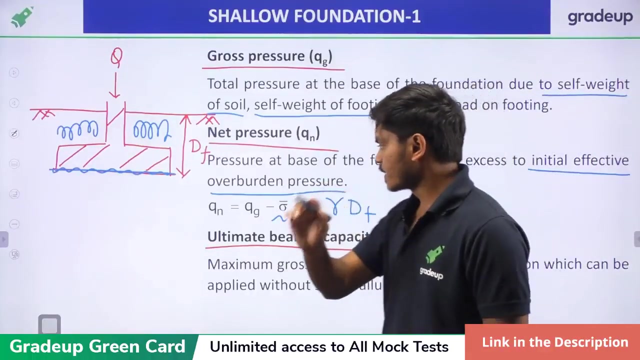 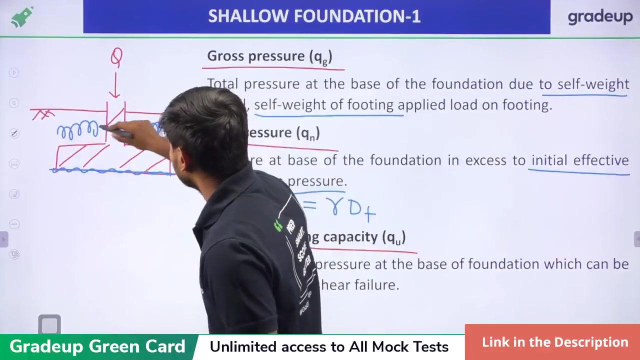 what you are doing is you are just, you are just getting the pressure, which is only by the foundation itself. all right, so this is your net foundation, which is gross foundation minus gamma or initial effective overburden pressure. all right, and mathematically, magnitude is gross pressure minus gamma, DF. gamma DF is what this is, the unit weight of. 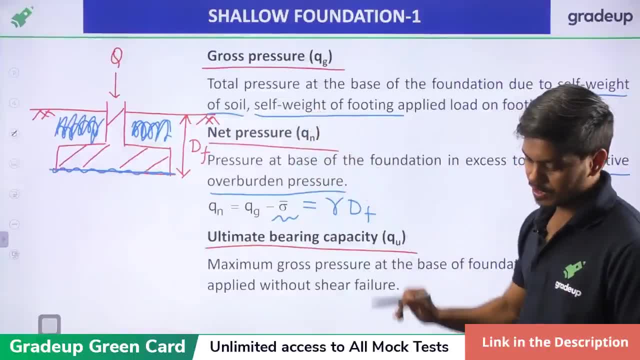 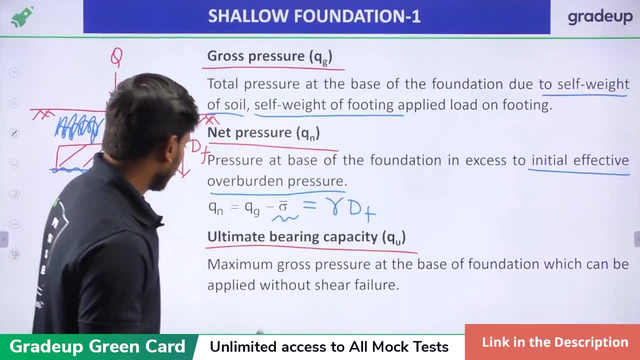 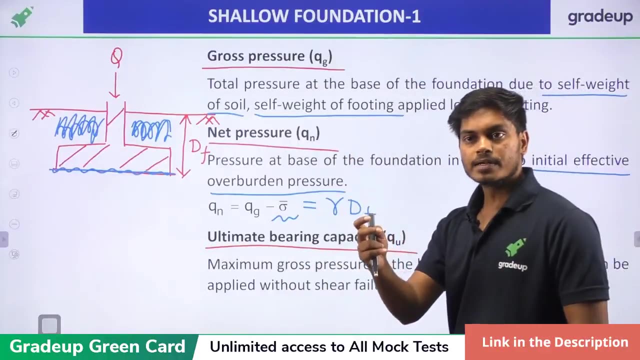 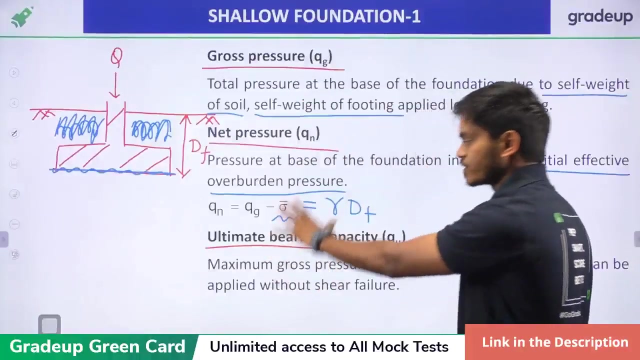 this soil gamma and up to the depth of foundation. this is your net pressure. all right, now, what is ultimate bearing capacity? now? this is important for us. okay, what is ultimate bearing capacity? it is now. look at this carefully. okay, you don't get confused in between gross pressure and ultimate pressure, all right? 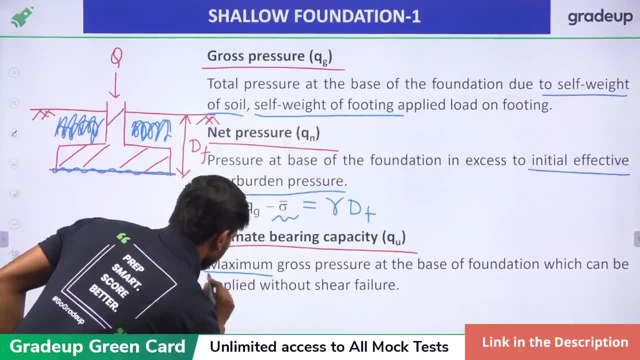 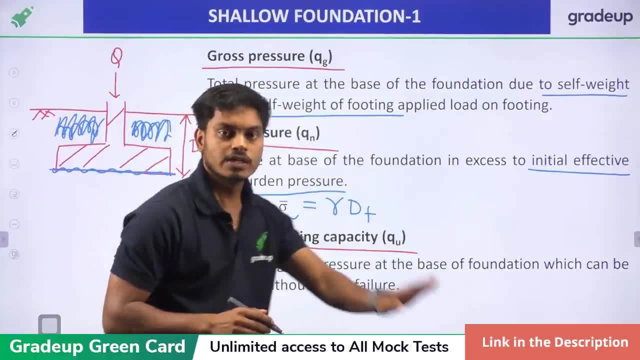 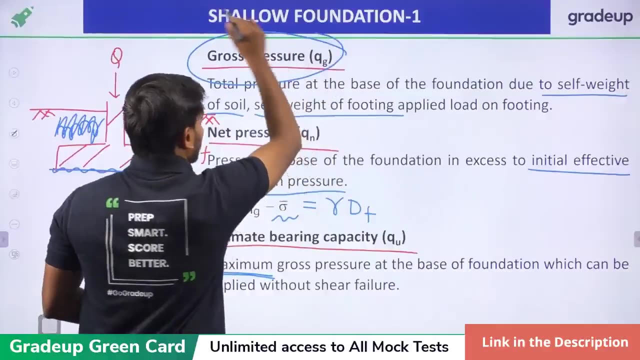 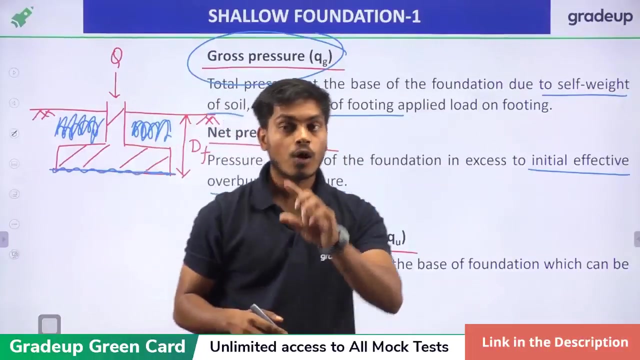 maximum- okay, I'll just make it easier for you. maximum gross pressure at the base foundation which can be applied without shear failure. okay, this is the maximum gross pressure, maximum gross pressure that can be applied without shear failure. or you can also say it is the minimum gross. 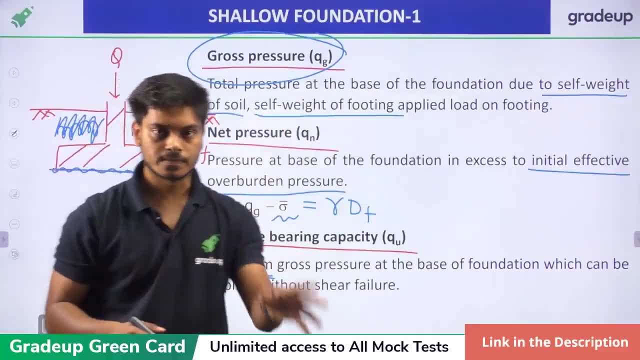 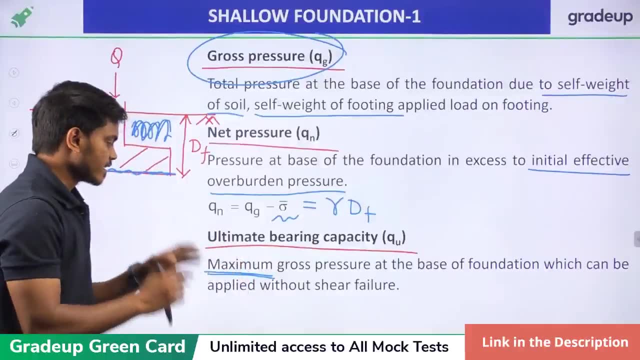 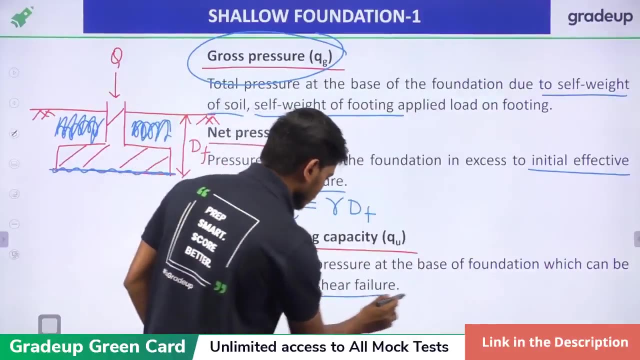 pressure at which shear failure will begin. all right, are you getting this? two sentences, these two are same, only first. it is the maximum gross pressure, okay, at which there will be you we can say there will be no shear failure, or you can say it is the minimum. 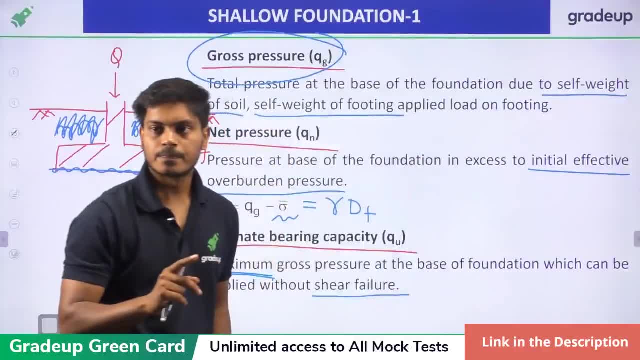 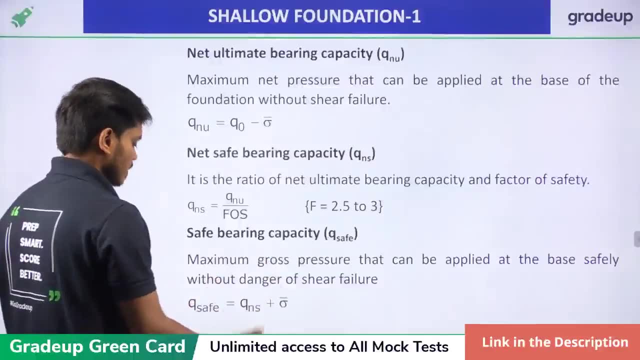 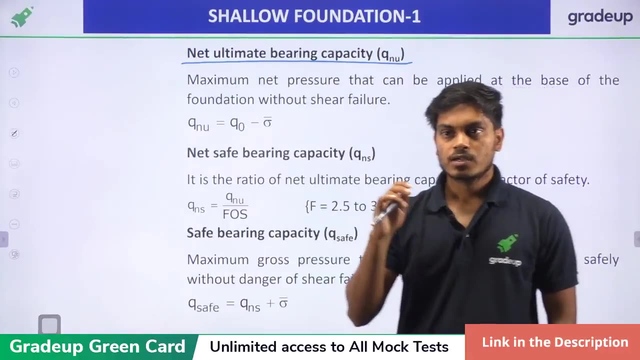 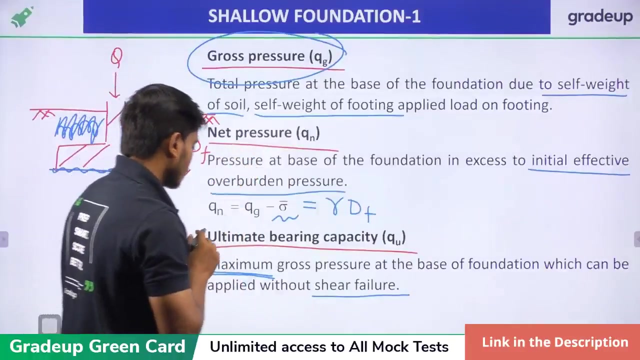 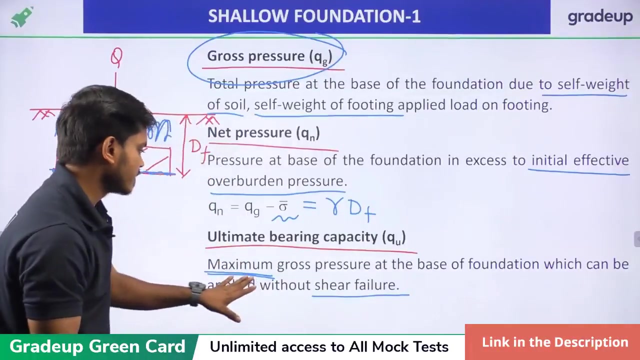 gross pressure at which the shear failure will begin. all right, so this is your net bearing capacity. sorry, ultimate bearing capacity. then we have this another term, which is net bearing capacity. you can understand. okay, I'll tell you again, hmm, hmm. so, ultimate wearing capacity. one statement is clear: okay, hi roshan, maximum, it is the maximum. 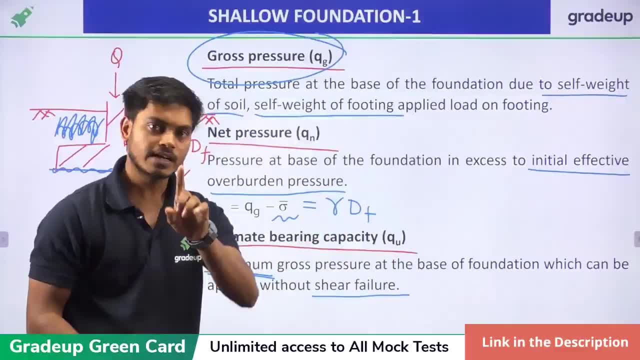 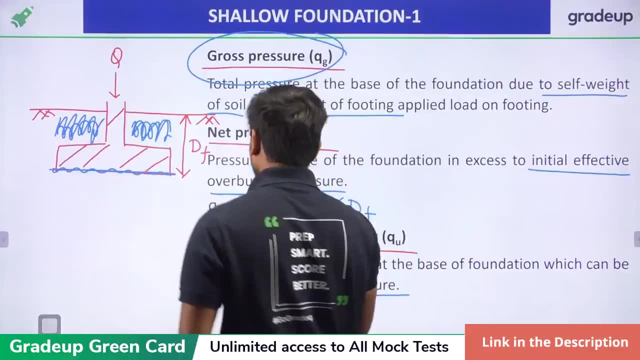 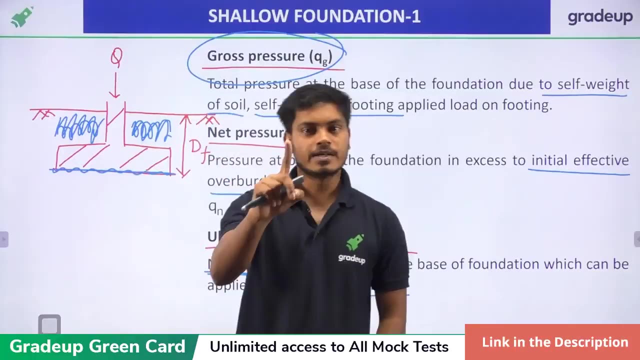 value of gross pressure which will be applied on the foundation and there will be no shear failure. all right, suppose this is my foundation and this gross pressure i'm increasing, increasing, increasing. and there will be one point: there will be one magnitude of gross pressure, after which, after 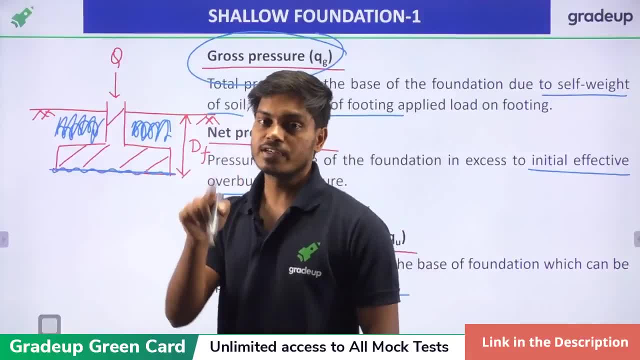 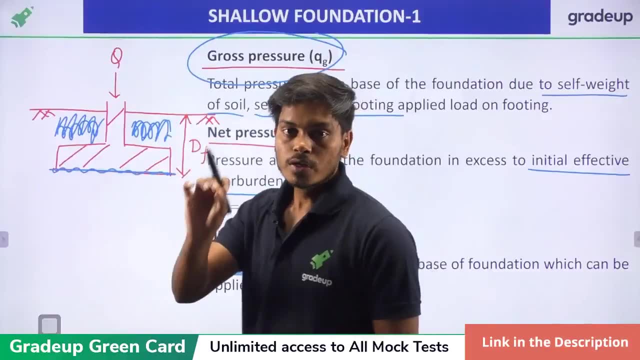 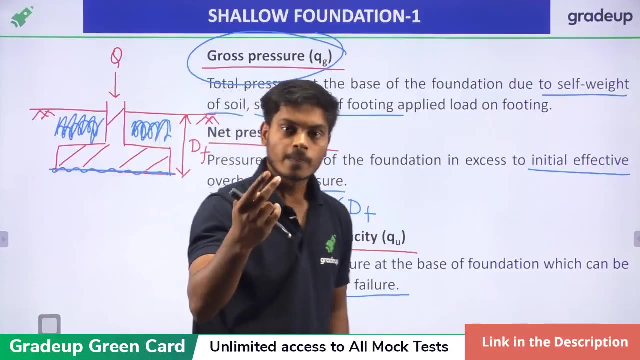 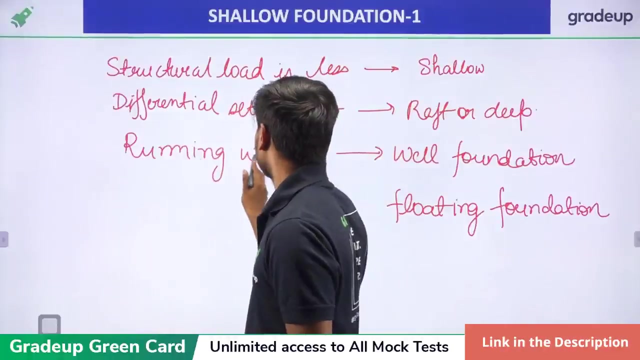 which it will fail. okay, i'm saying after which it will fail. so that means that particular pressure is the maximum value which this foundation can take without failure. all right, abhinash. next thing after that, after that maximum value, this- uh sorry, this foundation will begin to. 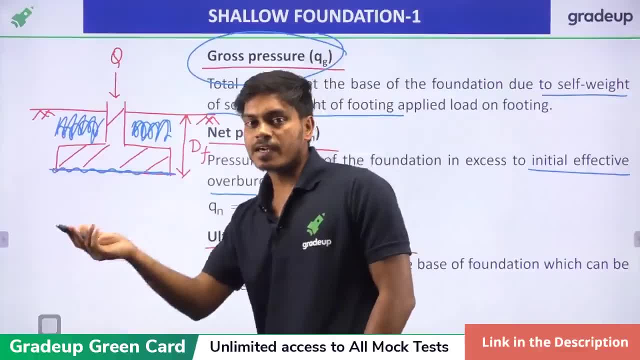 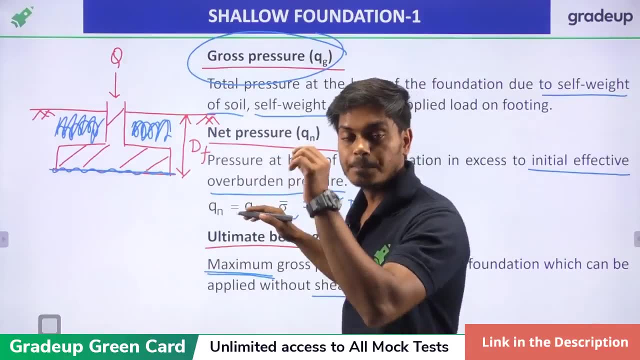 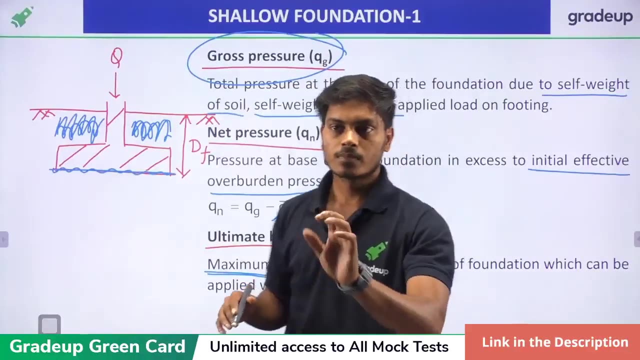 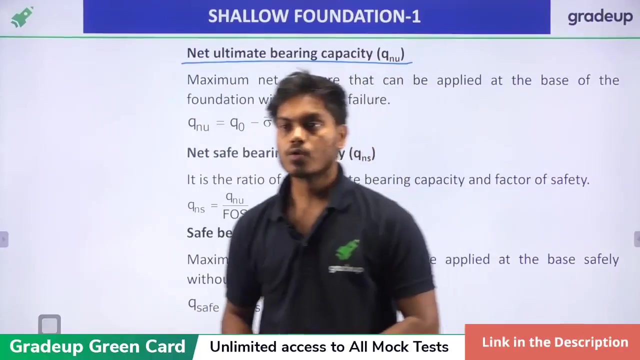 fail. so that's why i can also say that that particular pressure, which is the maximum gross pressure, is the minimum value of the pressure at which shear failure will begin. okay, okay, got it. thank you so much. uh, how can calculate the settlement of the footing? uh, we are going to discuss this. 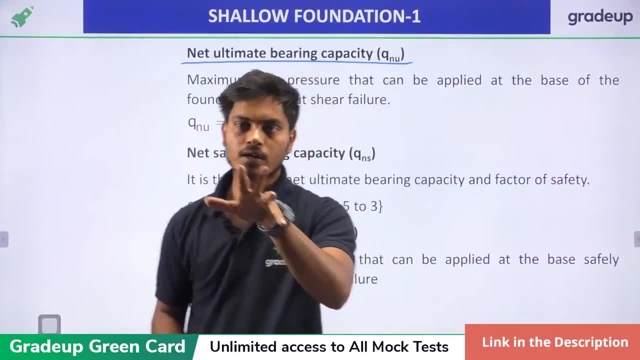 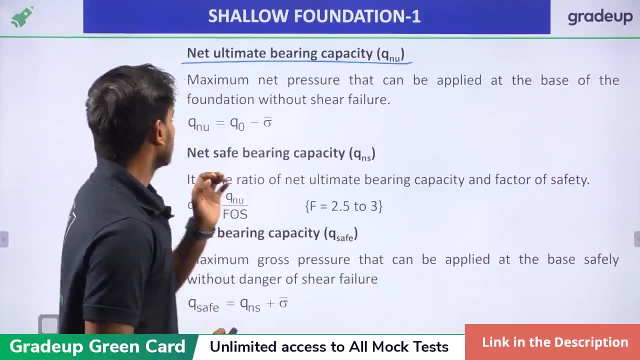 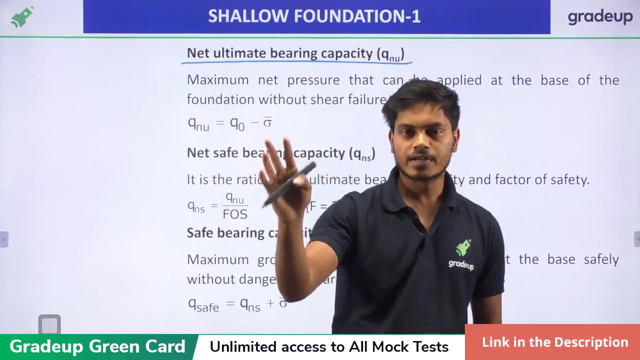 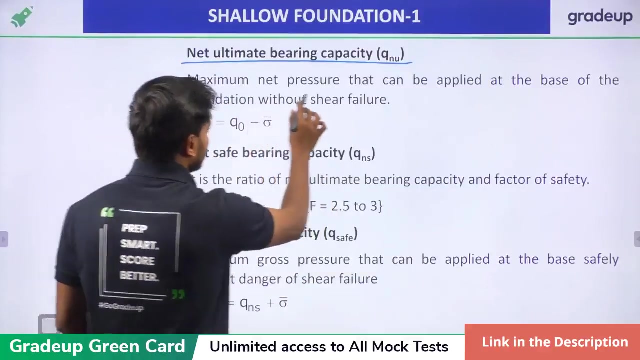 don't worry, but this footing thing, uh, it was there also in consolidation chapter. if you have missed it, you can watch the video. okay. net ultimate bearing capacity: same as net gross pressure- it was net pressure, you know- minus the initial effective overburden pressure. so same thing i'm doing here: the maximum net. 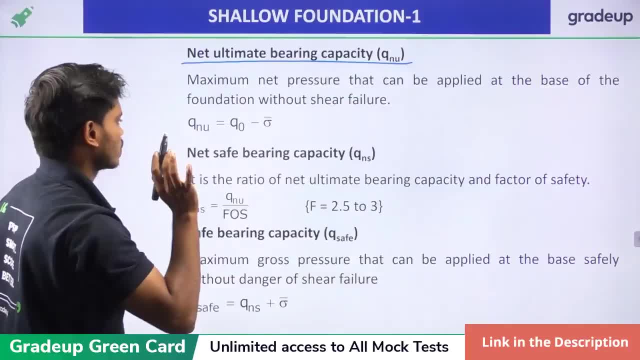 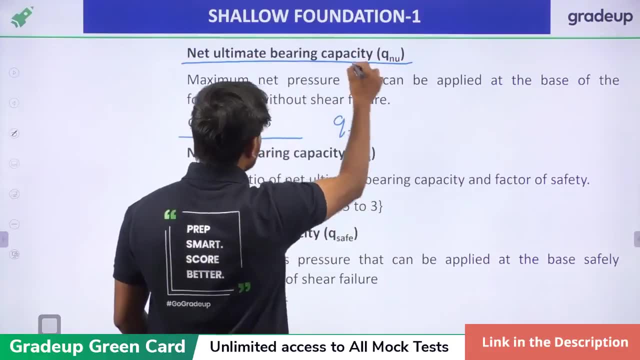 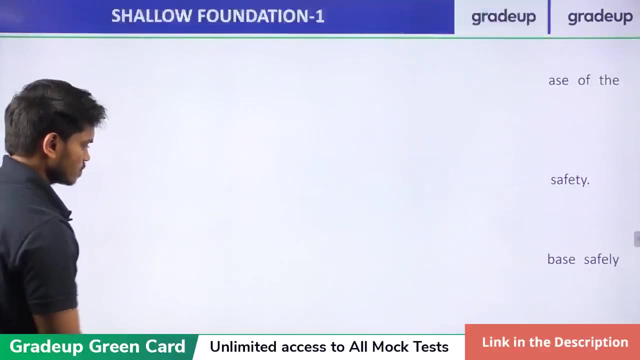 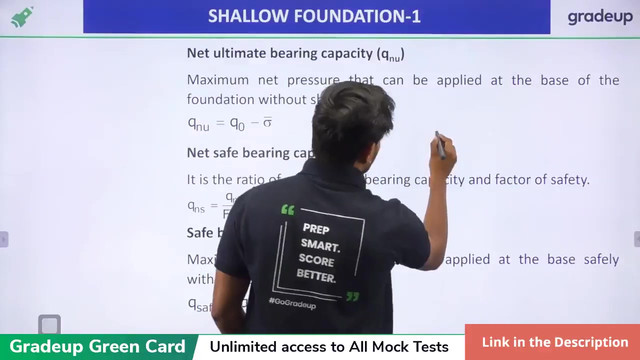 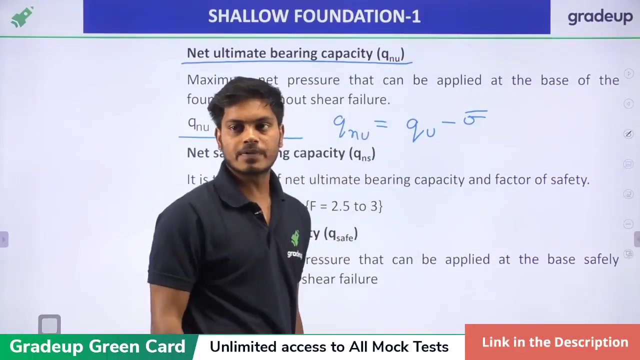 pressure that can be applied at the base of the foundation without shear failure. similarly, q and u- is what q, which is net ultimate bearing capacity, is equals to, is equals to this capacity, which is ultimate bearing capacity: ultimate bearing capacity minus initial effective overburden pressure. okay, so this value is nothing but Q, u minus gamma. 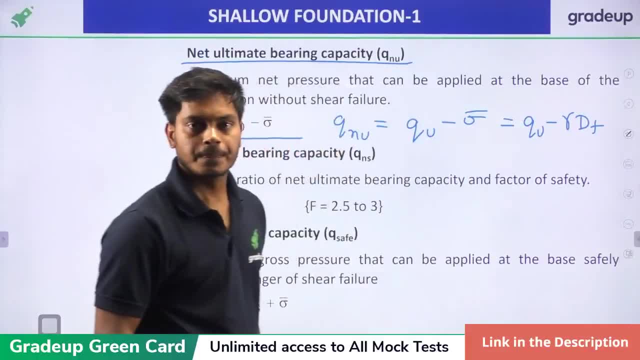 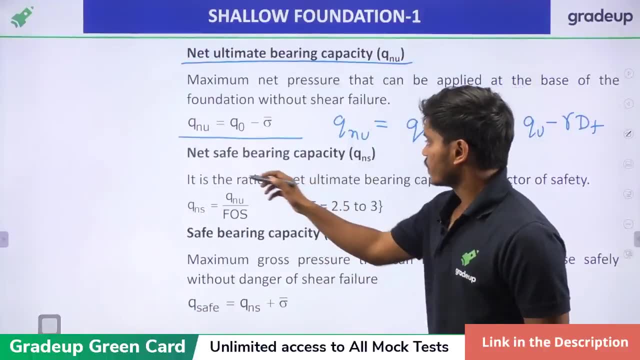 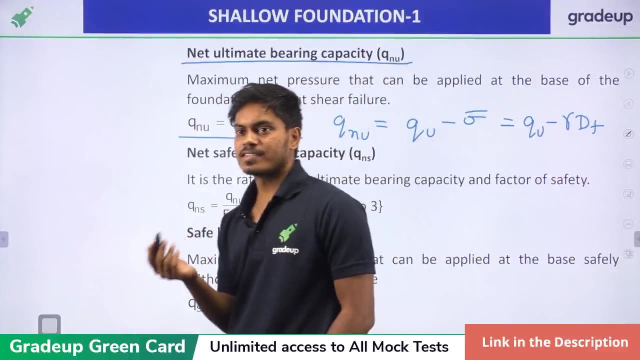 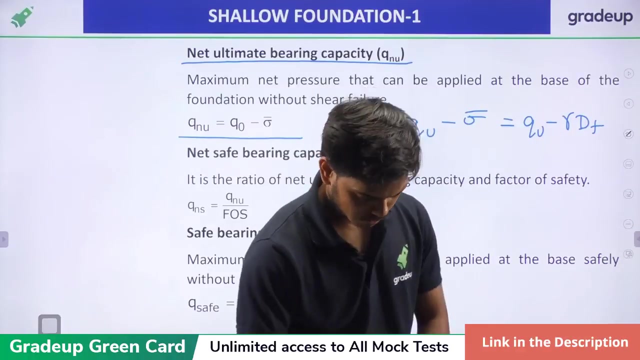 DF. all right, gamma DF. next we have net safe bearing capacity. so if you make, if you want to make this safe, then definitely you have to use a factor of safety here. all right, let me check if I have, if I'm missing anything. no, we are go, we are going good, so here. 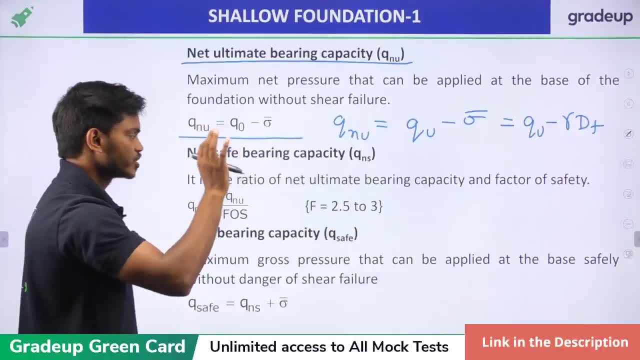 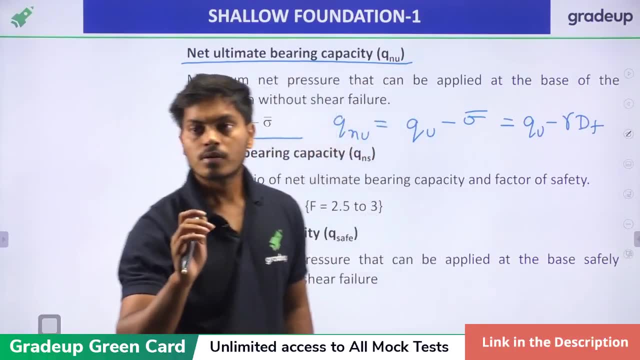 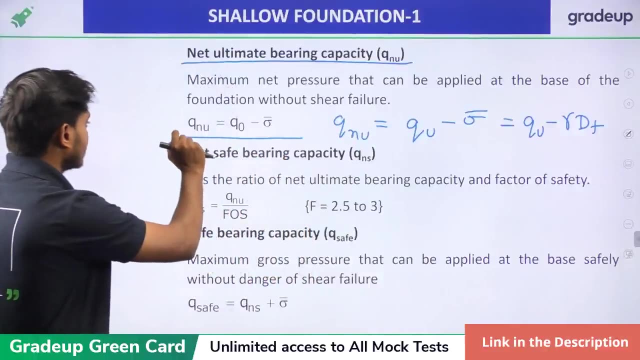 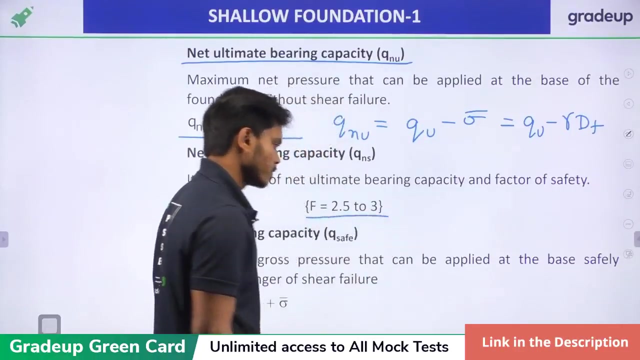 net bearing capacity is nothing, but it is the ratio of net ultimate bearing capacity and the factor of safety. all right, graph. we will see graph, don't worry, we have graphs. so net ultimate- here the Fos value, factor of safety value, could be 2.5 to 3. it will be given in the question, don't worry. okay, it will be. 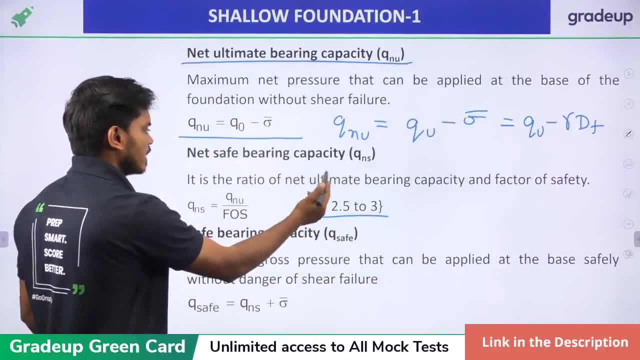 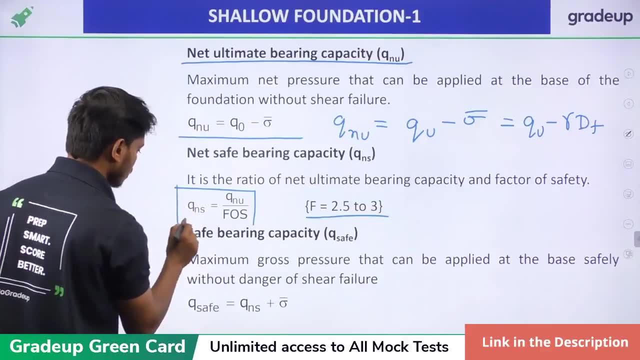 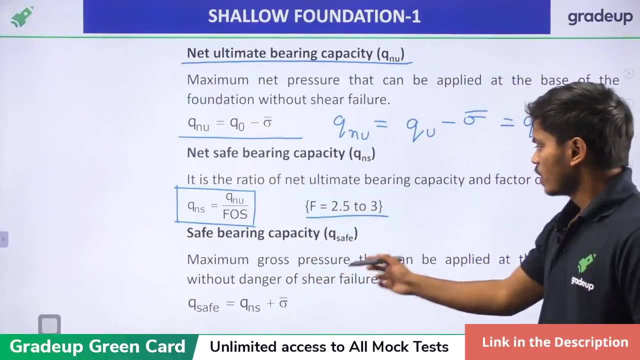 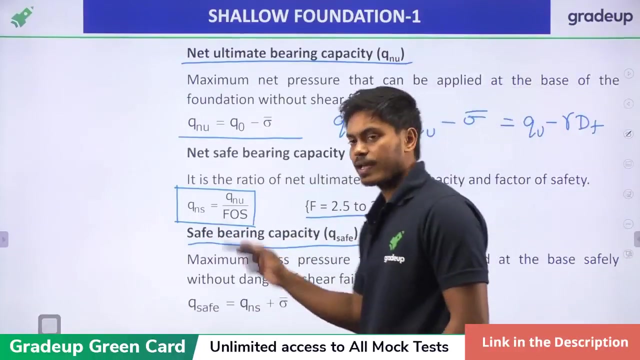 given in the question is the ratio of net ultimate bearing capacity and factor of safety here. so this is your net safe bearing capacity, all right, and I have to make it, make the, or I have to design the foundation for safe bearing capacity, all right. so what I have to do, I have the net value. if I need the whole value or the gross value, 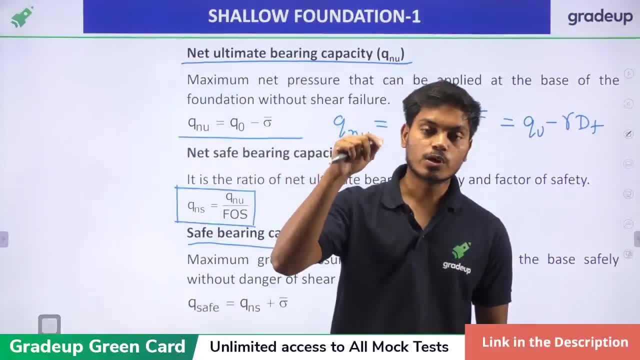 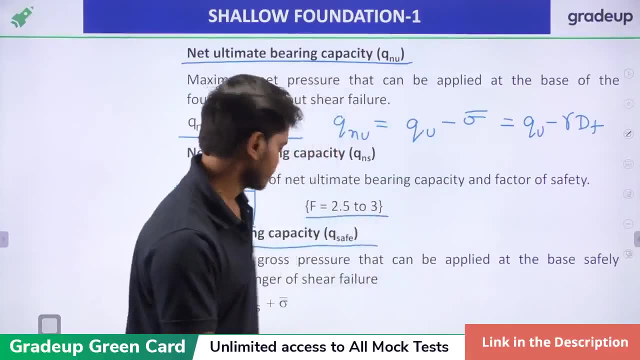 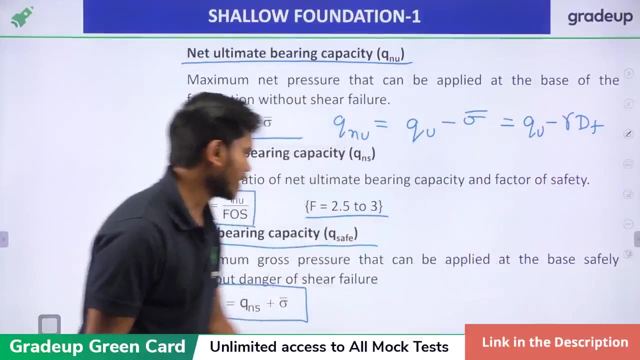 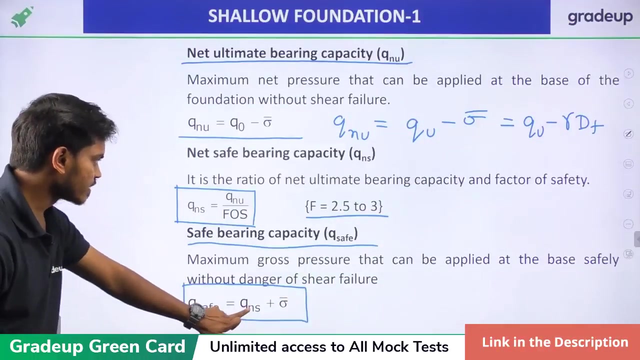 then what I have to do. the initial, or initial effective overburden pressure that I have deducted, I have to add it again here, as you can see. so maximum gross pressure that can be applied at the base safely, safely, without danger of shear failure, it is the net safe capacity or the net safe bearing. 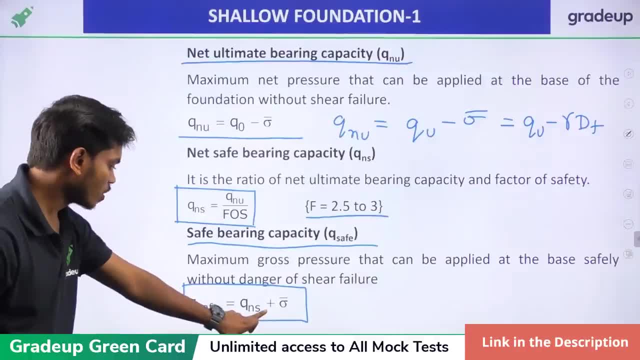 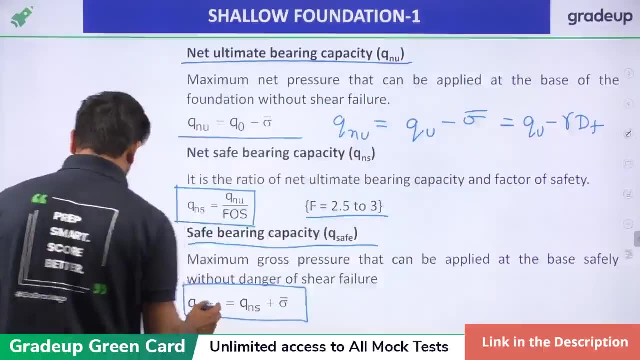 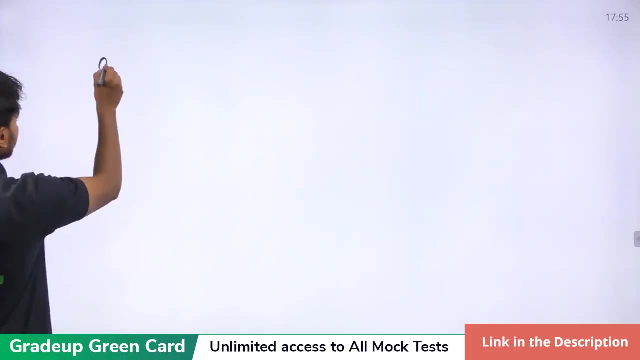 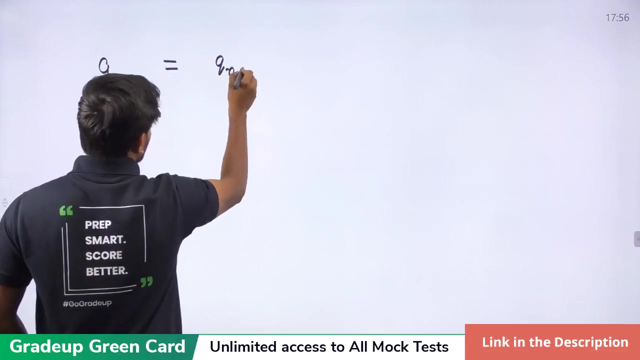 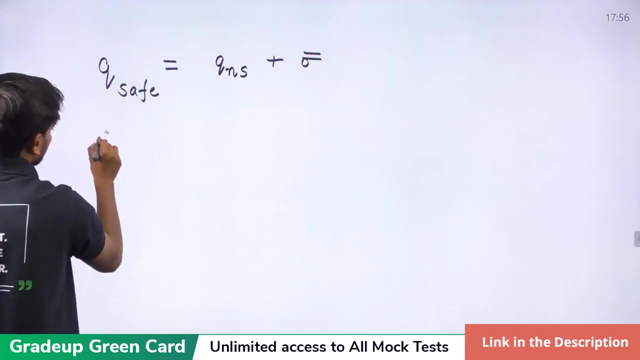 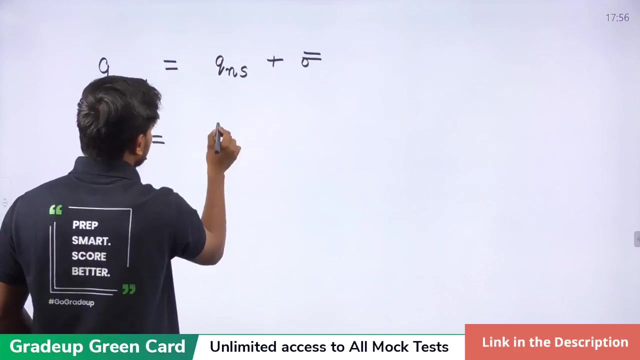 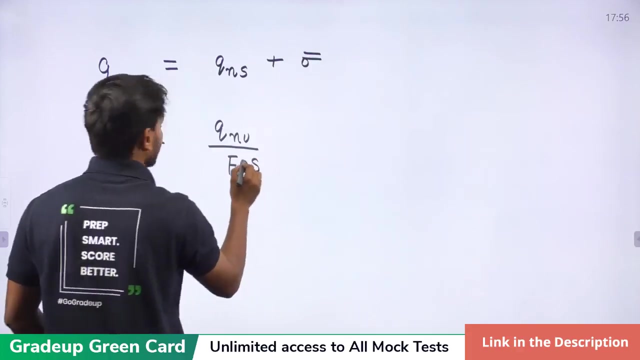 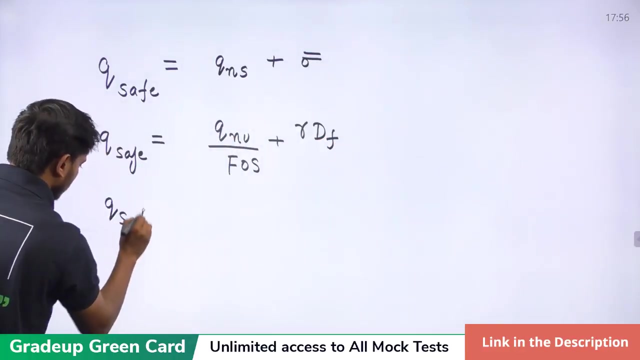 capacity equals to a plus the initial over effective, initial overburden pressure. so Q safe is what Q safe is equals to Q NS plus this. so if I write it, if I elaborate this, so what is Q NS? it is nothing but Q. and you divide by factor of safety, all right, plus gamma DF. and if I elaborate further, then what? 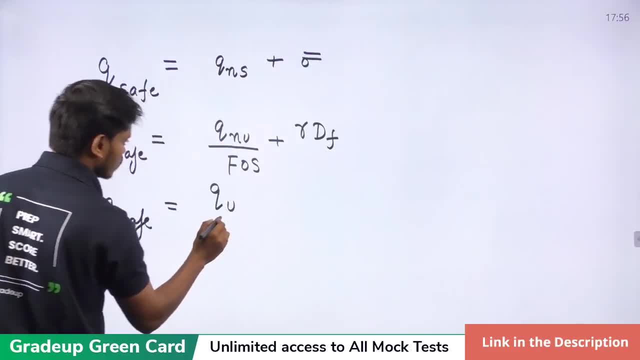 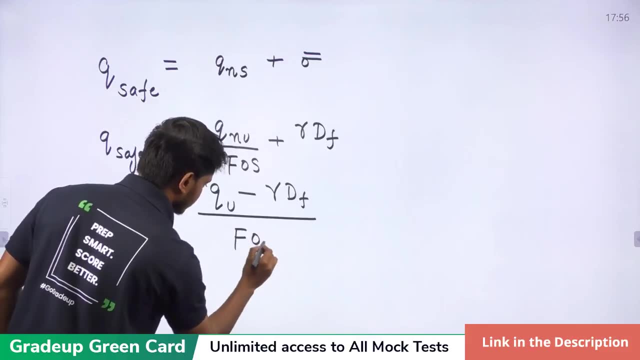 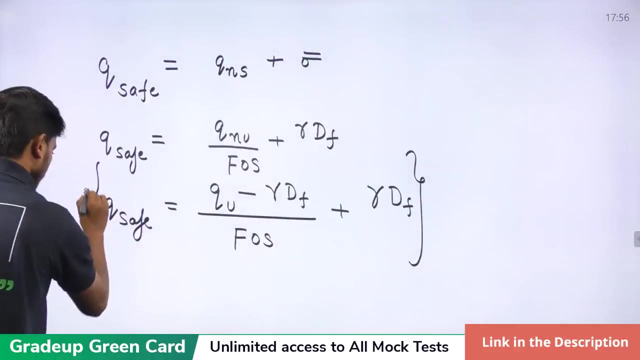 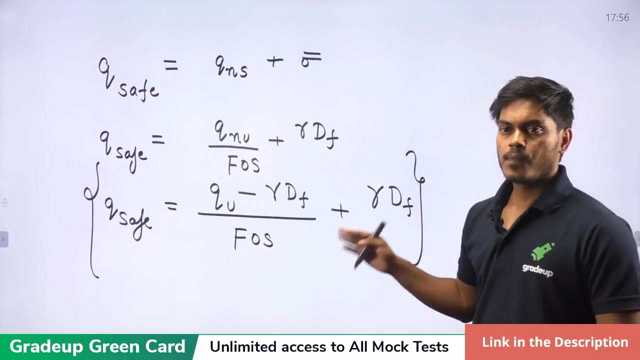 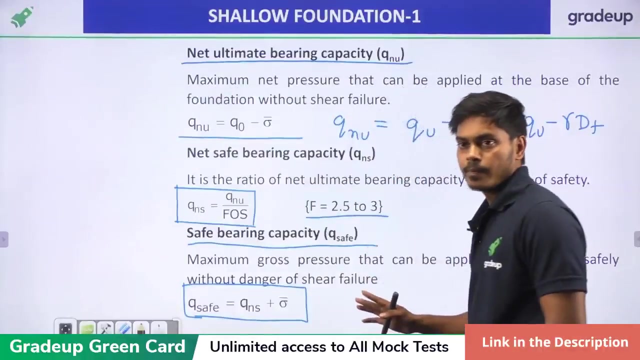 is Q and you. it is Q, you minus gamma DF divided by F OS. factor of safety plus gamma DF: all right if F, not. if F OS is not given, take this value from. take this value: 2.5 to 3. all right if it's not. 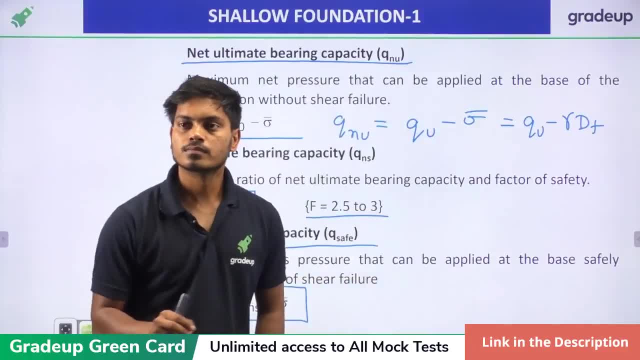 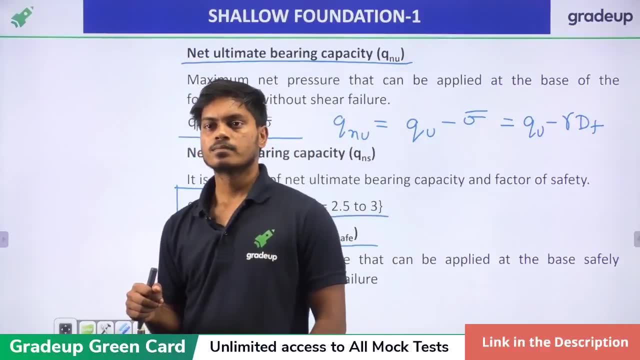 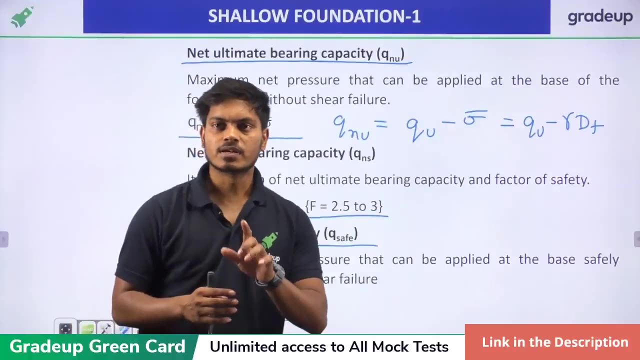 given: yes, I got it. yes, I got it. yes, I got it. yes, I am the right. it has to be deleted. calculation mistake: both of that. maximum question on a girl: current concept decreta. I'm just reading one comment. please just wait a series maya question. 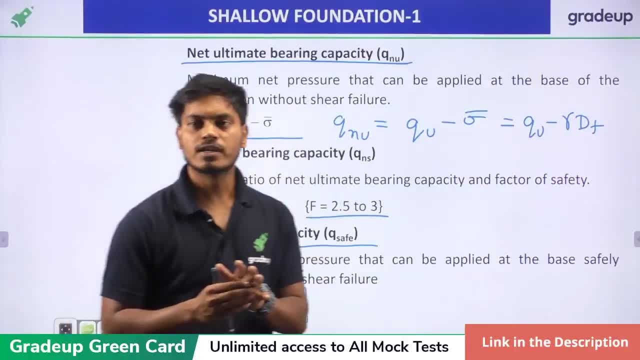 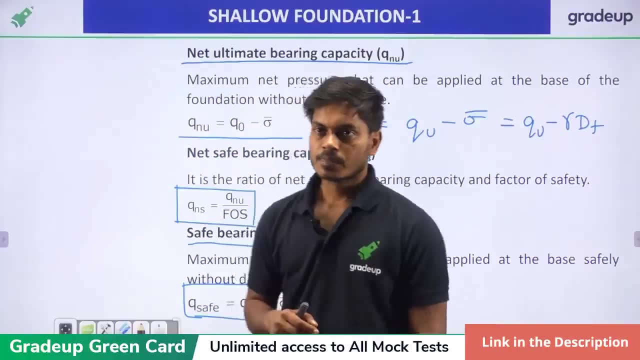 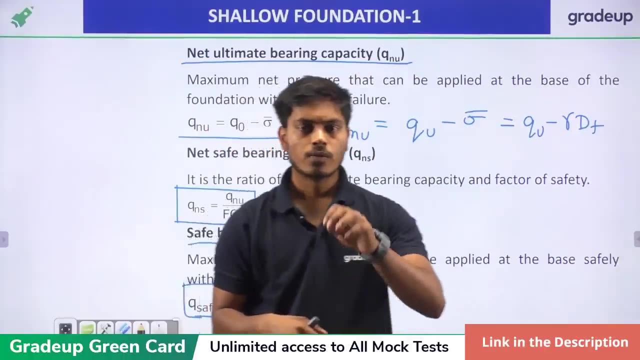 if this is the same problem you are facing. just listen this carefully: testes, make question 60 percent, talk who data? but calculation, mistake both at that. all right, see, there was this thing that me and my and my most of the friends they used to do is when we used to attempt the question paper. this is only 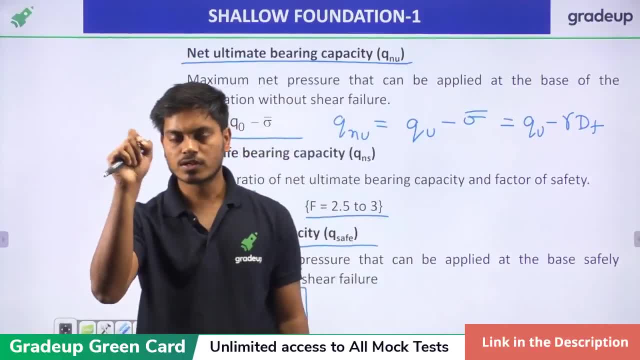 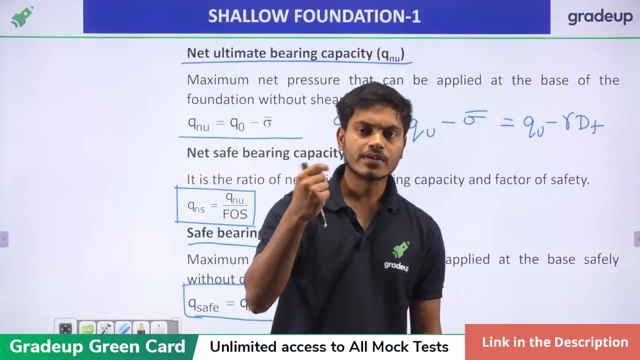 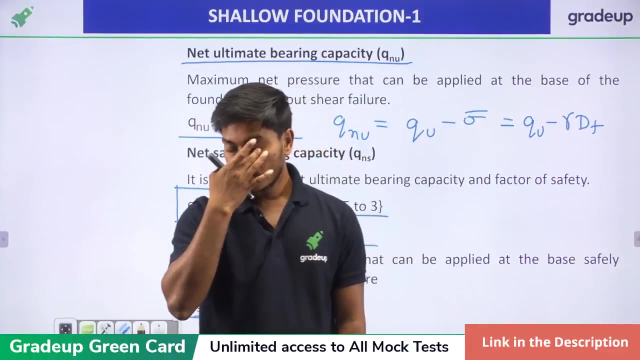 for gate ESC it's different because in ESC you have to fill the circles also, so the strategy completely changes in that condition. so for gate, when you are giving the test series, just go through the questions once. all right, just see if you know the question and like if you know the. 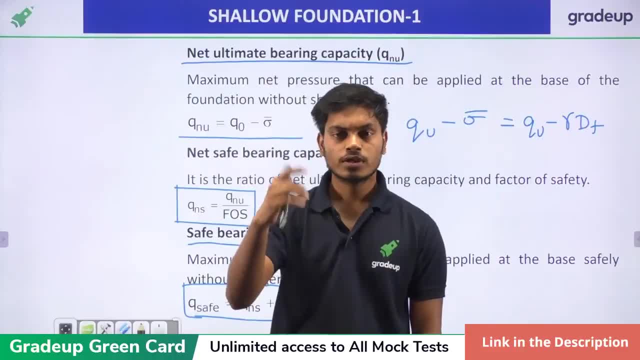 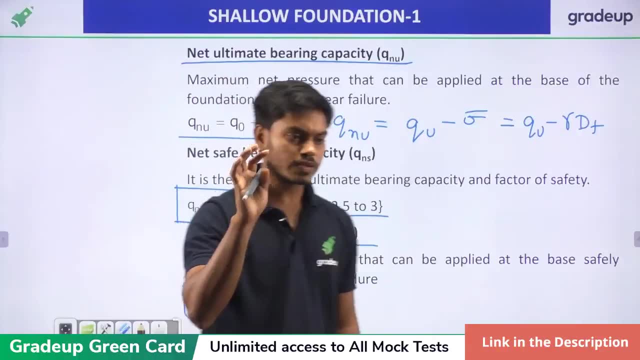 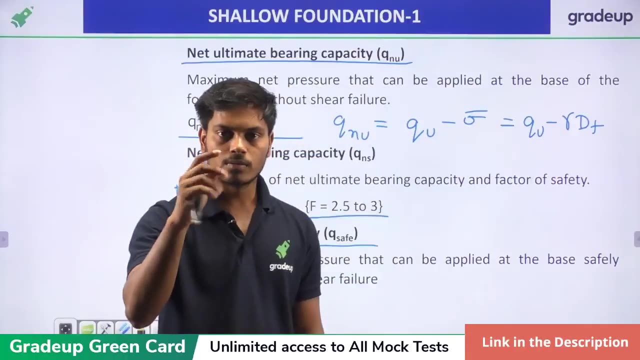 answer and you have feeling that, okay, this I can do, just solve it. just solve it, don't wait for anything, solve it. and if the question you are seeing and you think that it can take time, I know, but it can take time and I'm not sure about the answer, also just mark it. okay, just mark it. 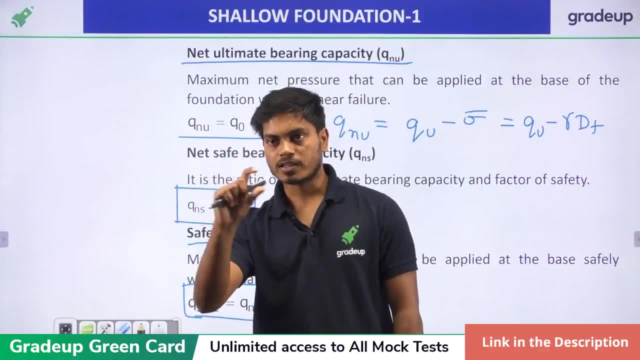 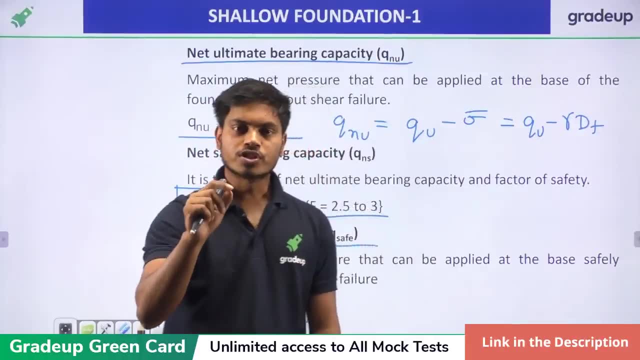 that purple thing will be there. there will be one option: mark the question. okay, so you're just, you just have to mark the question and move further, and there will be question which, after just looking at the at that particular question, you will be like this: I don't know. 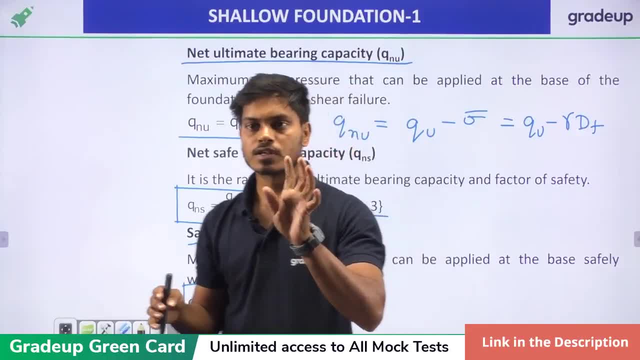 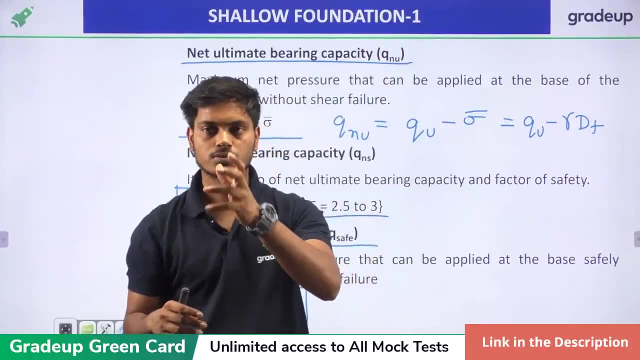 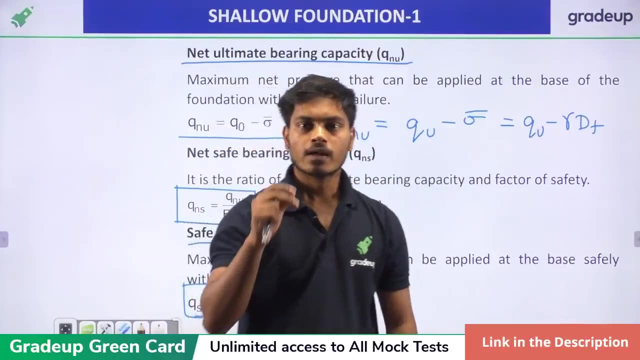 okay, this I don't know. uh, Hussain Sheikh, sir, reply please. okay, just after this I'll reply you. I'm really sorry. there are so many comments so I I know some of them are like I can't read, uh, every question. I'm really sorry for that. but yes, you can repeat the question, Hussain. so what you? 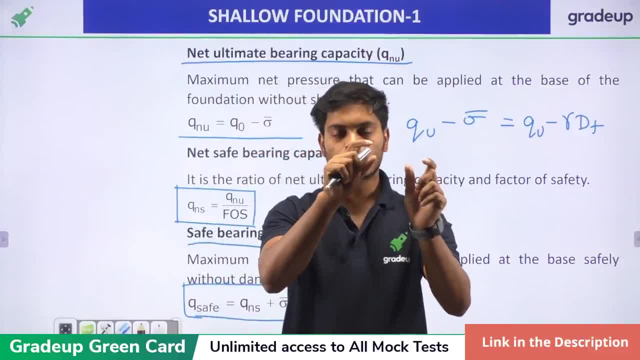 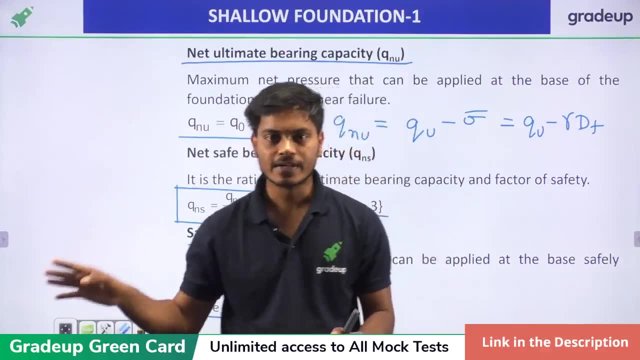 have to do is just go through the questions. as soon as you know that, okay, this I know, just solve it. if you have any doubt, just mark it. and if you know that I don't know this question, just leave it. so, in the end, just do it, uh, completely for whole paper, and it will take around, like your. 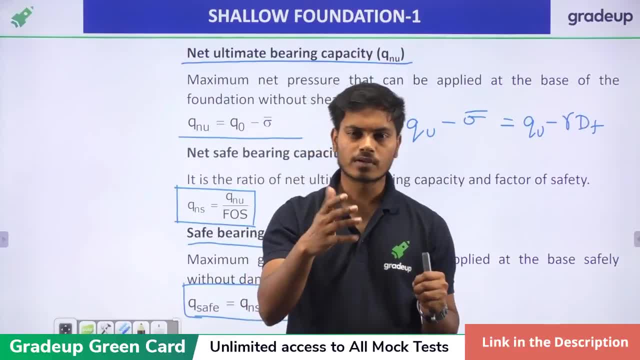 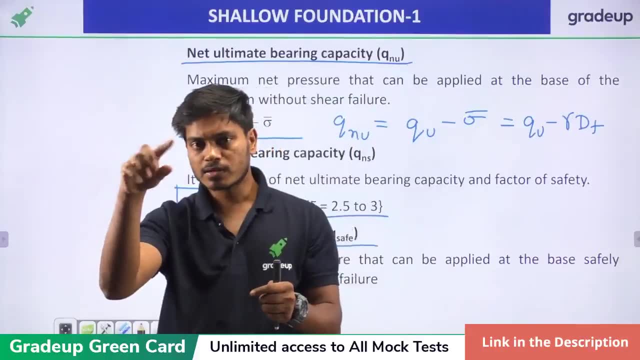 your paper will be done. this much paper will be done in around one and half hour. then look to the right side where the question number are written. you can easily see that. okay, purple are the ones which I have to solve. all right, then go to the purple ones where you can make mistakes, all right. 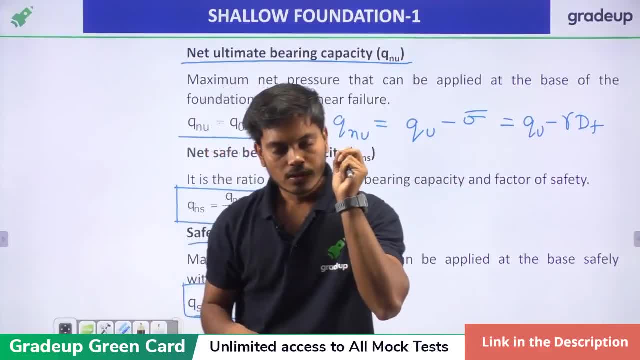 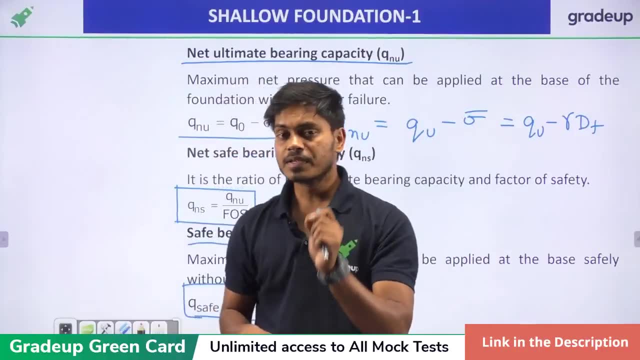 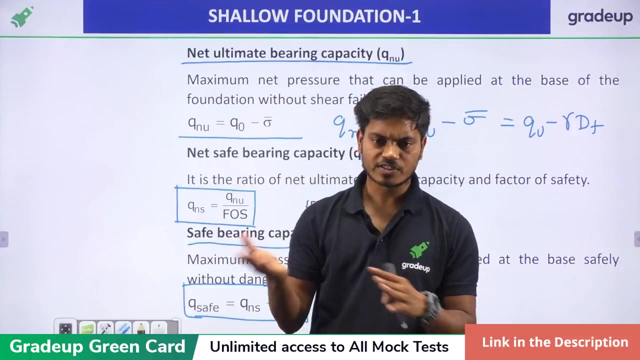 then solve those questions. and the last and the very important thing is you have to check every, each and every question. okay, there will be some question which will be very easy, suppose? uh, like, there is a question in which you have to distinguish between Westergaard and Bosignus. 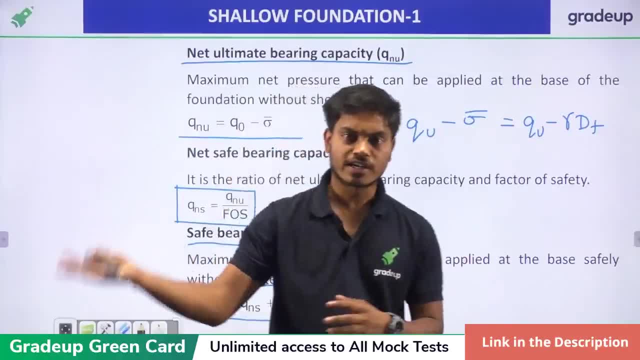 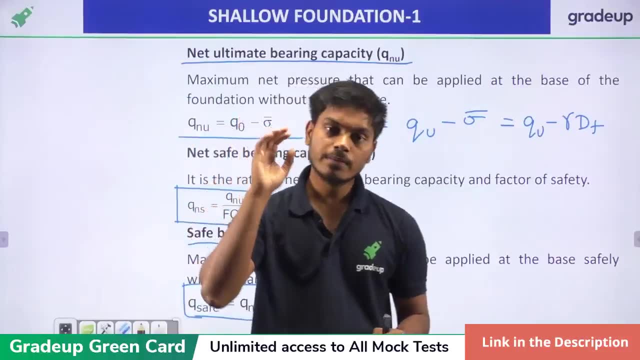 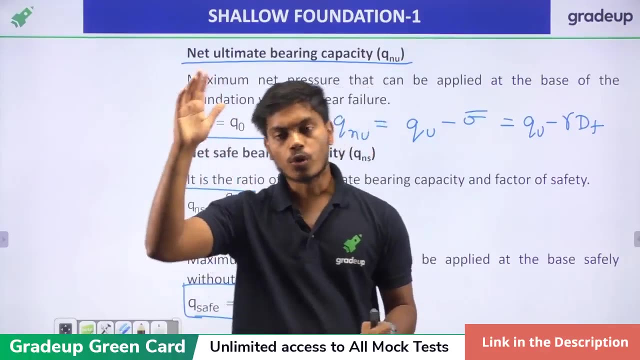 theory it is very easy. okay, one is stratified, one is for stratified soil, one is not for stratified soil. so you will be like, okay, it is easy, I'll do it, but you can make mistake in those type of questions also. so do not just answer the question and leave them. go back to them in the end of the 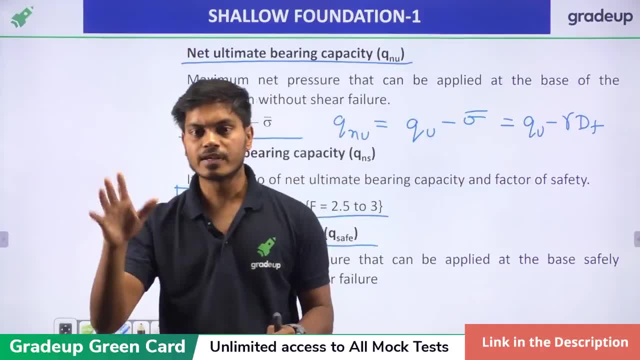 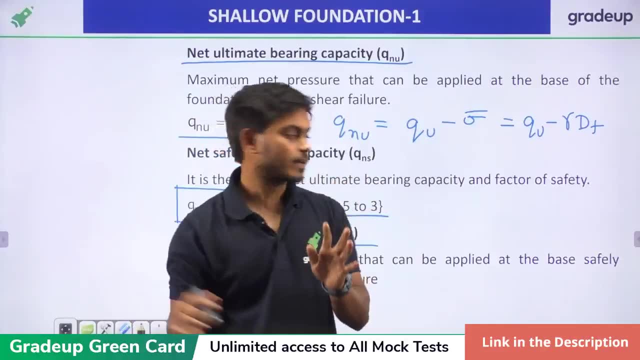 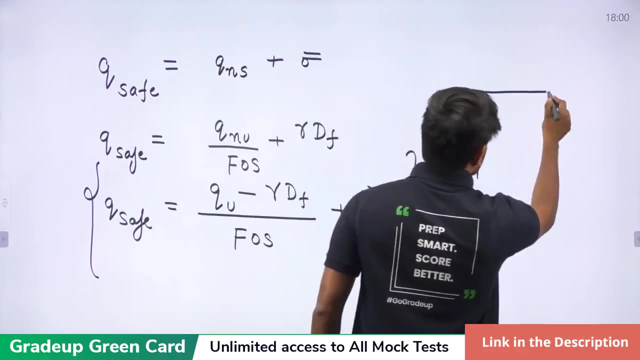 uh, like you have solved all the question, go back and check each and every question. wherever you are doing the rough calculation, please bifurcate it by other suppose. this is the suppose. this is your question. uh, this is your scribble pad. okay, so if you are doing question number one calculation, just do it. whatever you need to do. 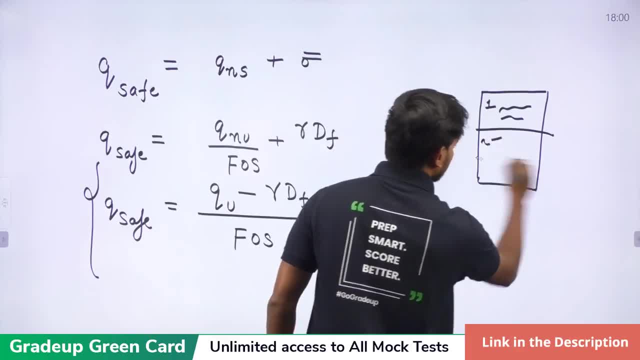 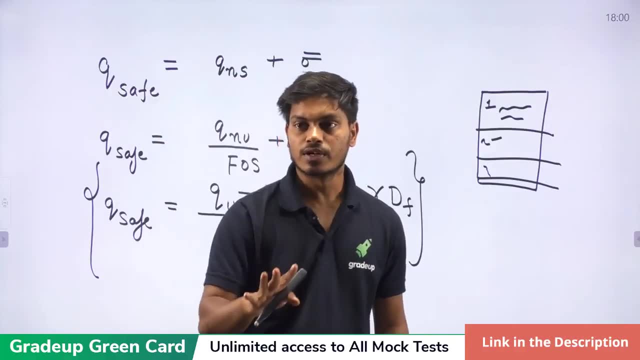 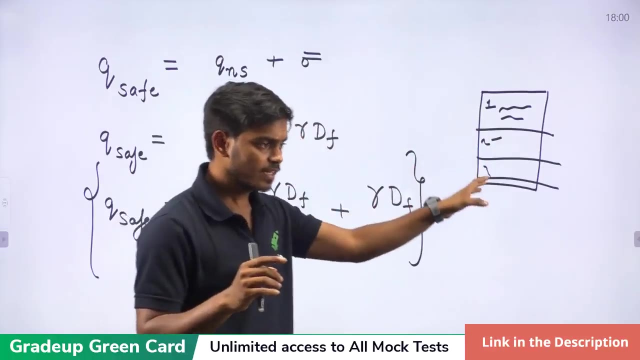 the calculation is there. bifurcate the page, then go for second: bifurcate the page. third, bifurcate the page, so you just have to check your calculations. okay, in the end you just have to check the calculations, all right. so please do this, do not, uh, think that. okay once i have done it. so it is. 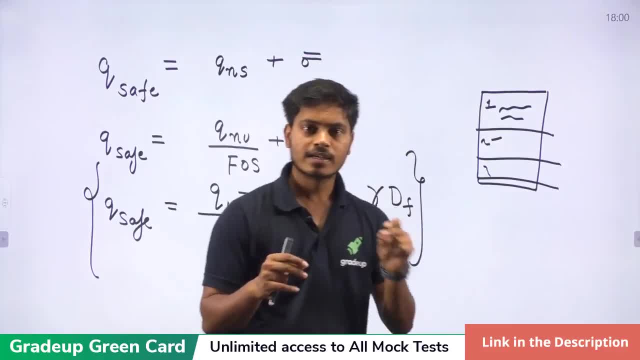 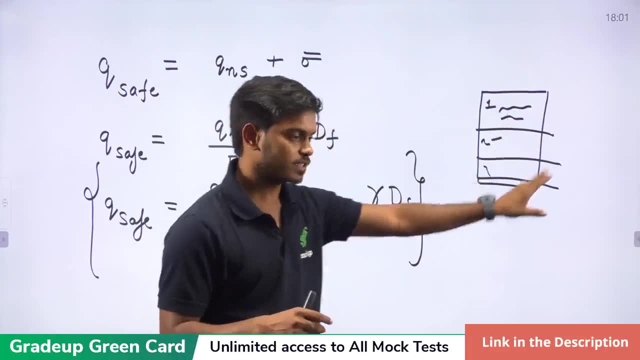 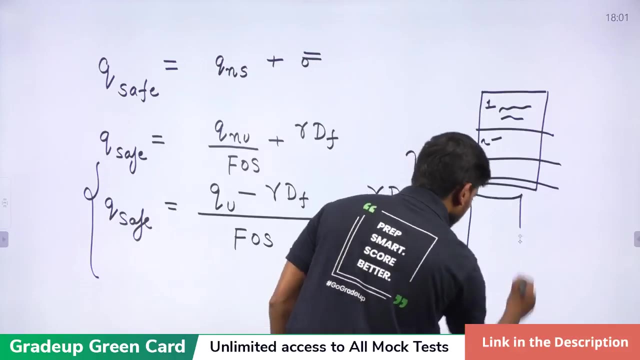 correct. okay, most of the mistakes will be cleared or, uh, recorrected in that checking of yours in the end of the question, in the end of this test. all right, so do not hodgepodge it suppose, uh, some people what they do is first, question solving- okay. second, they are solving here. third solving- 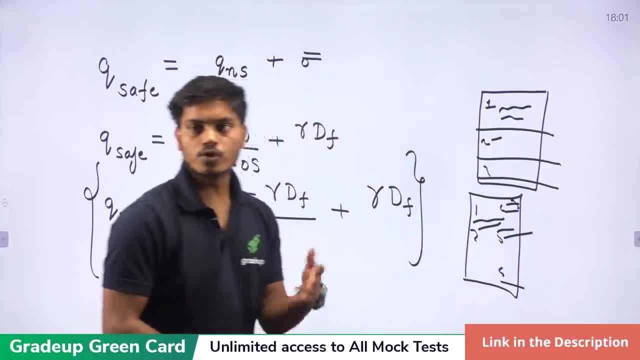 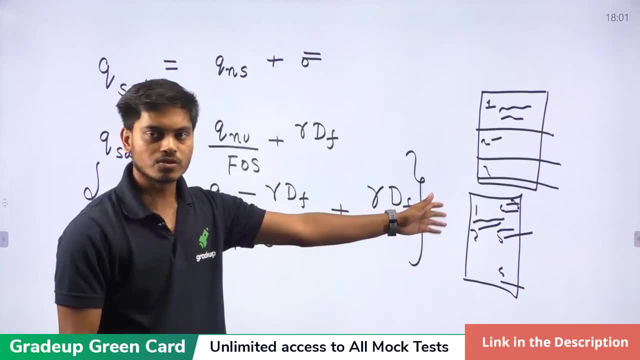 here. four, they are solving here. fifth, they are solving here. so, like, if you want to check the calculations, how can you do the? how can you check the calculation in this condition? okay, so you have to take care of these things when you are giving the giving the paper. 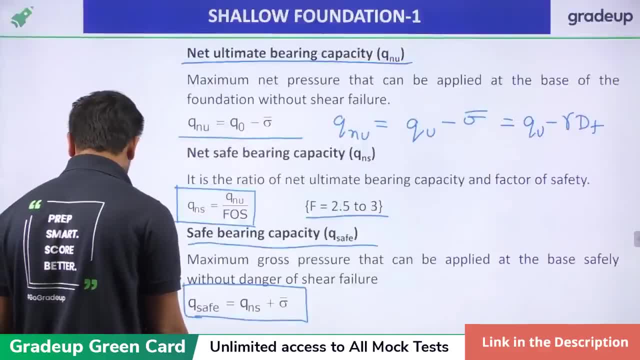 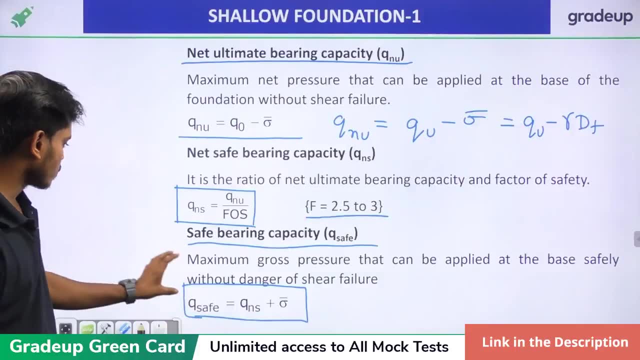 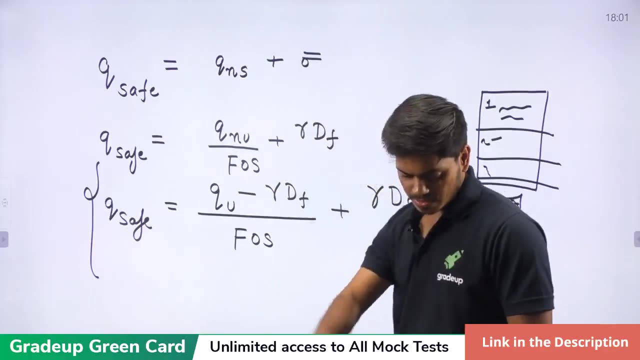 okay, all right, husseini, just please ask your question. what? what is there which i missed, i think? okay, till he is writing. uh, let me just recap all these things. okay, so, safe bearing capacity. we were calculating and this is how we can do that. q save is qu this and this is this. it is written over. 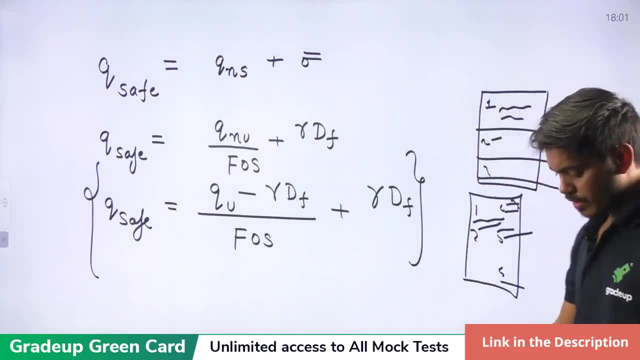 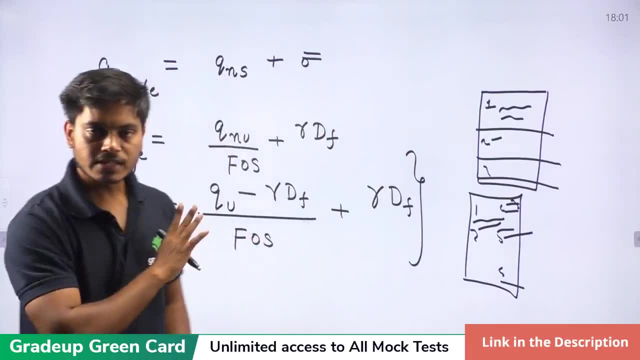 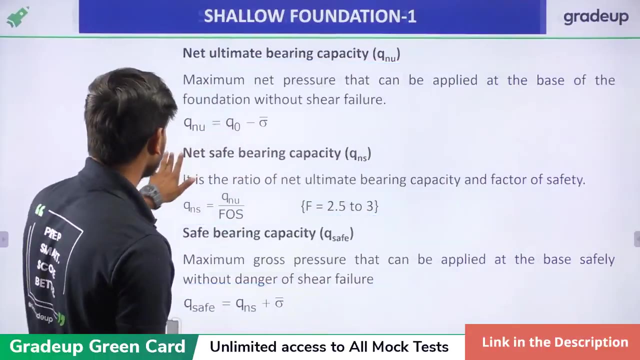 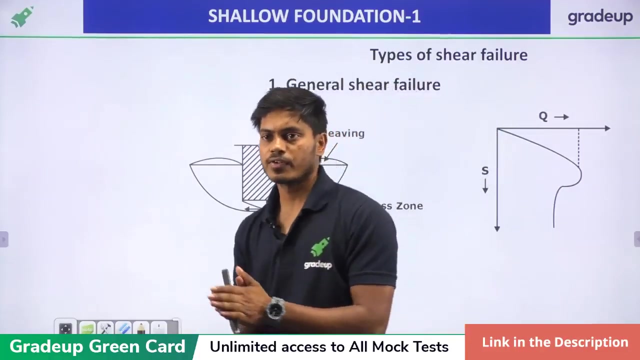 there you can see. so the safe load of the foundation is nothing but safe bearing capacity into area of foundation. all right, this is how you can get the value of your, your safe bearing capacity. now we have to see type of sheer failures. okay, this is why i was saying that we are going to discuss the failures. 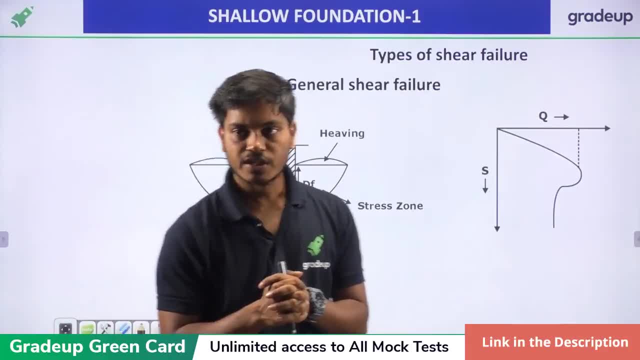 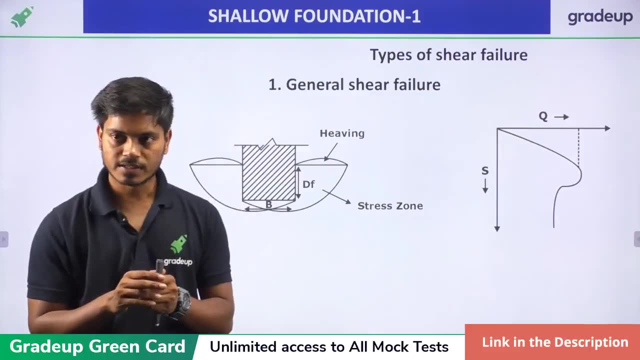 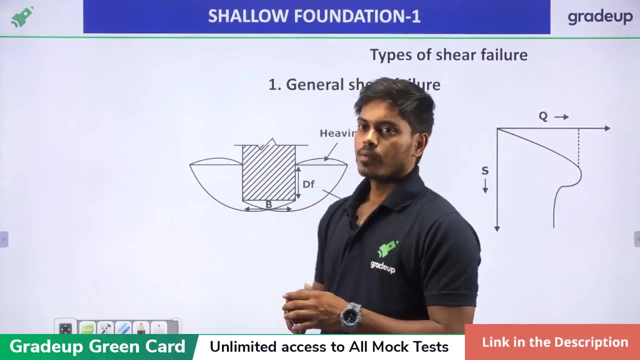 each one of them. so types of sheer failures are there, hi muthun. uh, sir, please discuss some numerical regarding the topic i. i will. i will discuss it. uh, who asked abhinash? okay, just give me some time, have some patience. all right, i'm trying to give you the best question out of every uh previous year question paper. okay there. 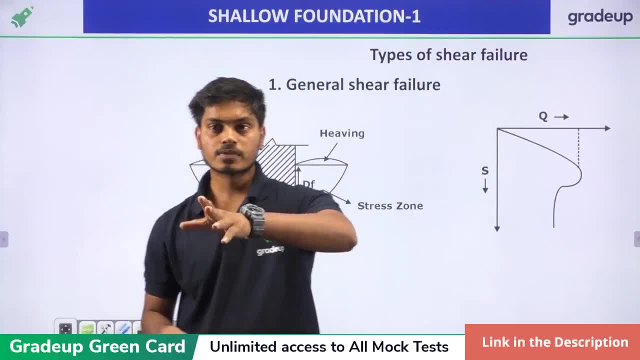 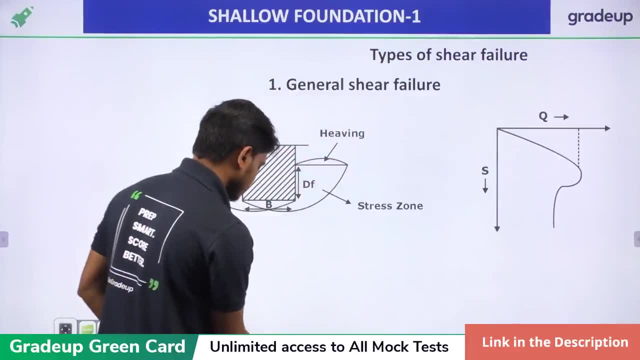 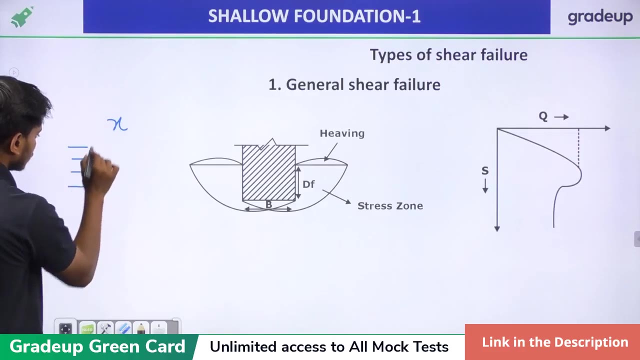 is one more thing there. one more thing what, like some, some uh students have asked me a doubt regarding this thing. see, uh, there is a topic x. there is a topic, suppose x and the coaches regarding x are coming continuously in 2011, 2012, 13, many ayah. 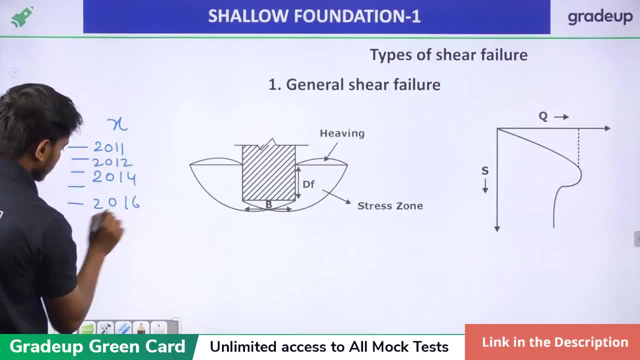 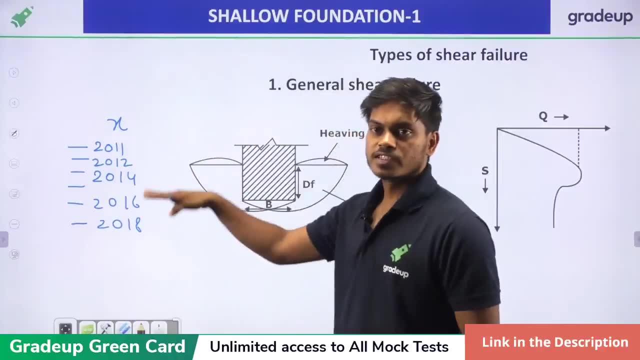 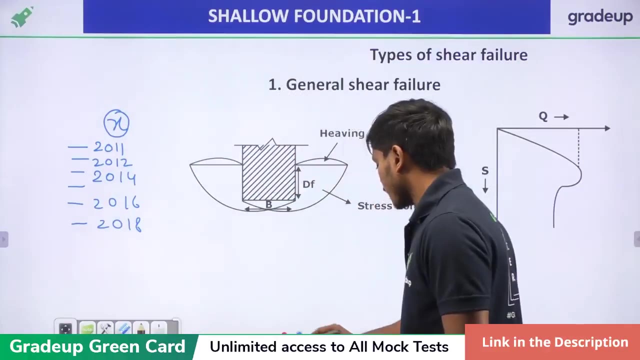 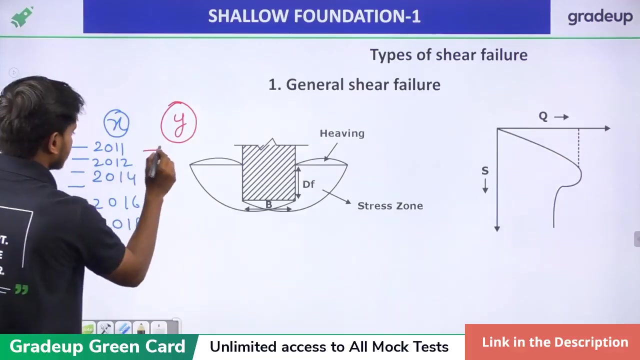 2014, 2016 and 2018. this is the pattern of the topic. hello, Rakesh, this is the pattern. all right that the questions regarding X are coming in the question paper. now there is another concept, which is why and the question regarding why are coming like this. there was no question in 11, 12, 13. 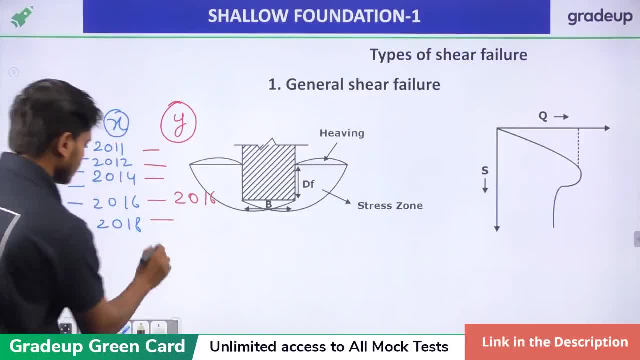 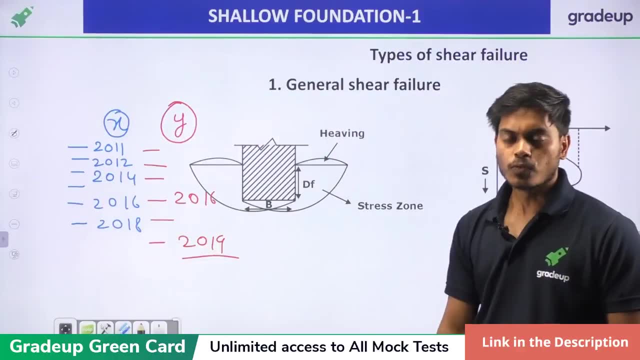 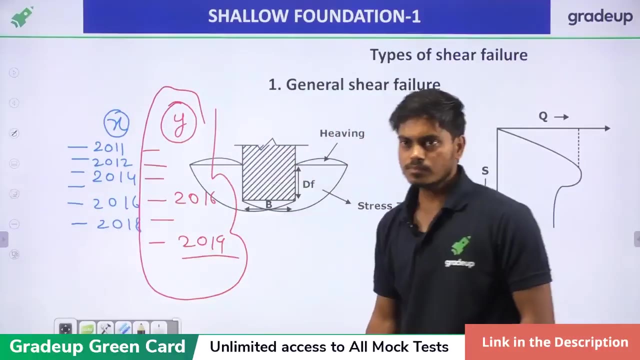 yeah, there was question in 16, no question in 18 and suddenly in 19 again they are asked. they are asking the same question or the question regarding this topic, so what they will do is what? what student have asked me said: this is important and please focus on these thing. I have a request from you people. 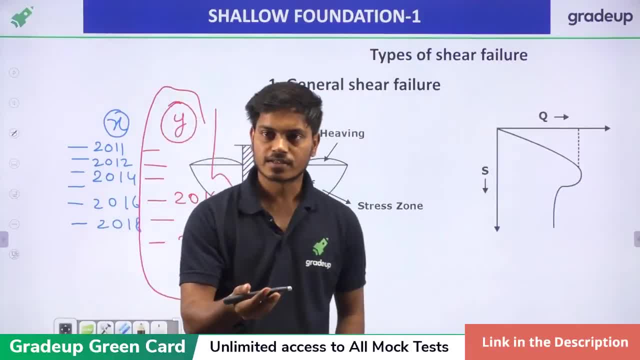 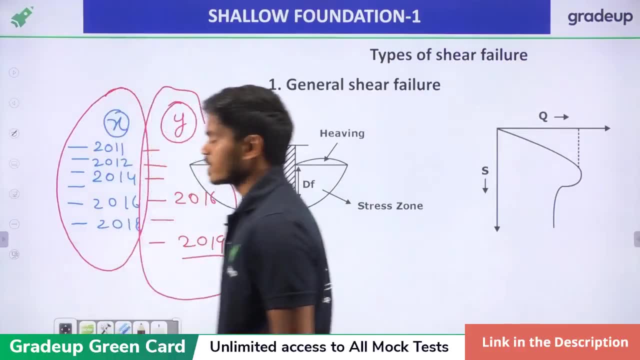 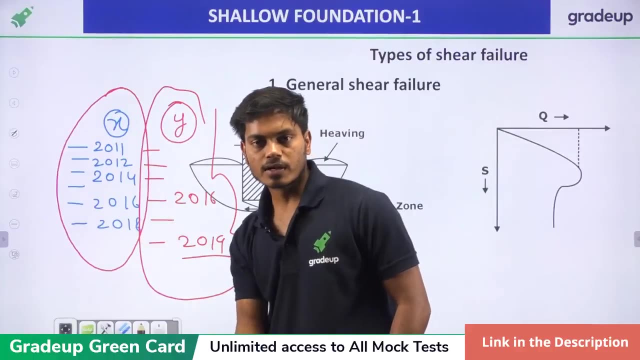 that this is not the case. okay, this is not the case here. you have to focus here first the things which are coming continuously, as you can see the pattern, they are coming continuously. but where you are do like what you can say: focusing, you are focusing on a topic. 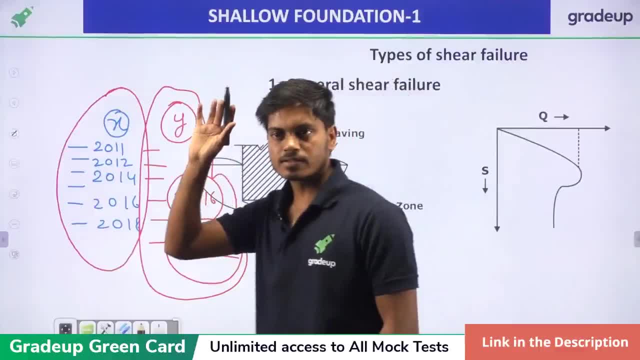 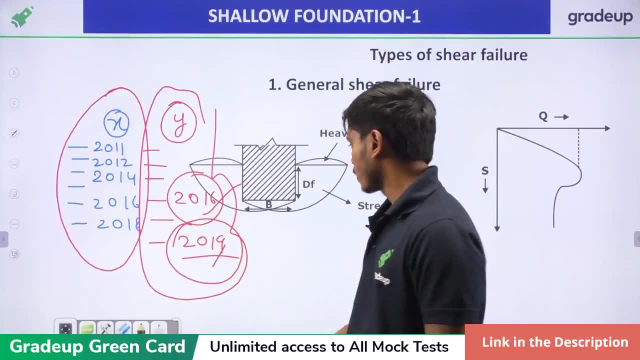 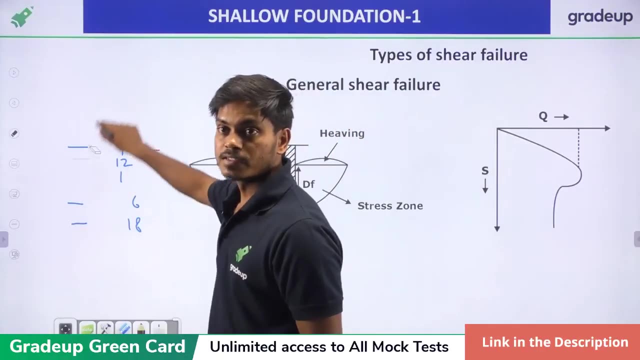 which is coming only, like from 90s. okay, from 90s it has come only in 2016 and 2019, so this doesn't make it important. all right, sorry, I have made this thing here only. let me take some comment in. essentially, this is the question, which is why are you asking me this question? 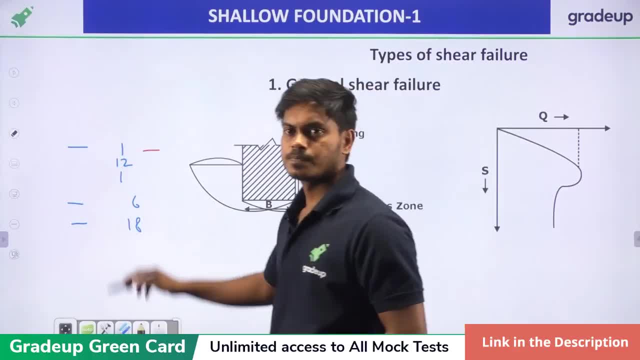 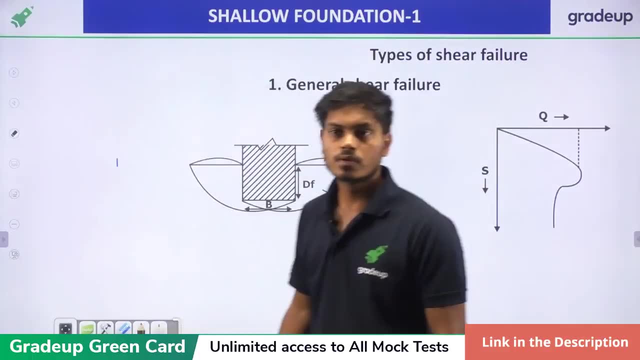 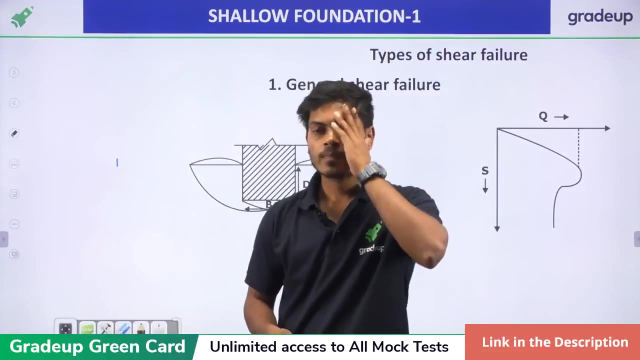 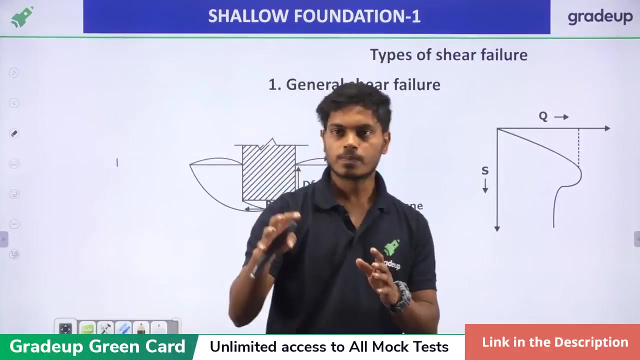 I have taken from you. it's a question about the socio technical or not. in terms of socio technology, is it easy or not okay? so actually, these things, I don't know if you, your people, don't know that I'm dealing with two type of comments. one is coming from our 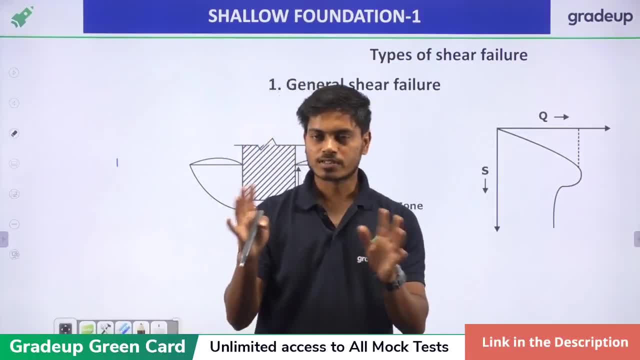 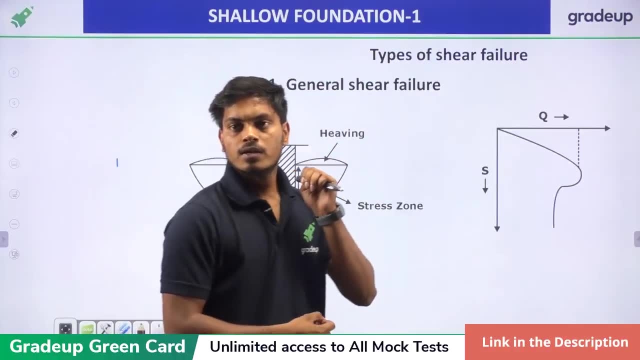 GridUp ad and the other one which I've put together at Understanding 1995, which app and another are from youtube, so i have to just focus on both of them. so just please be patient. all right, i'll going to answer each one of you compared to, so this geotechnical is easy there. 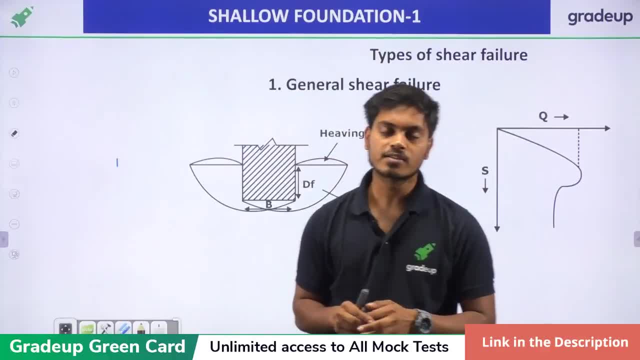 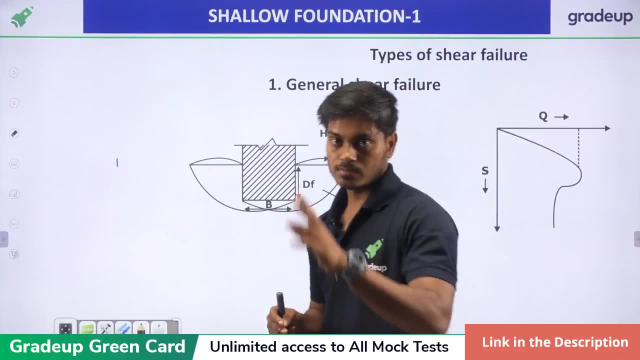 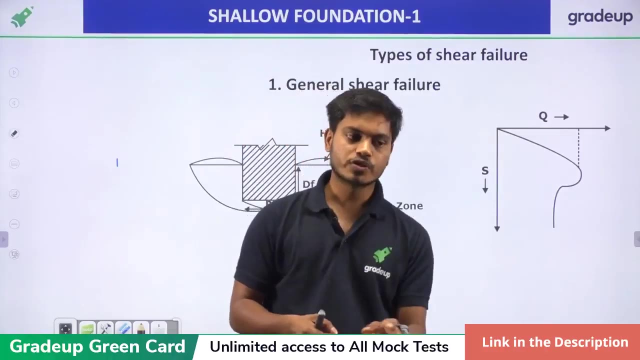 is no comparison between both of them. one is completely numerical based. second is completely based on theoretical portion. all right, but yes, these, both, these, both subjects. fortunately, both the subjects are that type of subjects. if you will understand the concept, then there will be no question in the previous year question that you won't be able to solve. all right, yes, just. 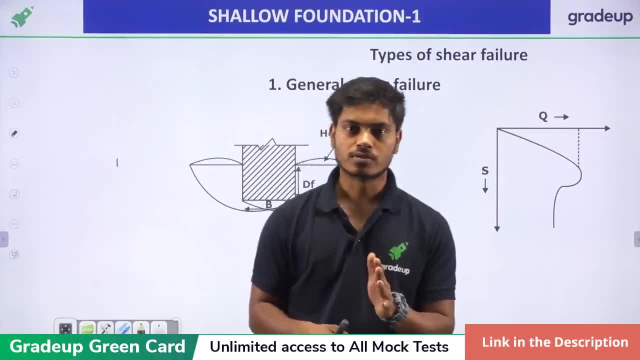 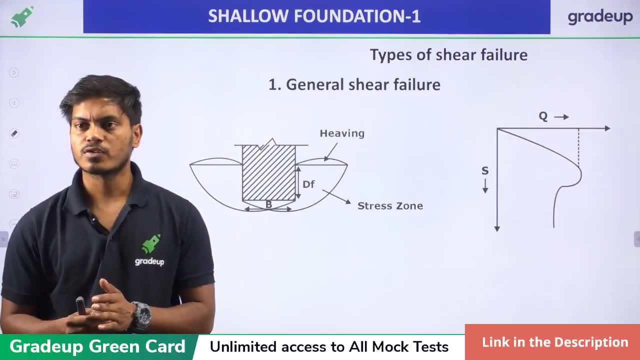 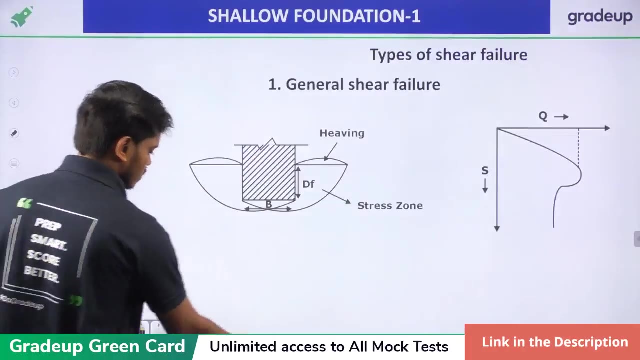 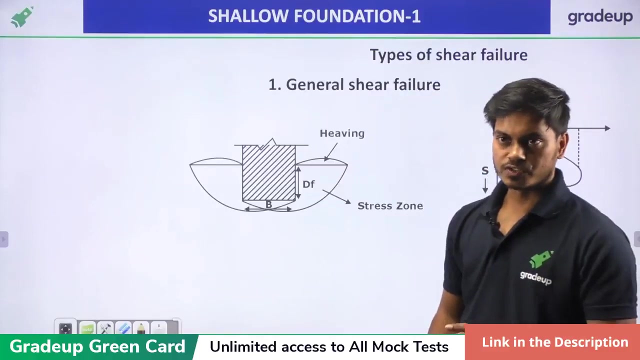 just geotechnical. take some time because it has this theoretical portion. okay. deep foundation, kashan foundation. deep foundation, fair, shallow foundation. what's the what's the question here? rakesh, you write the question, i'm telling you what is shear failure? all right, so this shear failure, it occur in shallow foundations, okay. 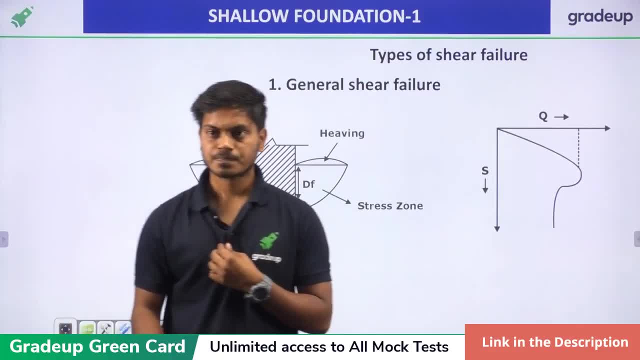 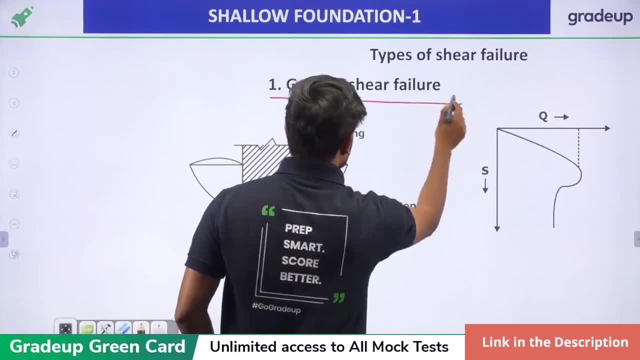 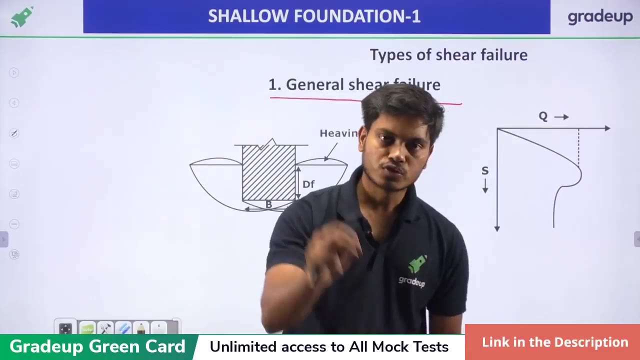 it occurs in shallow foundations. so now for shear failure. we are talking here. so this shear failure occur in case of shallow foundation first, and what happens here is if the soil is medium to dense, then only this will happen. so this is important point. please note these down. 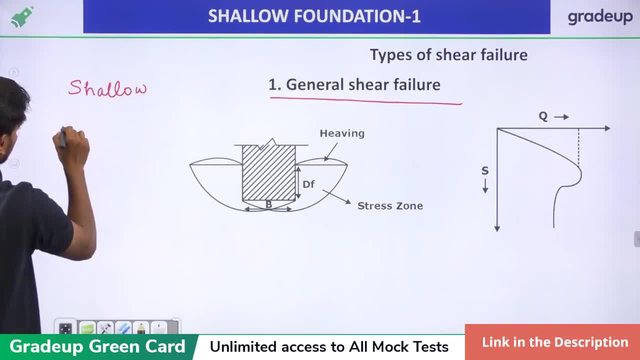 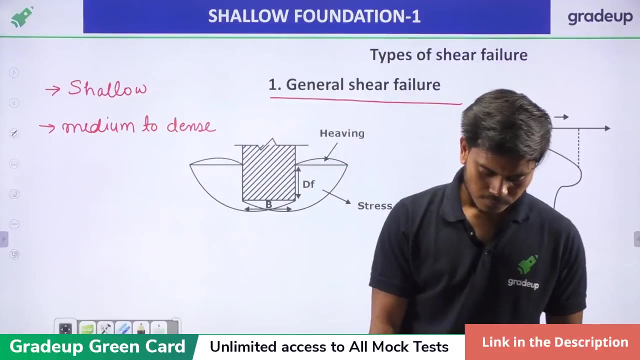 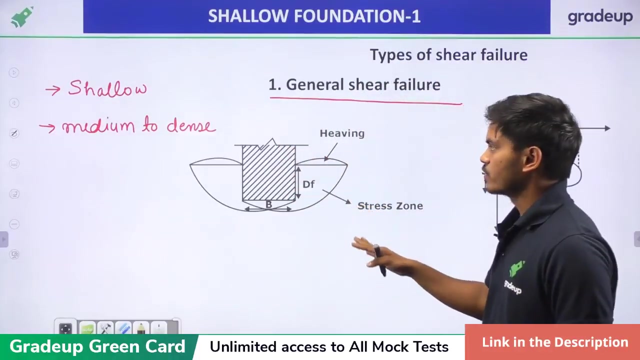 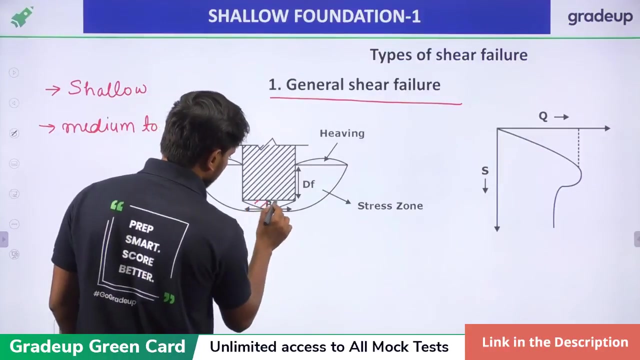 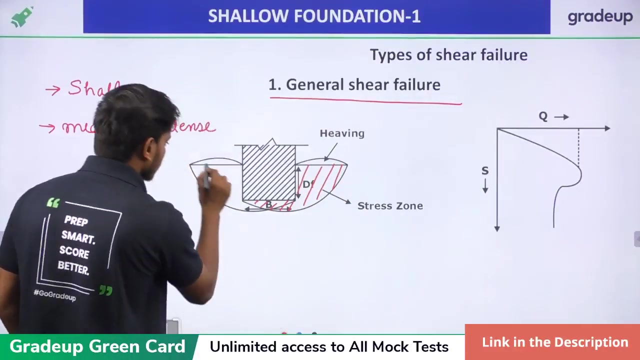 first is: foundation is shallow. soil type is medium to dense soil type is medium to dense. okay, the settlement because of the general shear failure will be negligible. all right, will be negligible, but this, this is the stress zone. actually, this thing, this is the stress zone. there will be some heaving also around the 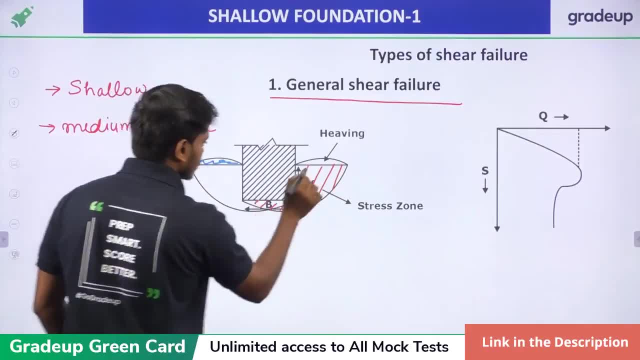 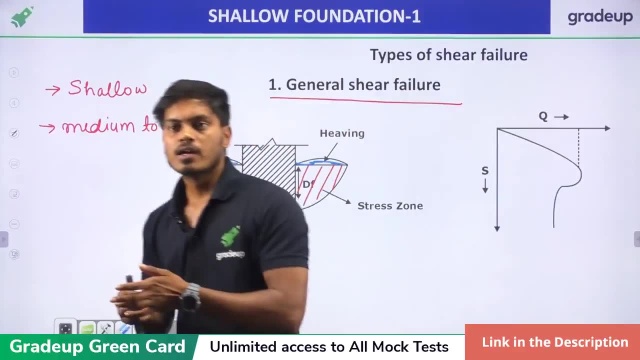 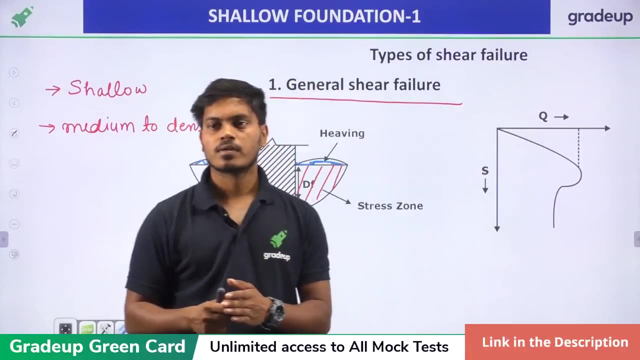 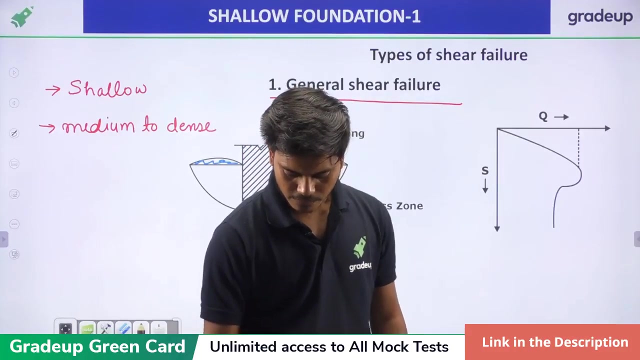 foundation. this is the heaving. heaving is nothing, but in hindi you can say: okay, it happened in gate. no, shilpa, this won't happen in gate. okay, all right, this won't happen in gate. they won't give you the previous question paper, but, yes, there will be a case when topic will be repeated, all right. 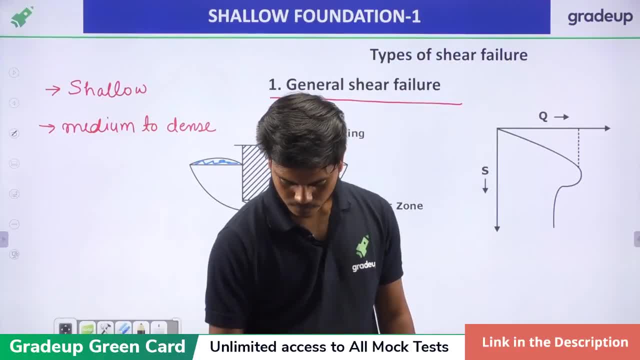 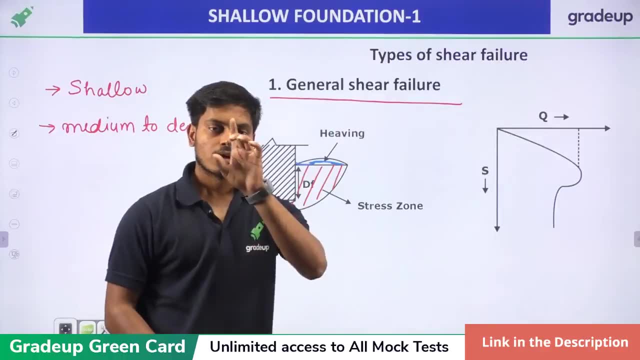 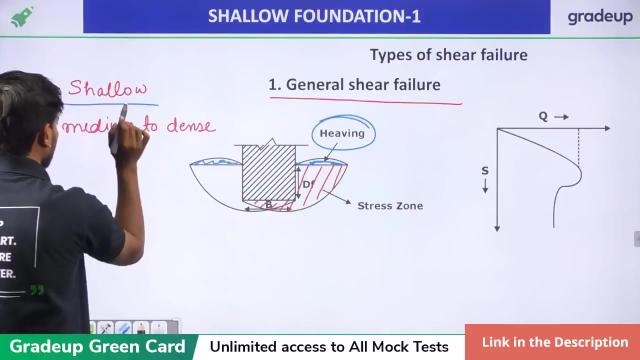 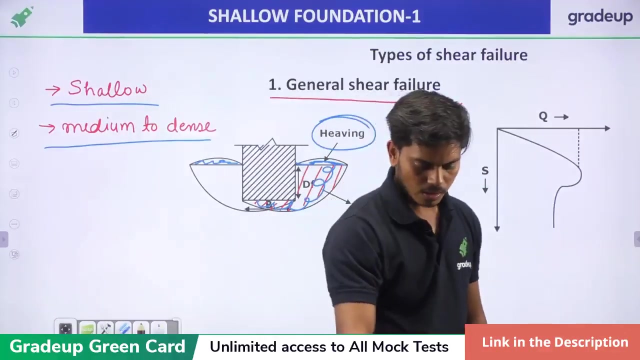 where topic will be repeated. all right, so there will be some heaving in case of general shear failure. okay, these are some points that you have to take. uh, take care of these points. heaving is there. happens in shallow foundation, medium to dense stress zone. comes till the ground surface, all right up to ground level. you can say: 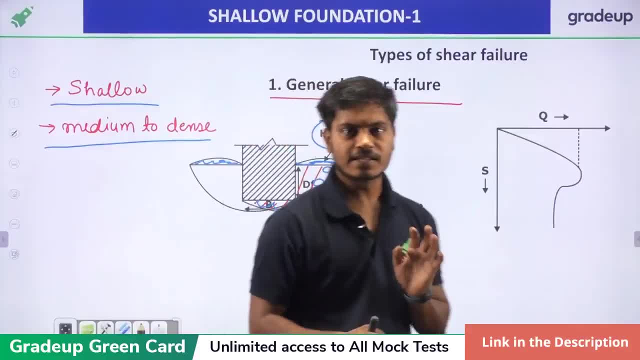 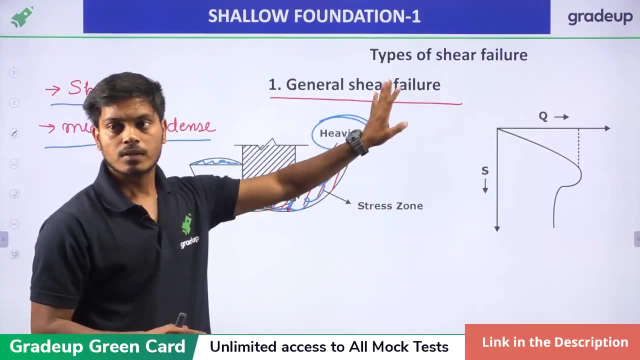 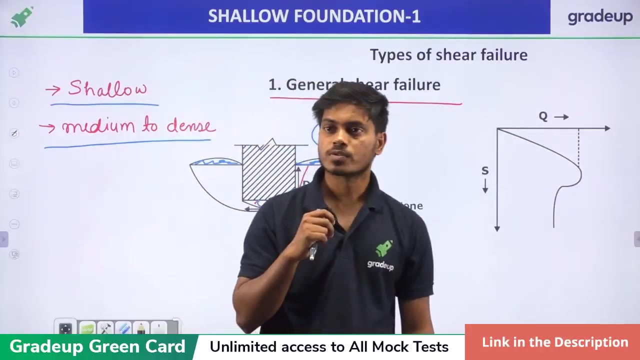 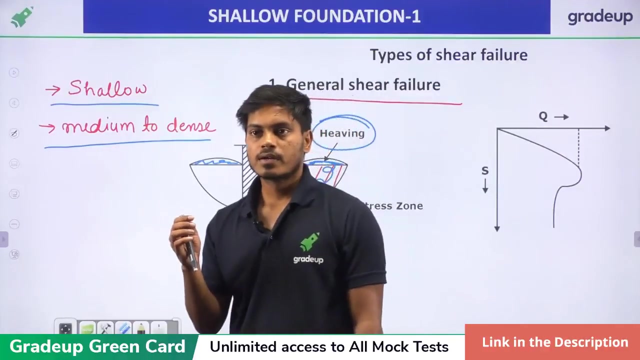 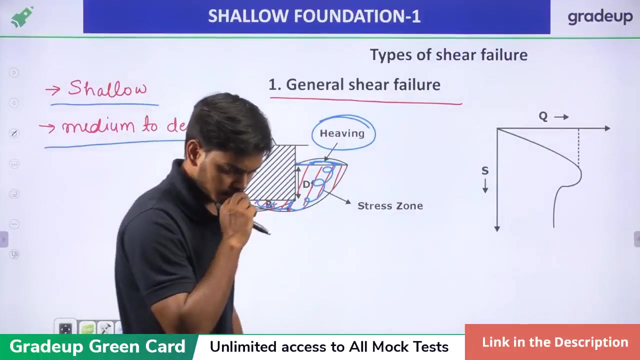 so if we make the graph of load by settlement, if we make the graph load by settlement for this, okay, saturated unit weight or submerged unit weight, cup question may use: uh, actually, this is a very question, specific doubt. all right, it is punching failure. what is punching failure? hardship? i think this is uh shear failure. only, according to me, this is general shear failure. 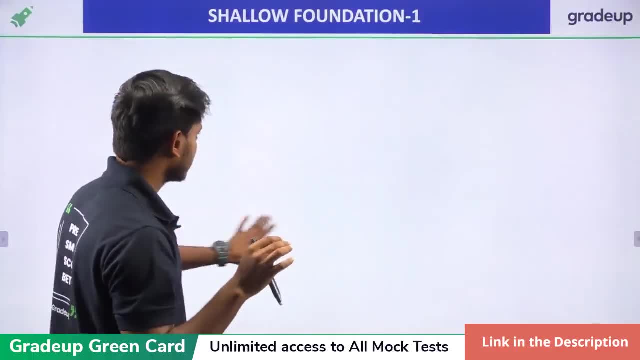 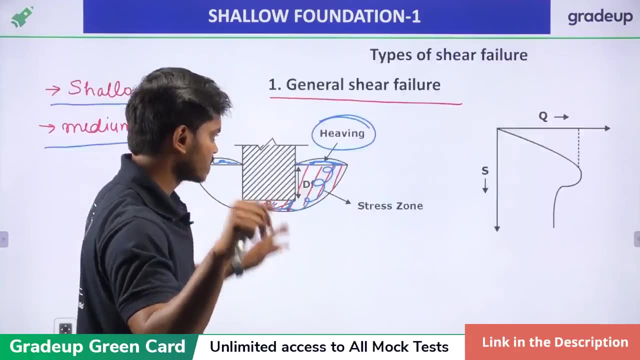 and you can rely on this information, because we have a complete different diagram for this local shear failure. and then there is your punching shear failure. so, okay, you can rely what i'm telling you here. so, general shear failure, heaving, is there these things? stress zone and all. 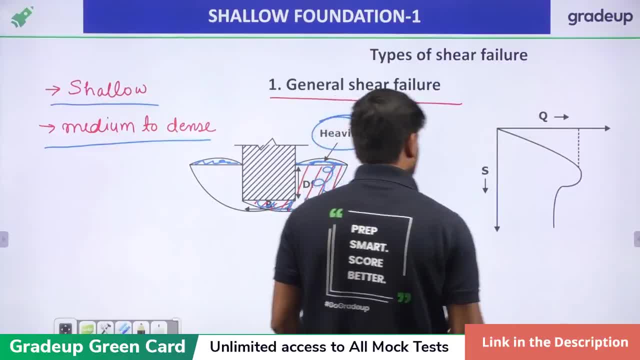 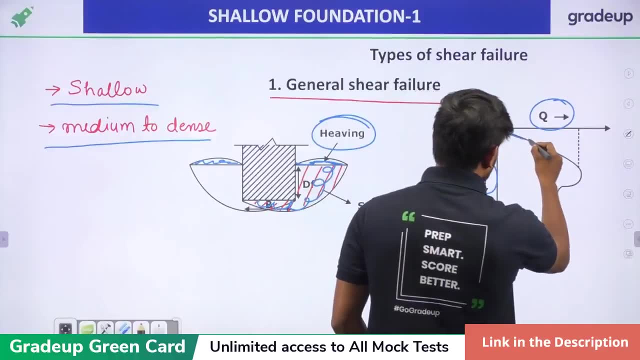 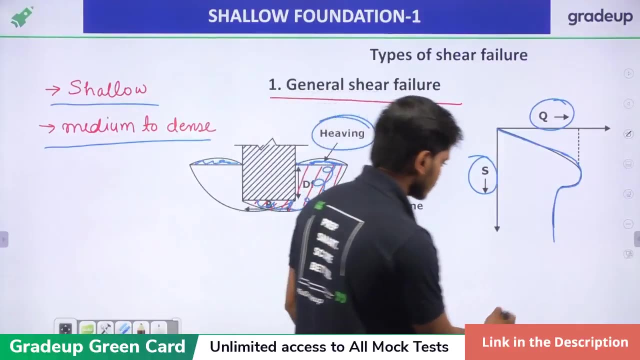 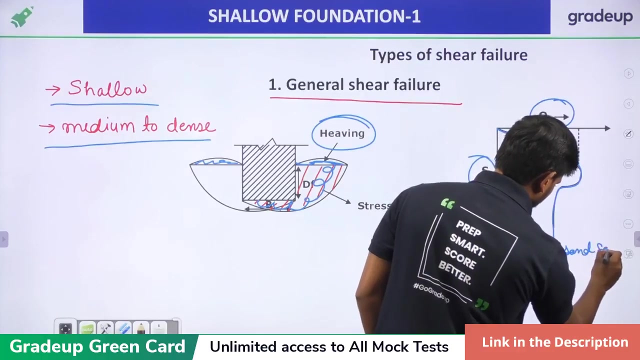 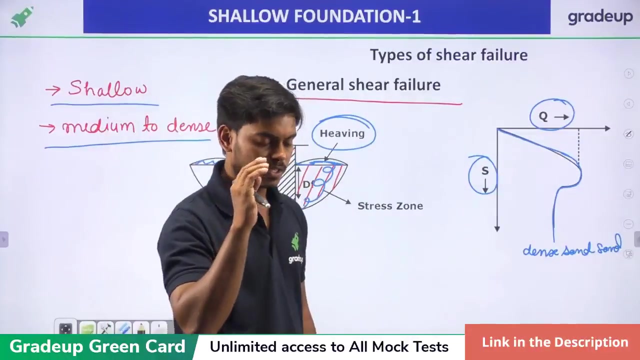 so there is this graph. this graph is there. it is between the load and the settlement, all right, so this is how it will follow. it will go and add, but at one position the settlement will occur. okay, so this graph is for, uh, dense sand, dense sand and over consolidated clay. also, as i have told you, in the uh in, in which, uh, yes, in consolidation. 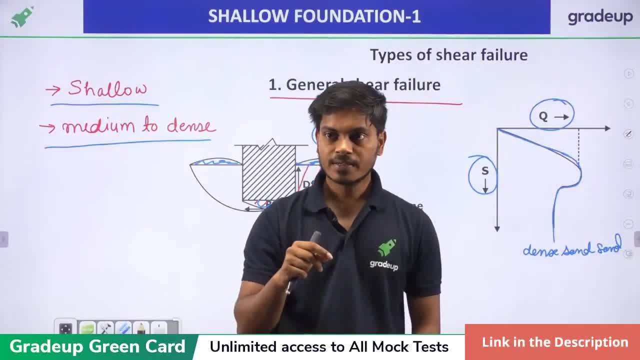 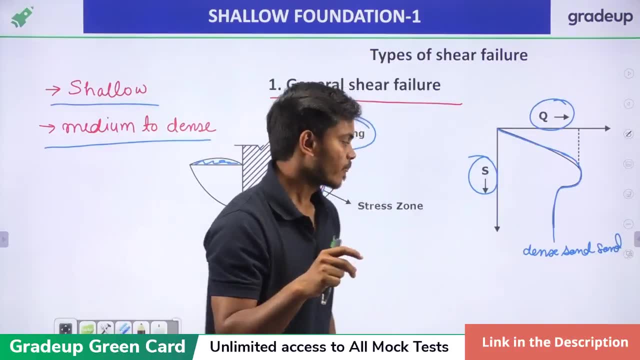 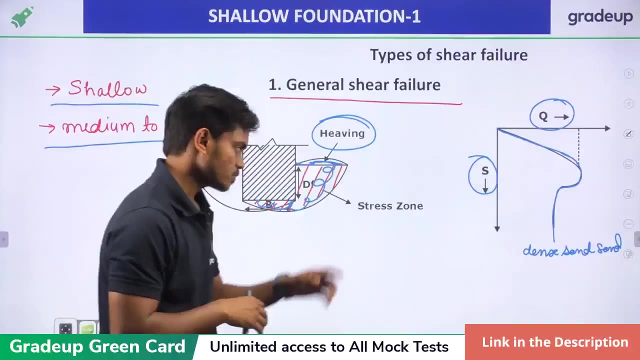 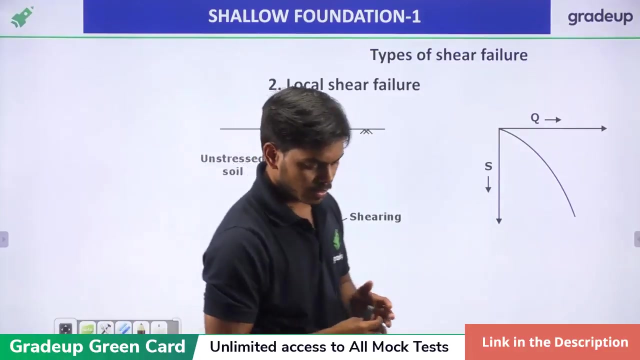 chapter. that the over consolidated clay behaves like a angle between two net is easy. it is in punching failure, right? actually, uh, the over consolidated clay acts like dense sand, only all right. so this is the graph for, uh, general shear failure. next thing that we have is local shear failure. so, um, the previous one, the general shear failure. 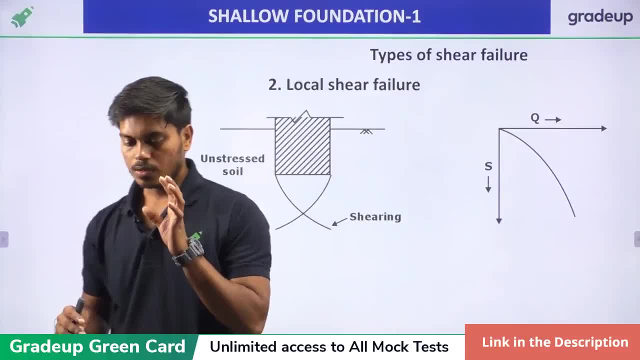 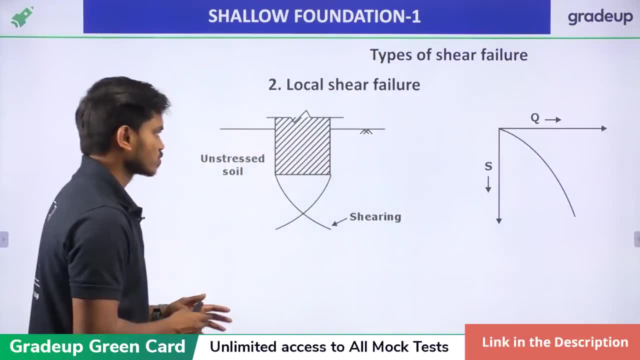 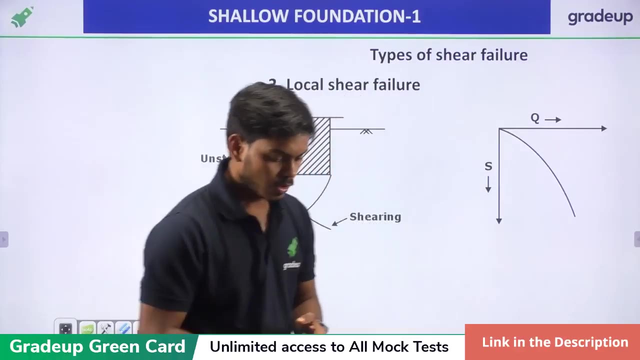 it was happening in a medium to dense end. but if the sand is loose, if the uh sand is loose or it is a soft clay, then in that case local shear failure will occur. okay, local shear failure will be there. it is different from general shear failure. there can be local shear failure which is being quarried on powder hand sand. 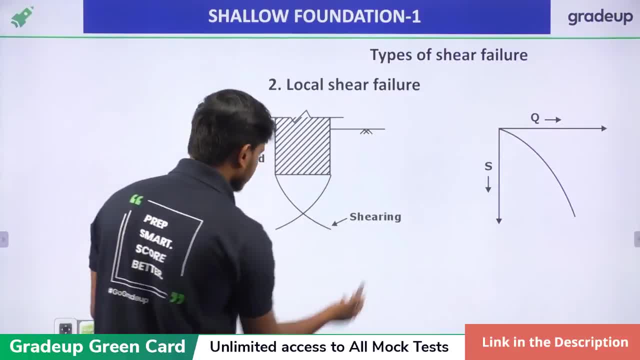 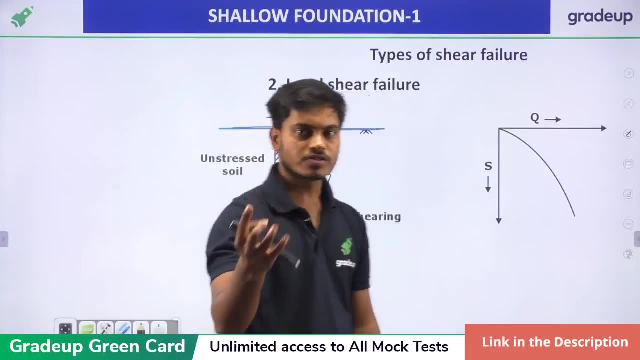 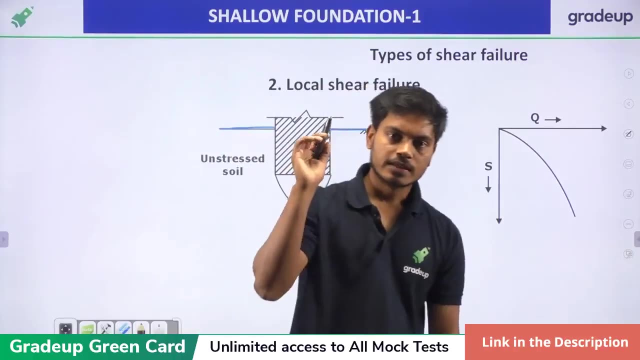 from general shear failure how? first thing is, there is no heaving in this case because the soil is soft, so it will just take all the stresses in itself. that's why the stress zone will not reach up to the ground level. okay, the stress zone will not reach up to the ground level. this is the second point. 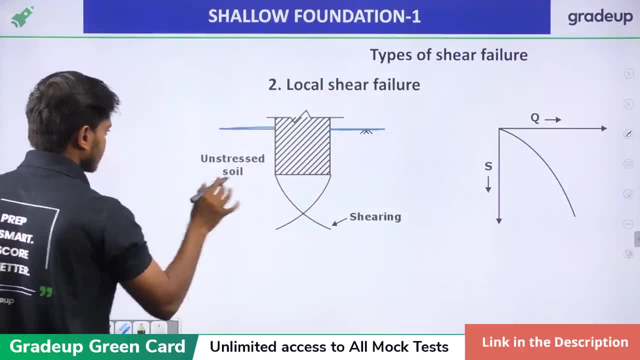 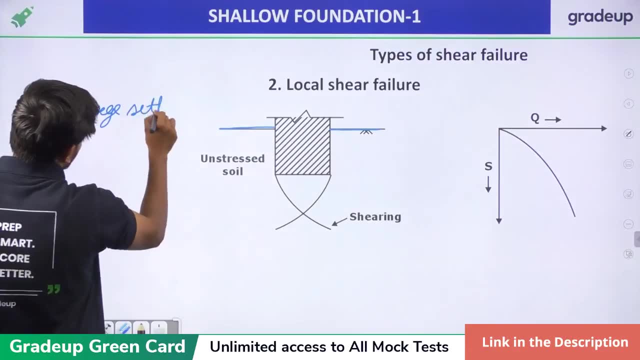 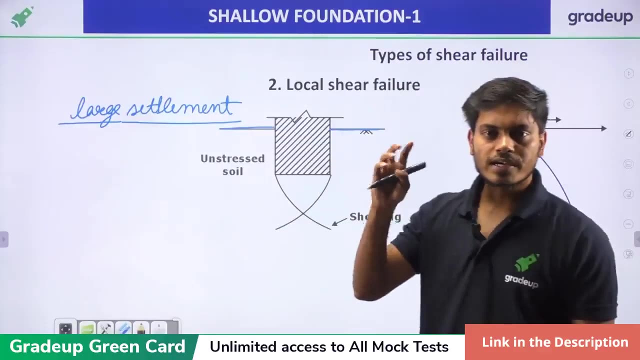 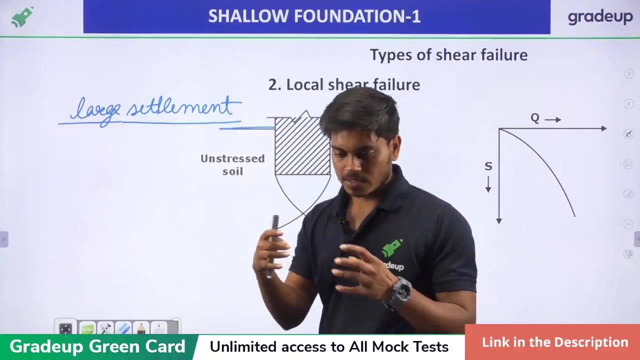 regarding this. but there will be large elastic settlements. there will be large settlements you can say, but in case of general shear failure, there was a negligible settlement. okay, as you can think or imagine by the name also, that the soil is soft. you can say: and like the clay, soft clay or loose sand. they 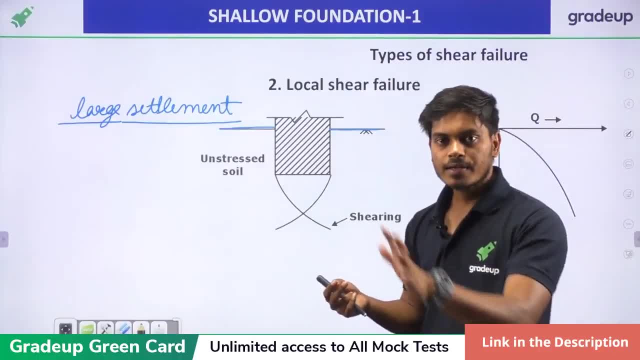 are very loose, so that's why the settlement will be high in comparison to the general shear failure. but no hearing is there, or the soil is soft, so that's why the settlement will be high in comparison to the general shear failure, but no heaving is there, or 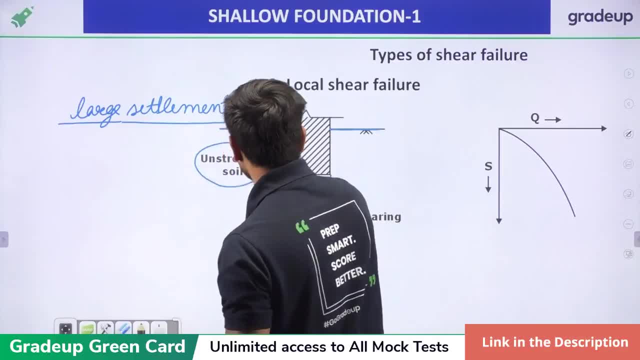 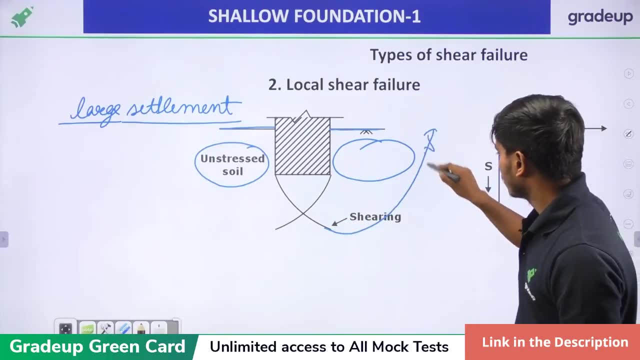 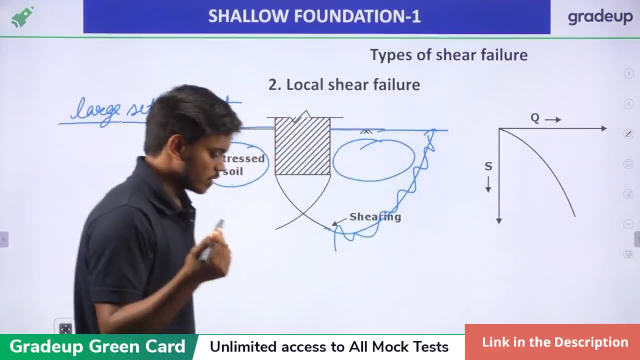 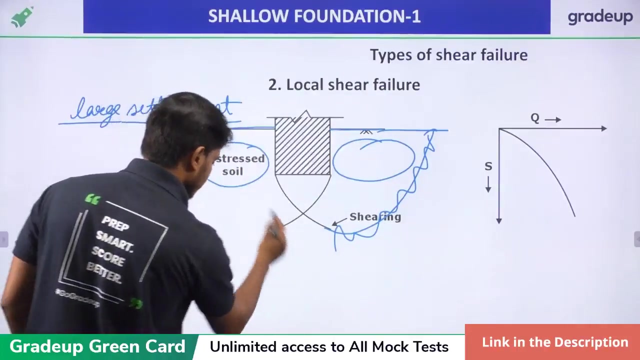 also you can see that the soil- here it is completely unstressed because it is the stress zone- is not coming, is not coming till ground level. okay, so this failure is basically progressive failure. okay, it is not a sudden failure like this. in previous case, failure was sudden after this particular value. sorry, 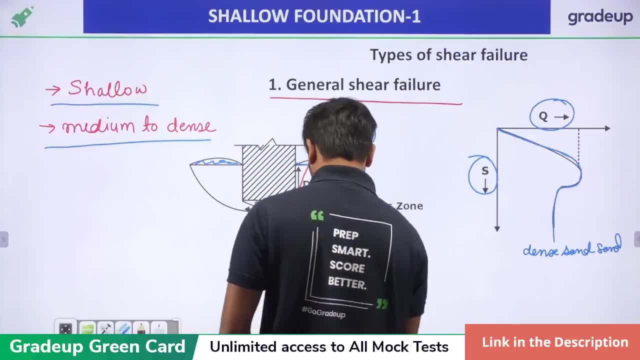 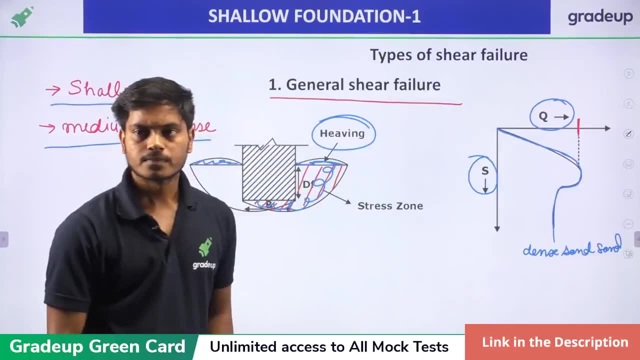 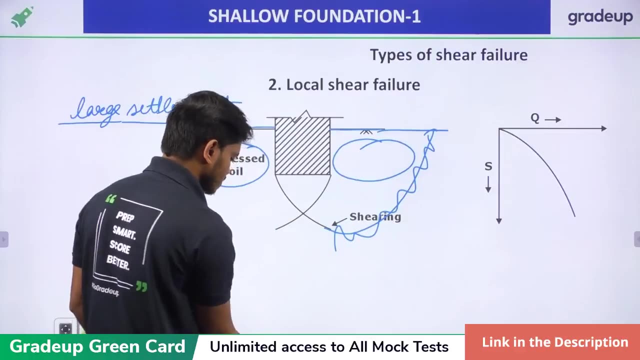 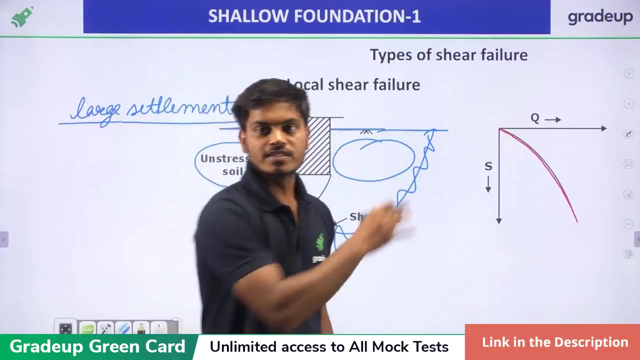 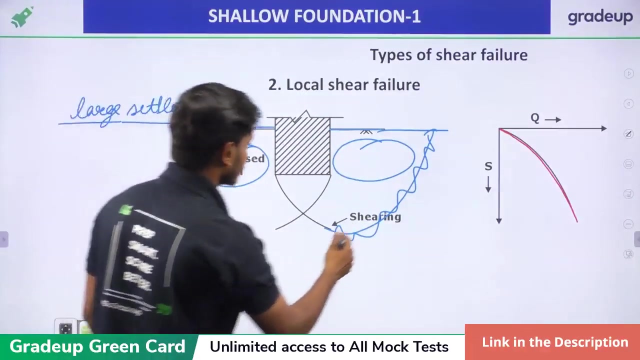 after this particular value of load, the settlement is sudden. okay, but in case of this failure, this shear failure, which is local shear failure, thus this failure is progressive, okay, so this is why we are making the graph perfect. so here, as you can see, this was all about local shear failure. last is your. 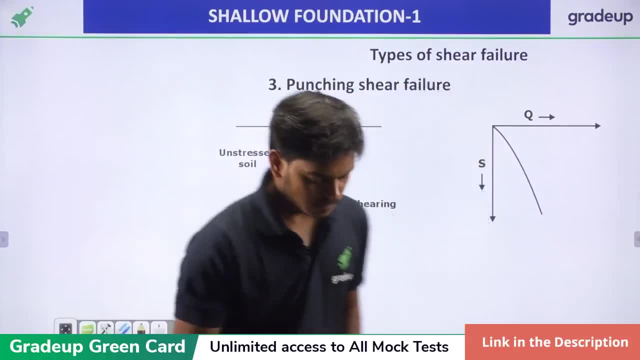 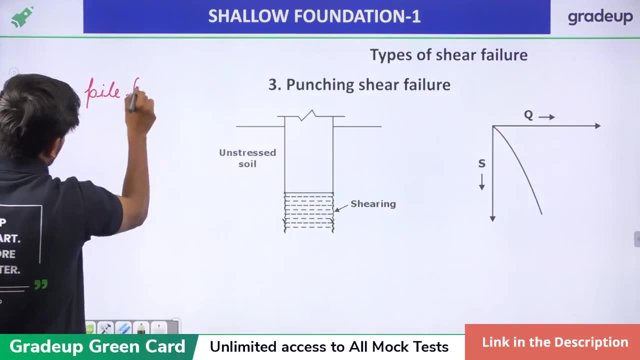 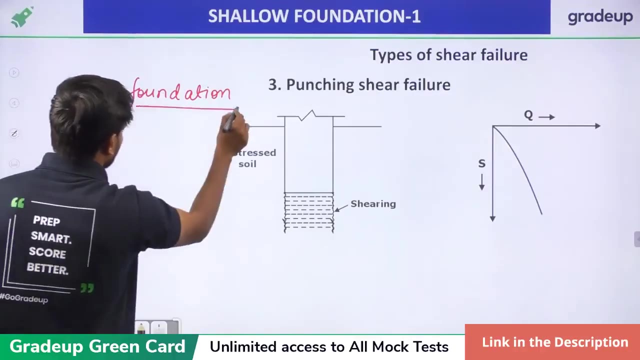 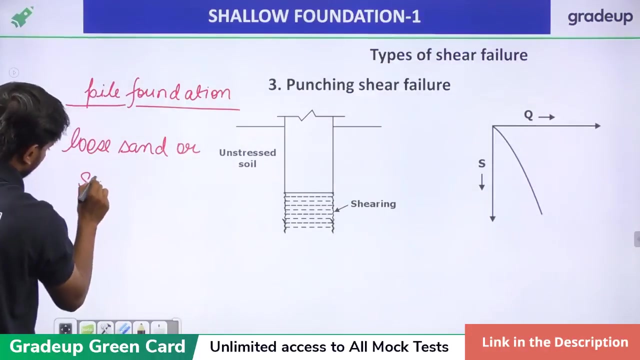 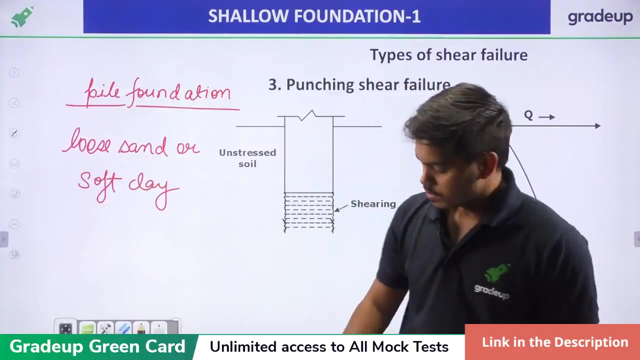 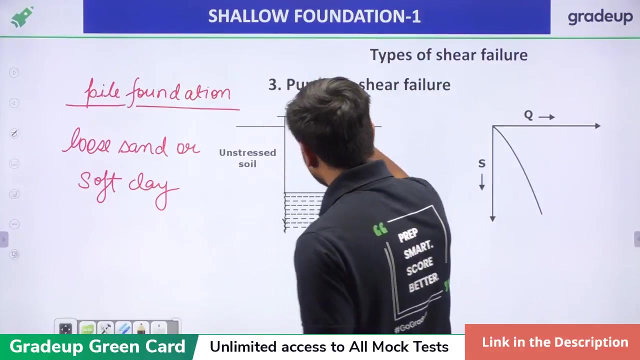 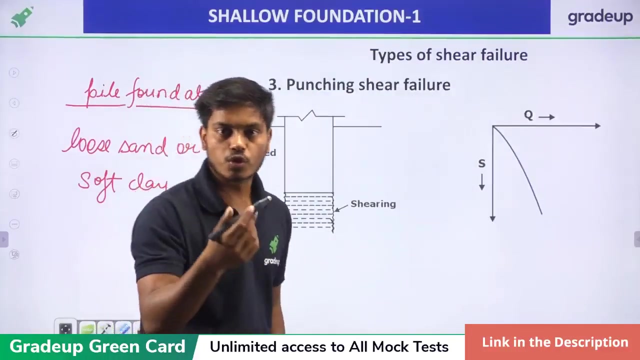 punching, shear failure. punching, shear failure. first thing is it happens in your pile, foundation, pile foundation, loose sand or soft clay, all right. so in this, what will happen is because of the excessive load, because of the excessive load, this particular pile all right will be the soil below this pile. the soil below this pile, it will just sheared by its. 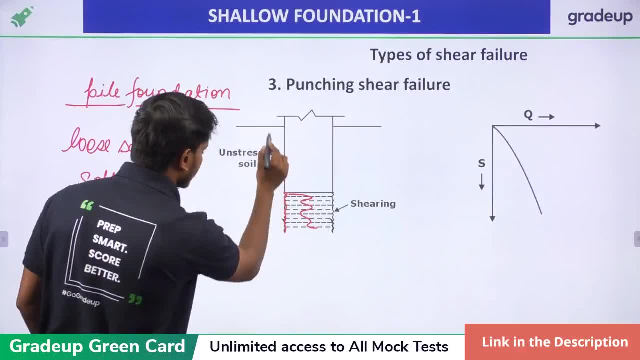 adjacent soil. so suppose this is the soil below this pile, it will just sheared by its adjacent soil. so suppose this is the soil below this pile, it will just sheared by its adjacent soil. so suppose this is the soil here. this is the adjacent soil right now. it won't. 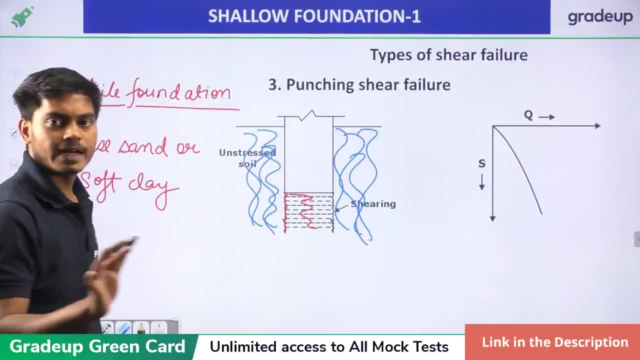 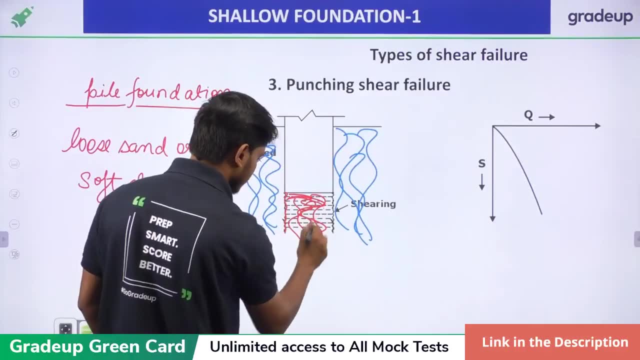 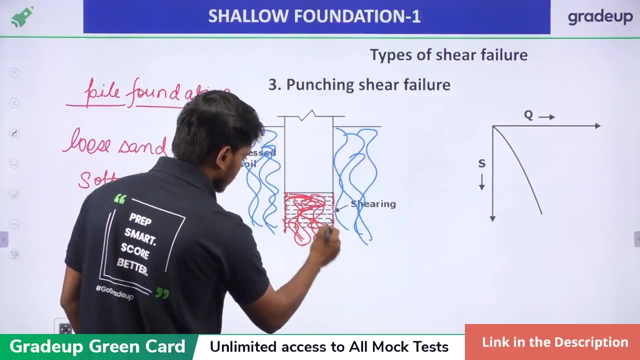 even affect. it won't give any affect to the adjacent soil, so it will be just punched by the lane. it's clear that it will be just punch. this is the soil which will be, will be, which will get affected. okay, and this right here. this phenomena is known as shearing, so you can say that the soil below the 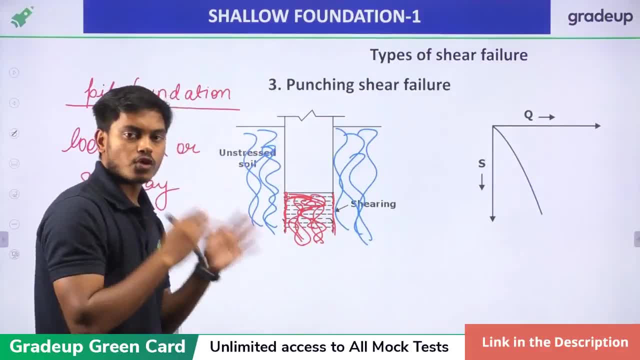 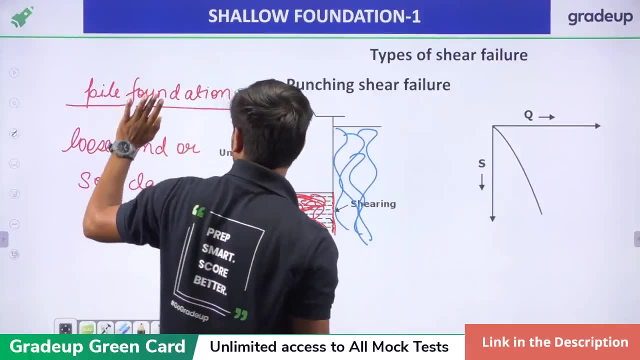 foundation pile. you can see this has become Butchering of 후� Rockyա�n foundation will cut. all right, it will cut from its adjacent soil. okay, this happens in your pile foundation or deep foundation and the type of sand or the type of soil is loose. 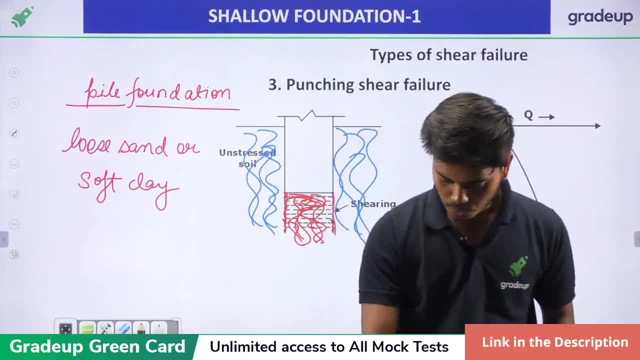 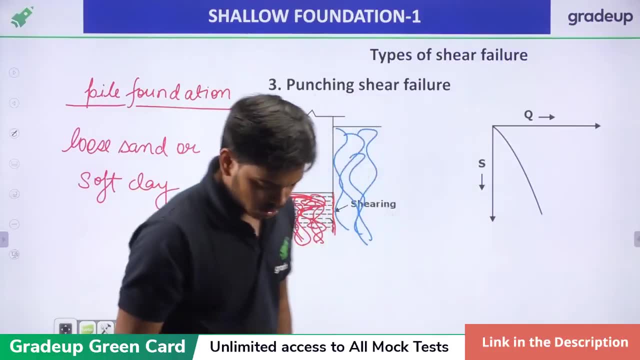 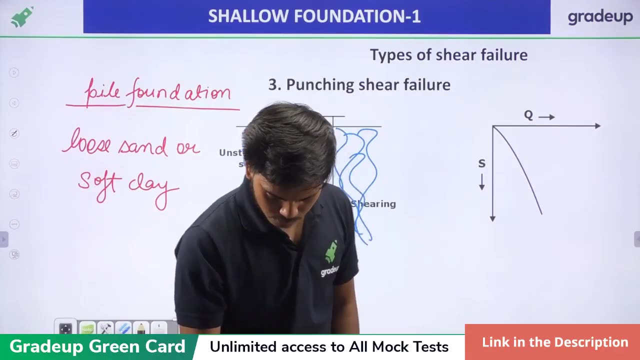 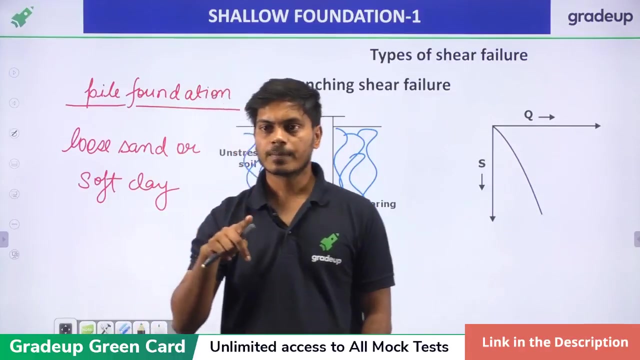 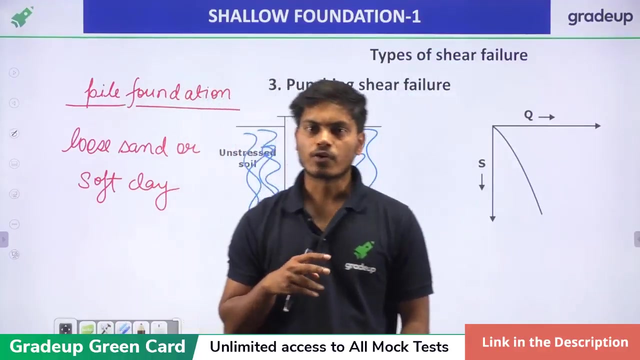 sand or soft clay, loose sand or soft clay, all right. So these were the type of failures. the type of these are the type of your shear failures. one was general shear failure. okay, in question it was. it will be given in the question, azar, that the foundation has failed in general, local or which failure in most of the question. 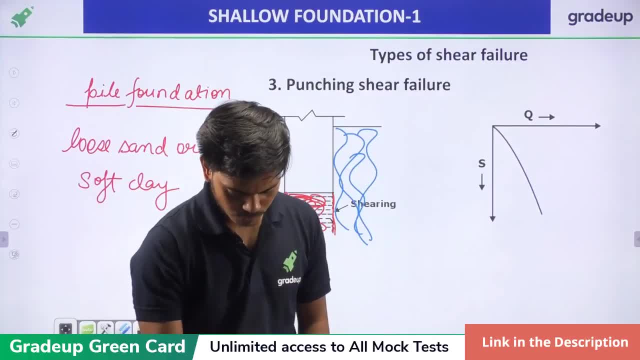 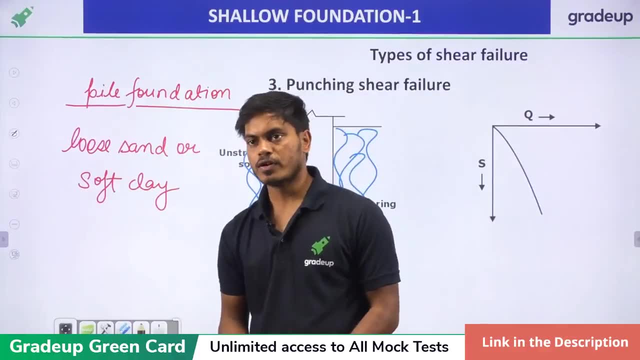 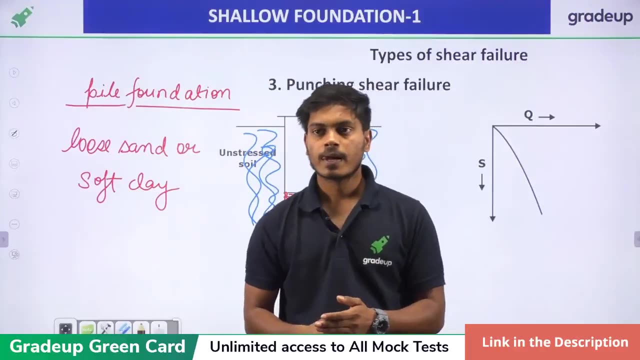 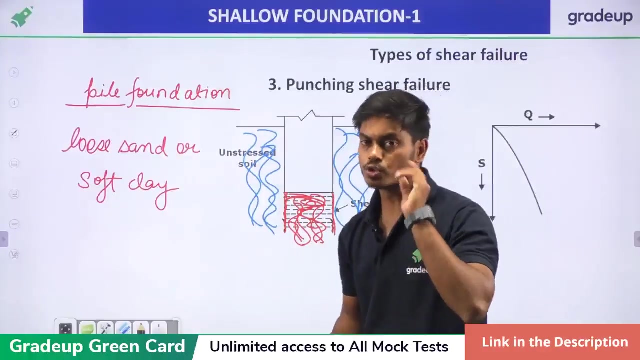 it will be given to us. all right, Okay, question: foundation is type of type of deep foundation? yes, Rakesh, okay, so these are the information that will be given in the question. all right, okay, and in case, in case, for one percent, it is not given in the question. so now you know the conditions when the shear 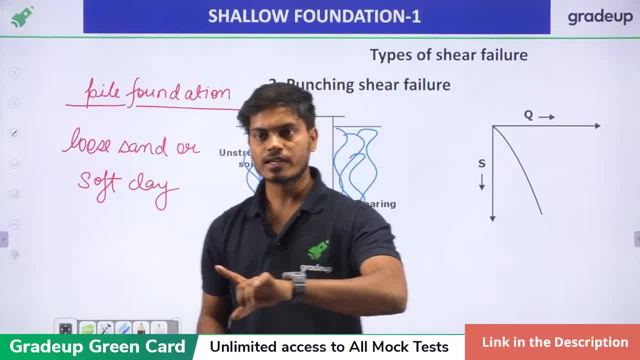 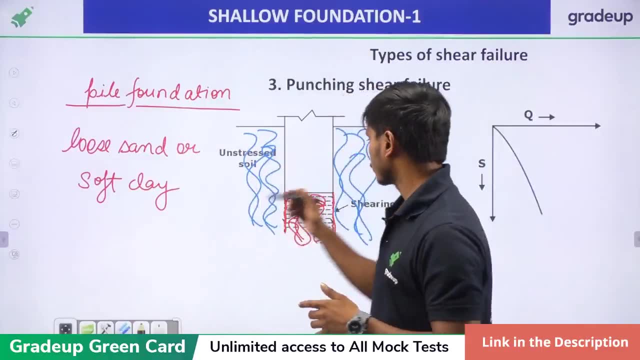 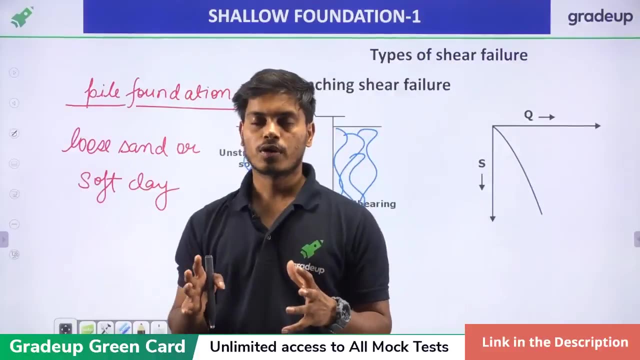 failure will occur. the general shear failure occur when the local shear failure occur and when the punching shear failure will occur. okay, How, like you know, The when the stress zone will come, like here also stress zone won't come all right on the ground level. so you know in which failure the- what do you call it? the stress zone will. 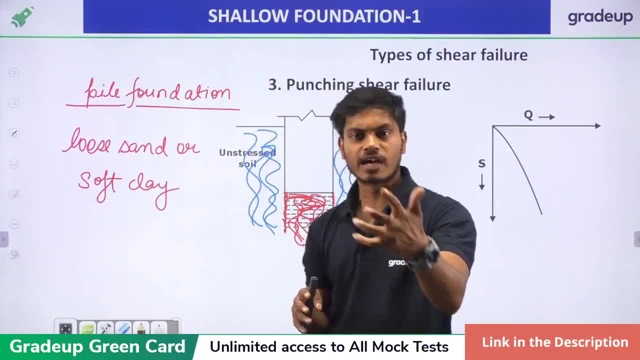 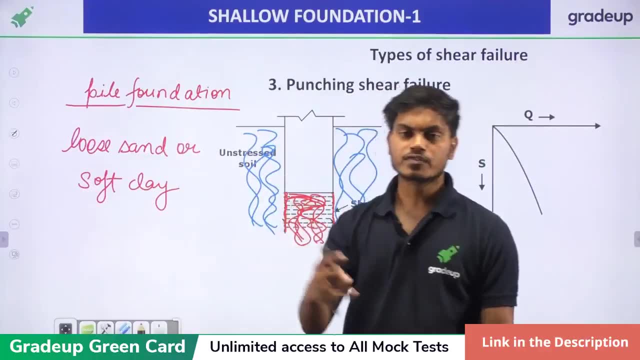 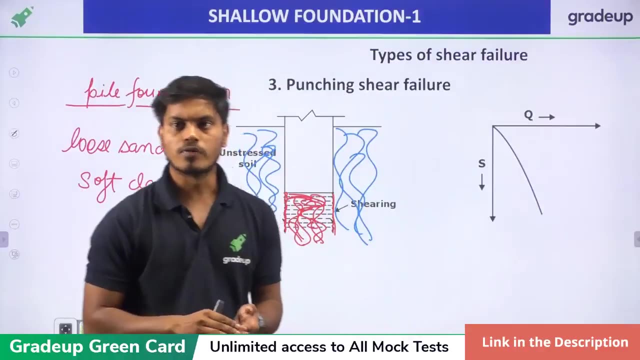 come up to ground level. also, you know which sand or which type of soil okay is like, which failure will occur in which type of soil okay and which foundation also. so by these information they will be given in the question, you will be able to solve it okay. 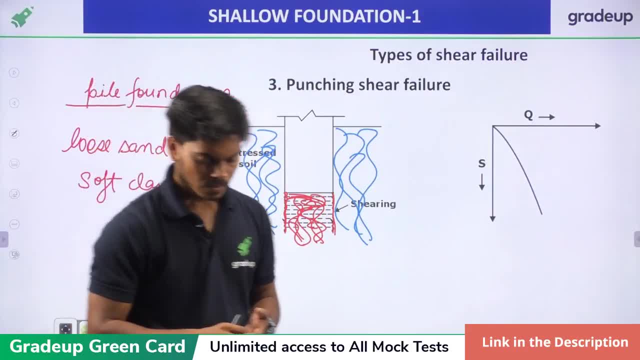 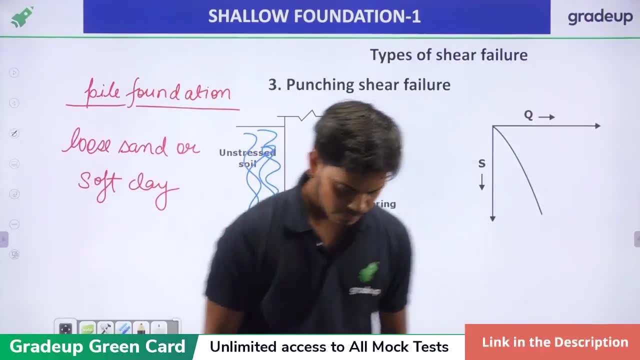 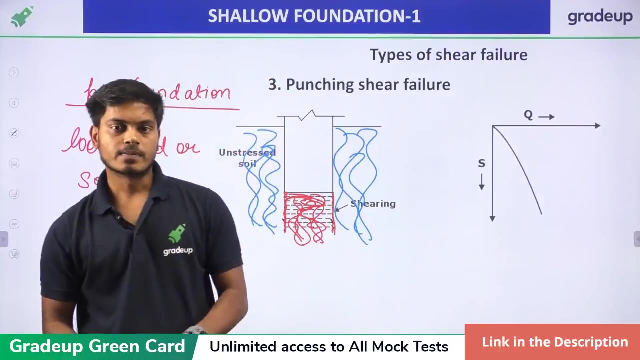 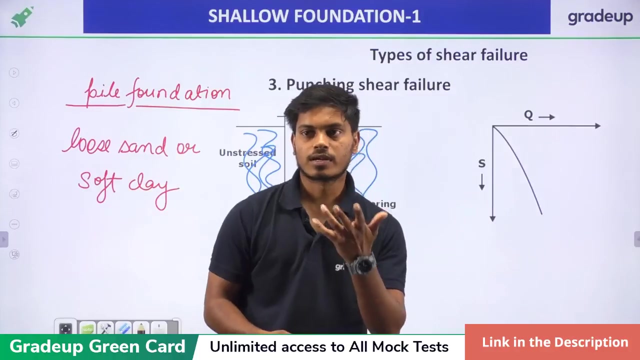 Abhishek. okay, so these are the things that we are going to discuss today? I think yes. after this, the thing that we are going to discuss is how to determine, how to determine the bearing capacity. there are various, various methods. okay, good evening, Sonal, you are late. 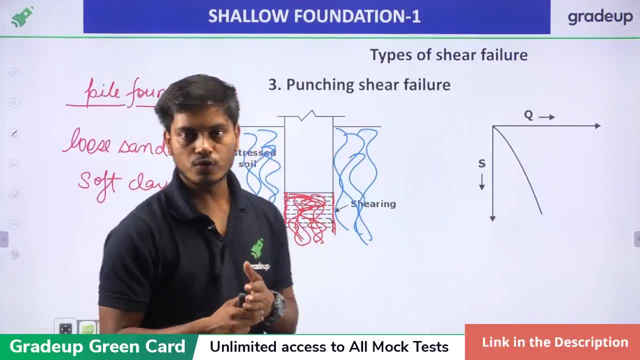 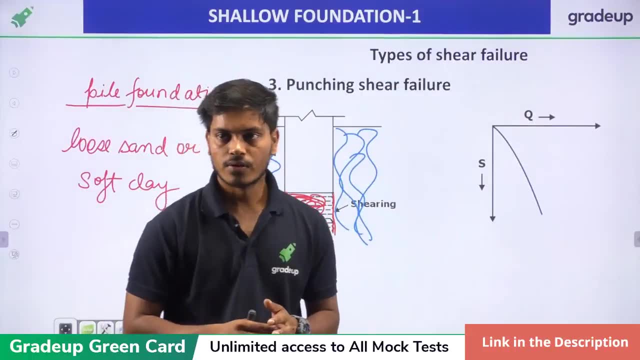 I think. but you can watch the video and any one of you who are going to watch the video later on, You can just ask anything what you have regarding the topic in the comment section. okay, I am replying each one of you. in case I am not able to reply any one of you, please let me. 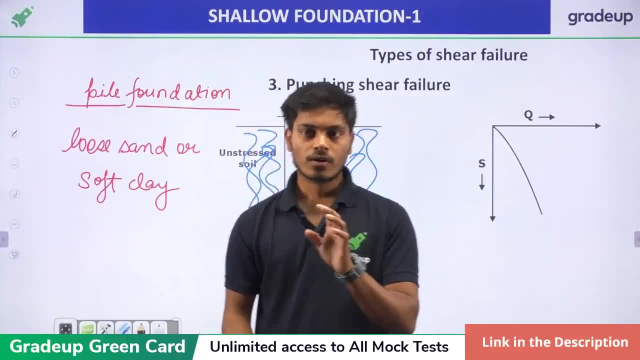 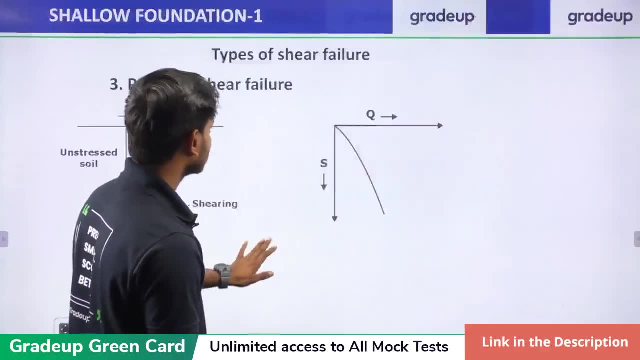 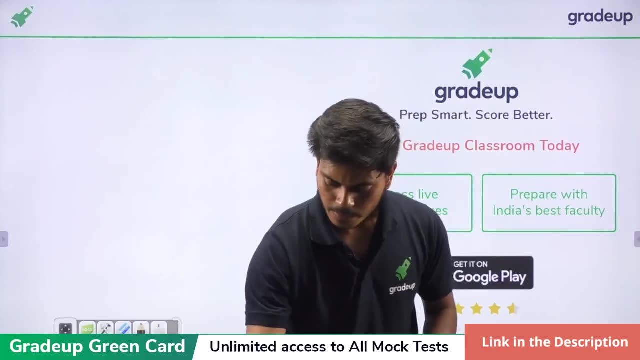 know. okay, it will happen only by by mistake. all right, there is no intention of mine of not replying anyone. till now I have replied each one of you, okay. so this was it. okay, this was it for today's session, for shallow foundation. In tomorrow's session we are going to discuss the tomorrow's session. timing will be 7: 15. 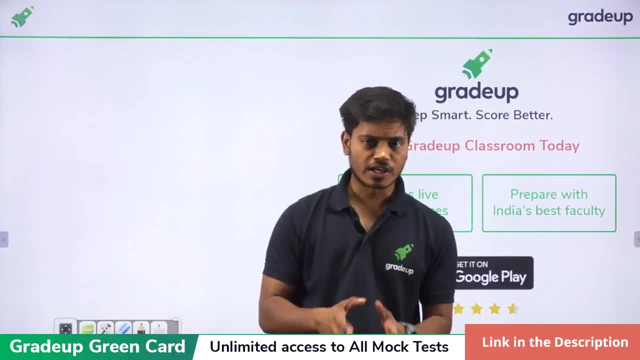 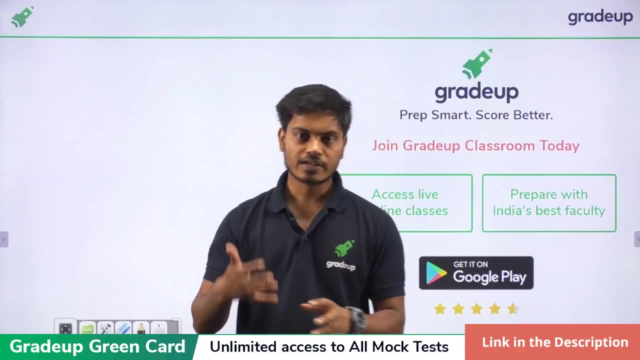 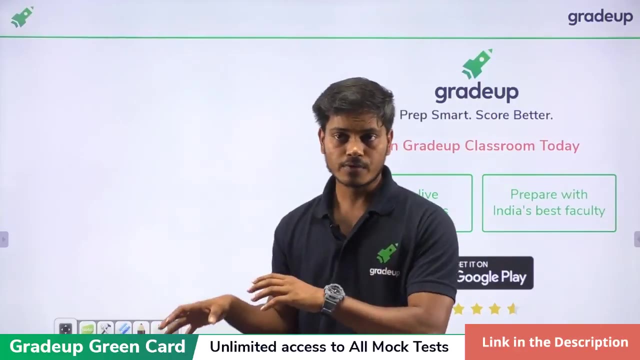 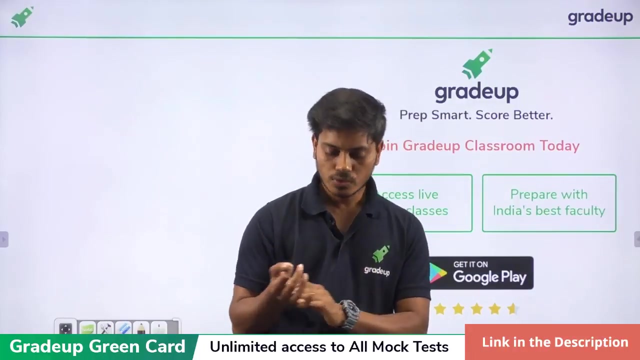 PM and we are going to discuss the shallow foundation, part 2, in that we will be talking about the method to determine the bearing capacity. all right, there are various methods. so, like, field method is also there, and there are some analytical method also, so both of them we are going to see tomorrow. all right, floating raft foundation. I have told you what. 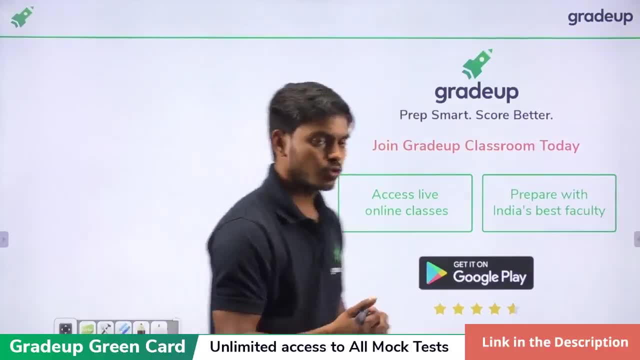 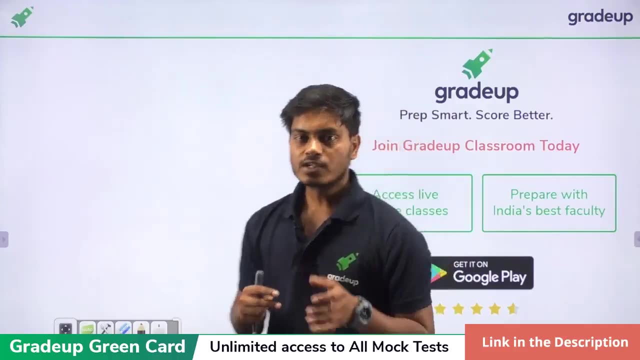 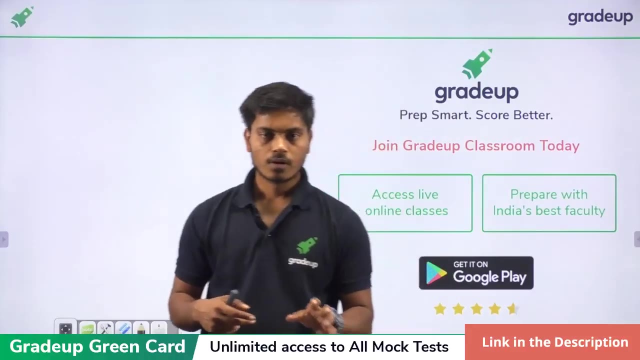 happens in that particular foundation is: we have to excavate the soil. excavation will be there. we have to excavate the soil. how much soil? the weight of that soil should be equal to the weight of the building and the weight of the foundation. all right, so now. 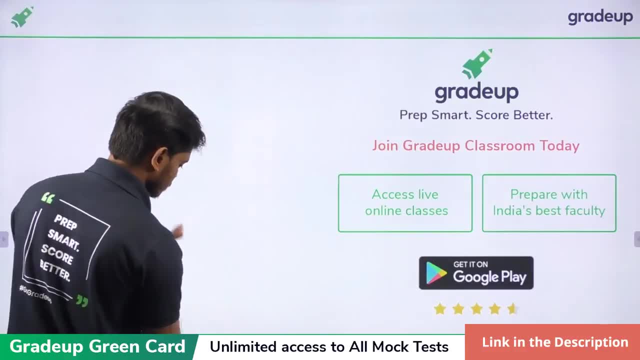 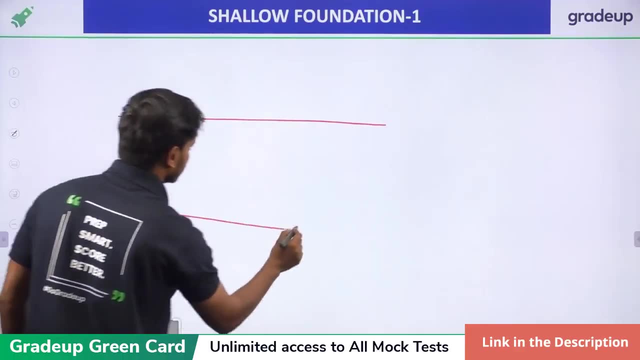 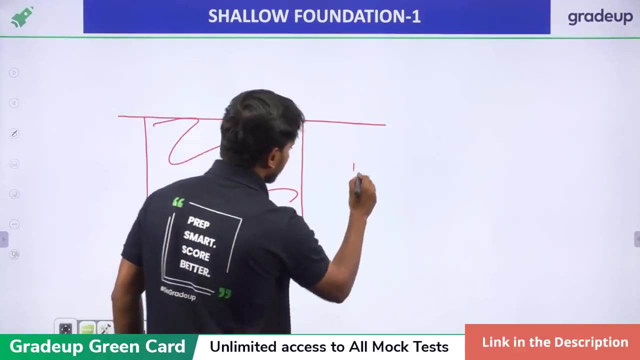 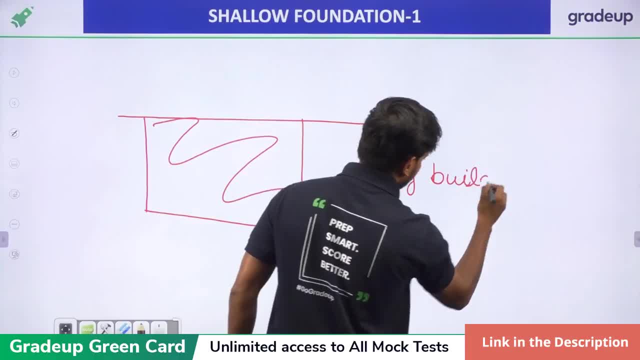 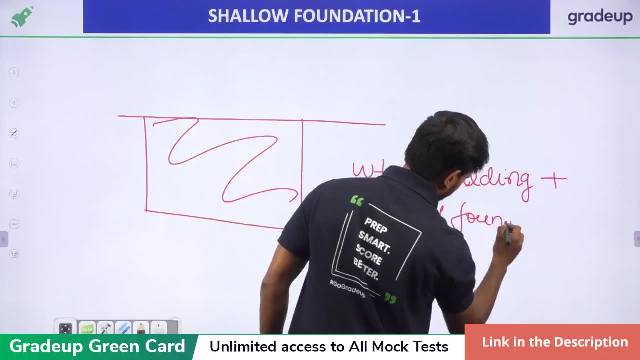 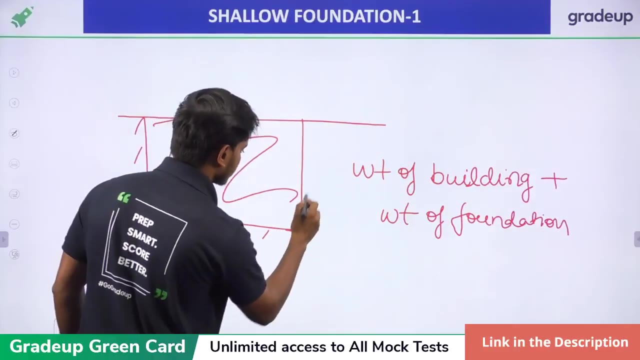 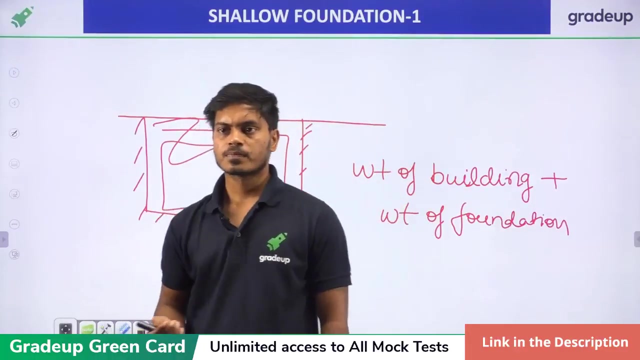 of building or structure, any structure, it could be, plus weight of foundation of that structure. all right, so now you will. you will have the extra space. like. this space is free for you. you can use it for any purpose: Parking and anything else. okay, excavated soil equals to weight of building plus weight. 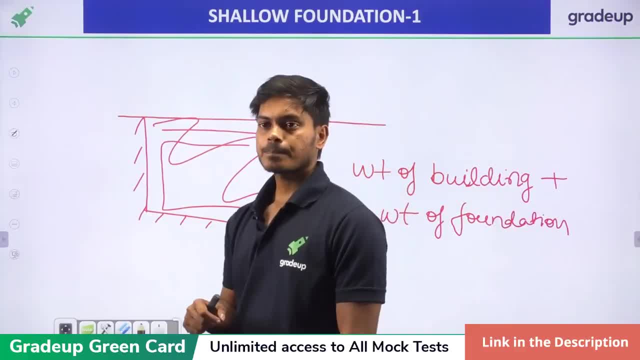 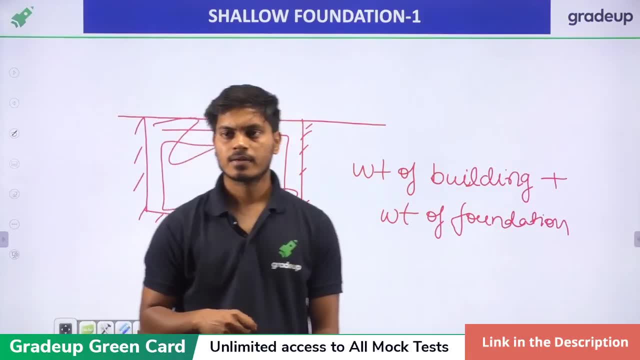 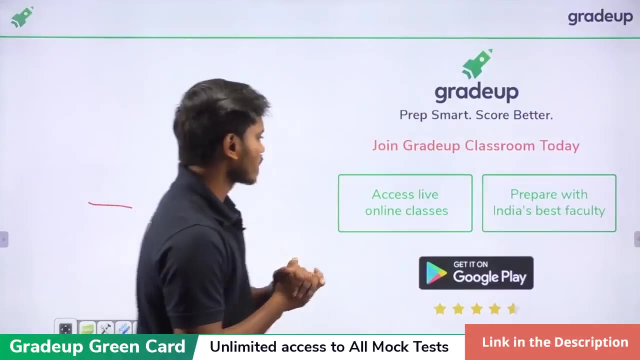 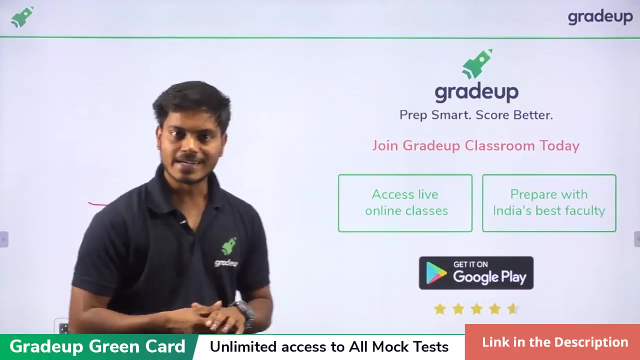 of foundation. yes, Kiran. good, yes, Arshad, it is enough, right, okay, all right. so his doubt: it is clear and if you have any doubt regarding anything and if you want me to answer your doubt, you can join the grade up app and also you can go and follow me on the grade up app.